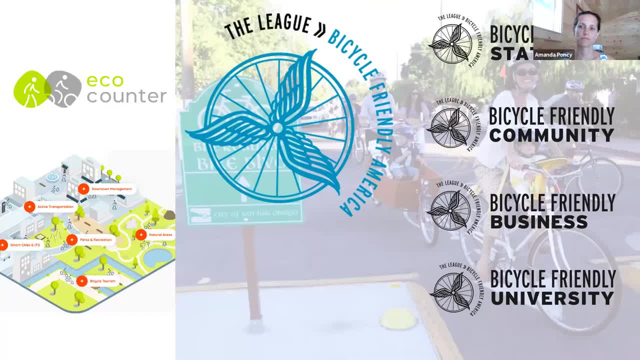 So I'm going to go ahead and start off with a little bit of an introduction to the topic itself, And we're excited to transition a little bit to how to use bike data. if you've been doing bike counts for a long time but don't quite know what to do with that data- to tell your story or to have 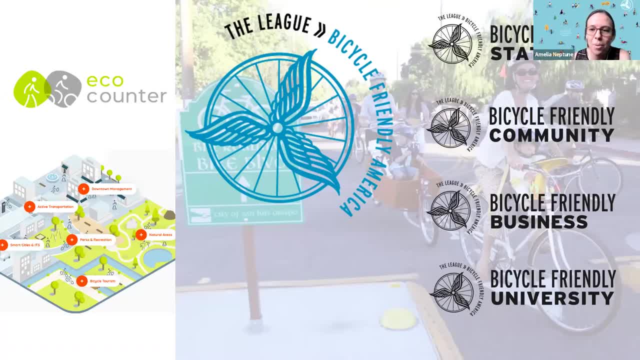 an impact in your community. So that's the goal of today's webinar, And I want to give a special shout out to Matt Ainsley at EcoCounter, who's a co-founder of the National Bike Summit. He's a on the call today, but not officially presenting. I hope he'll jump in and answer questions. 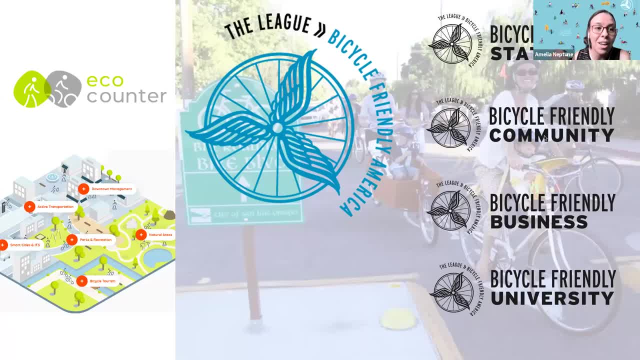 if needed. But Matt has done so much of the behind the scenes work for the competition that you'll hear about today, as well as the webinar itself today. So thank you, Matt, and thank you EcoCounter, for being such an awesome partner of the League. I also just want to give a little bit of background. 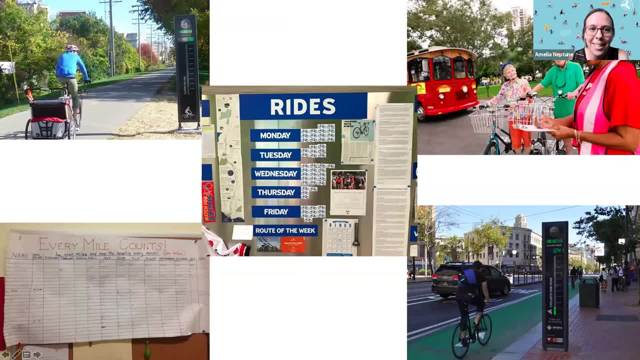 about why we care about data collection at the League of American Bicyclists and the Bicycle Friendly America program. Data collection is so important to so many partners. We all know that the bike data collection is one of the most important aspects of the Bicycle. 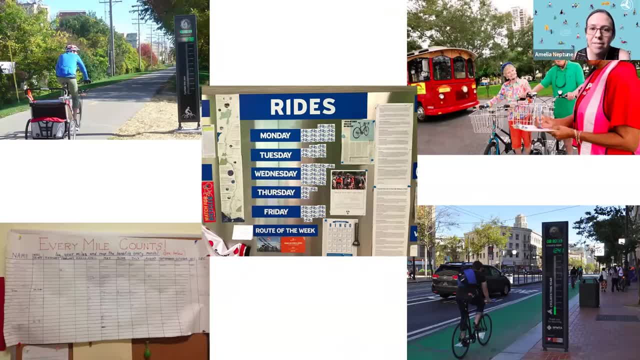 Friendly America program. So, whether you're a community, a business, a university, a state, quantitative and qualitative data are both so critical to making the case for improving bike infrastructure in your community, for increasing funding, for improving specific intersections in the entire network, overall equity related questions as an encouragement tool. There are so 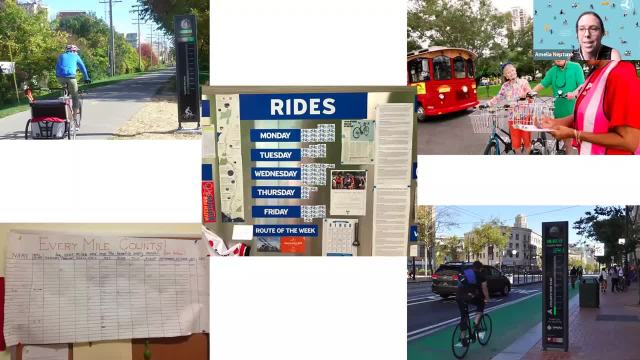 many reasons to do bike data collection and there are so many ways to do bike data collection, and that was one of the goals of the competition that you'll hear about today was bringing together different types of data collection. so, whether you're doing a gps, app based data collection, 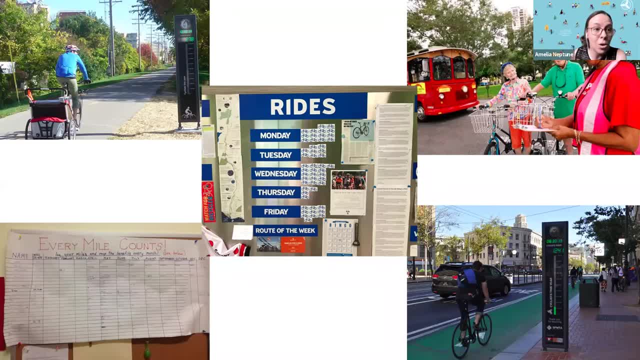 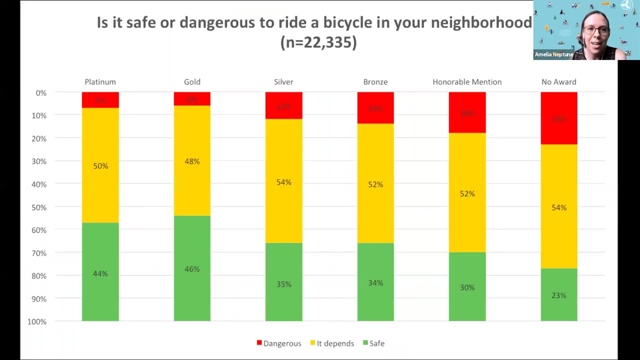 or manual counts or camera based collections or, if you have eco counter, automated counters. we hope that today's webinar is useful for you, regardless of the type of data you're collecting and the way that you're collecting it, and i mentioned qualitative data and i i want to 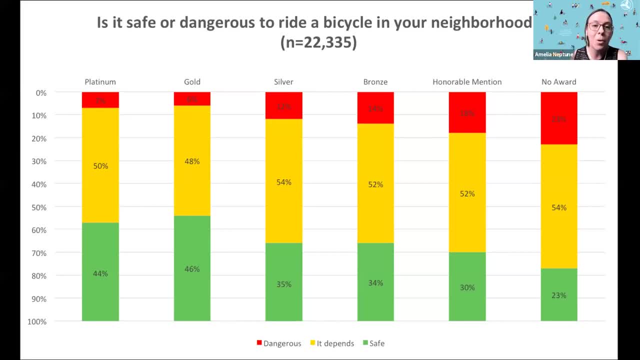 emphasize how important that is. today we're mostly talking about quantitative data and um for good reason, but i, you know, we do surveys as part of the bicycle friendly community program, and understanding the barriers that people feel, perceived barriers and perceptions of safety are so important when you're talking about bike infrastructure and creating a 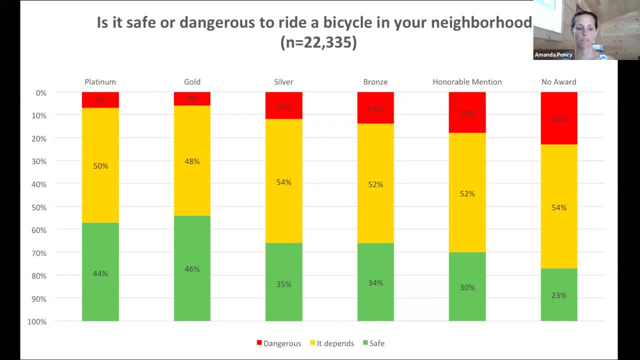 a safe bike network that's appealing and inviting to bicyclists of all ages, and about all ages, and if you're interested in learning more about bike infrastructure and So this is a snapshot of one of the questions we ask on the public BFC survey that we do whenever a community applies to the BFC program. 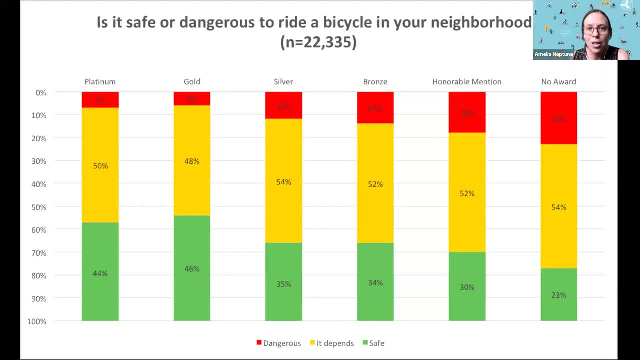 And we've been able to do some analysis over the years of how a question like this varies in different award level communities And, as you can see, even the platinum level communities have room to improve And our goal at the league is to help all communities improve, sort of meeting them where they are, regardless of where they started, where they are now, you know, climate size, geography, density, all of those factors. 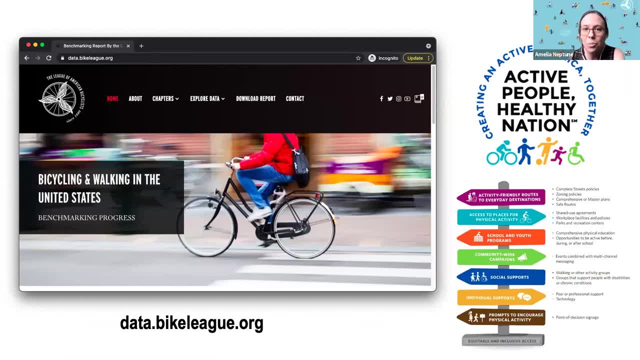 And then I also wanted to give a shout out to our relatively new website, databikeleagueorg. If you're on this webinar, you're probably very interested in bike data, so I wanted to make sure everyone is familiar with this. For years we have been partnering with the CDC through their academic 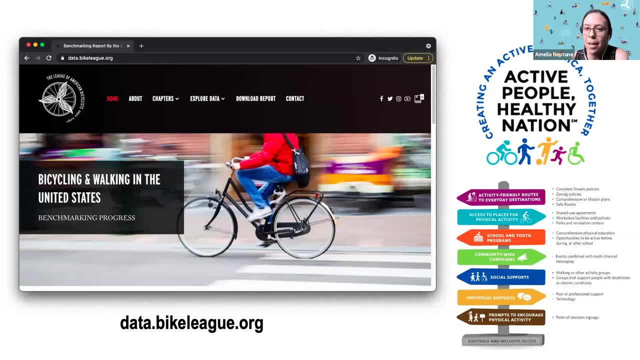 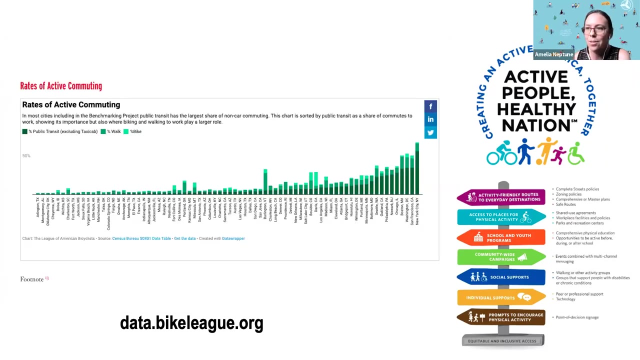 and active people. healthy nation initiative, which is an effort to help 27,- 27 million Americans become more physically active by 2027.. And the bicycle friendly community program and the benchmarking website, which used to be a printed report that came out every two years, is- it's now- a website with tons of great data about every state, all the largest cities in the country and some great graphs. 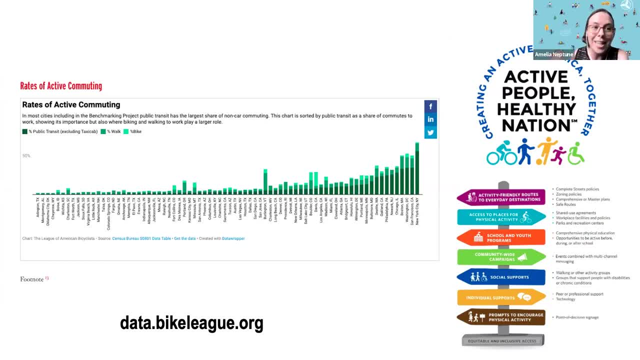 like like the one you see here, as well as spreadsheets that you can download of data To do analysis yourself. so if you're a researcher or you're just interested in bike data and you want to compare your community to other places, 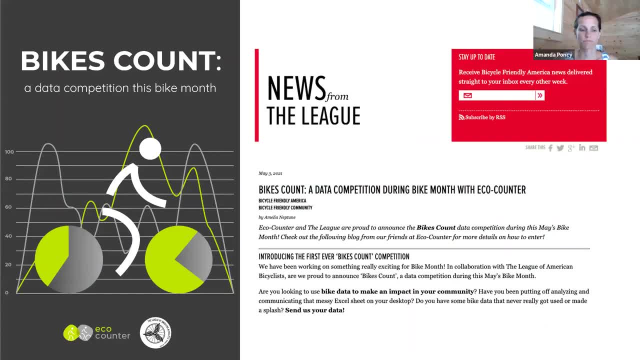 I encourage you to check out databikeleagueorg. So now getting to the competition. During bike month, the league and eco counter co hosted this bike data competition, where we invited communities, businesses, universities who are participants in the BFA program and advocacy organizations to apply for this competition. 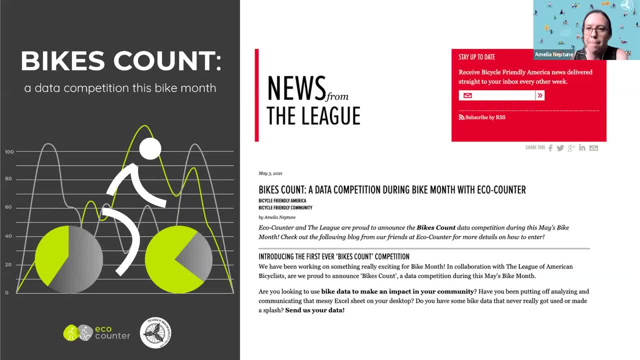 They had to fill out an application and describe their account program, the challenges they faced, their goals, including their equity related goals, And they had to submit their actual data. So we received dozens of spreadsheets of bike count data from all over the country. 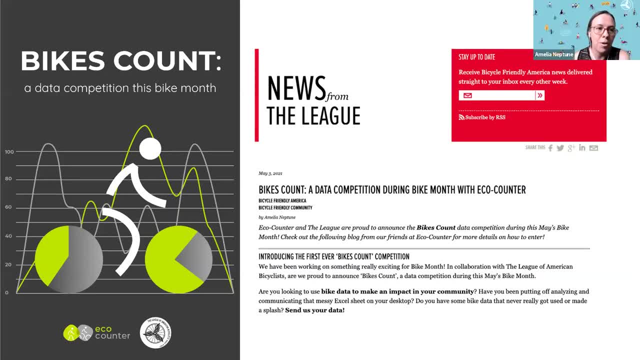 We received a number of really interesting submissions with everything from bike share data to manual accounts, to spreadsheets and maps that were produced from time lapse videos of GoPro footage. We received a number of really interesting submissions with everything from bike share data to manual counts, to spreadsheets and maps that were produced from time lapse videos of GoPro footage. 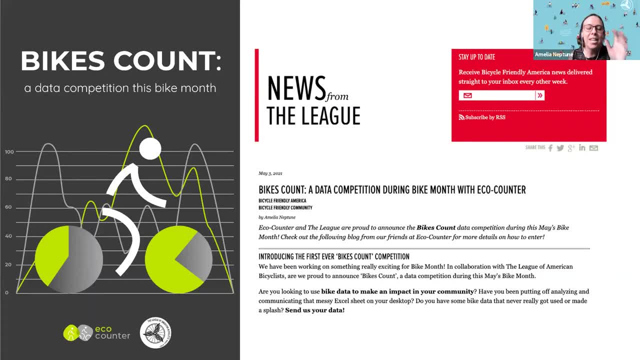 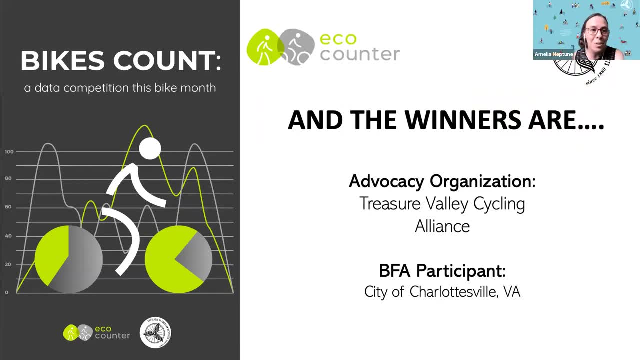 And it was really fun to review those submissions and to hear about the common challenges that so many communities and advocacy groups face. And we're excited to announce the winners who are presenting on today's webinar: Treasure Valley cycling Alliance, one in the advocacy organization category, and the city of Charlottesville, Virginia, one in the BFA participant category. 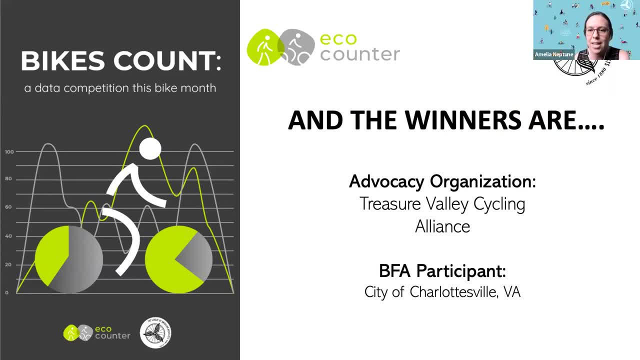 And in both of these places there is a long history of data collection challenge, of what to do with that data. So I'm excited for you to hear more about how those programs were started, how they developed, what challenges they faced and then what EcoCounter. 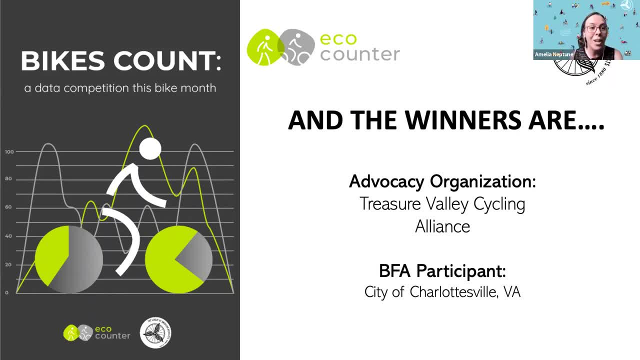 was able to do with their data, Because part of winning this competition was getting analysis and assistance with storytelling and data visualization using their, you know, decades worth of bite count data. So Mike and Amanda from those two places are going to be presenting on what they learned, what their challenges are and we hope those lessons. 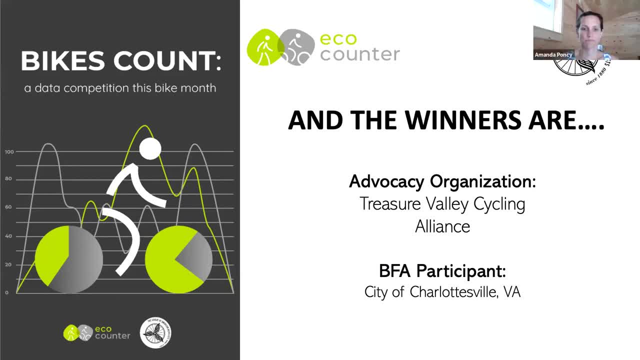 learned are applicable and valuable to everyone on the call. I also really briefly want to give a shout out to our honorable mentions, our runners up in the competition in the advocacy organization category- Walk, Bike, Tampa- and in the BFA participant category, the City of Columbia. 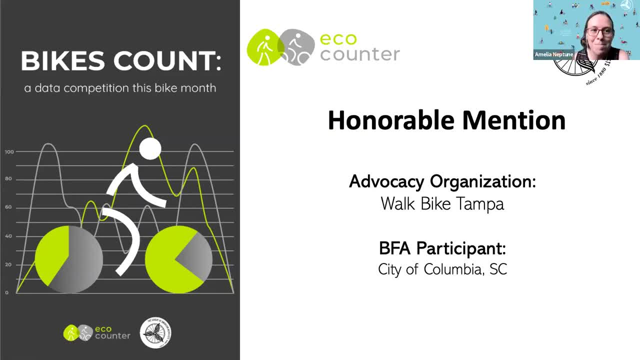 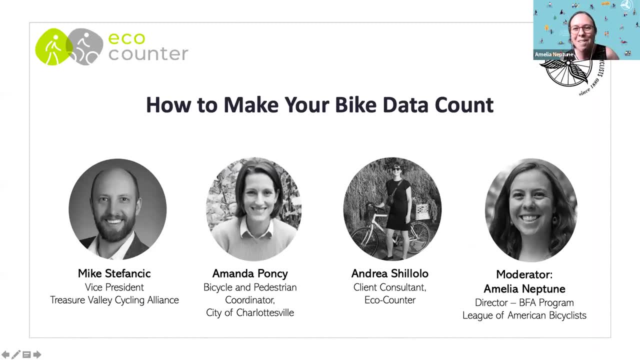 South Carolina, And both of those had really great submissions as well, and we just wanted to give a nod to them. So with that, that's enough for me. We're going to hear from our speakers now, and I'll introduce each of them right before they talk. 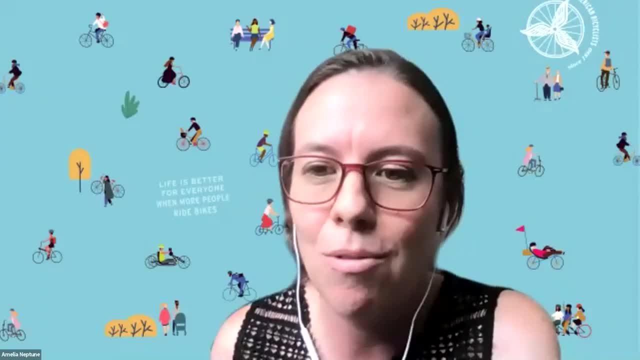 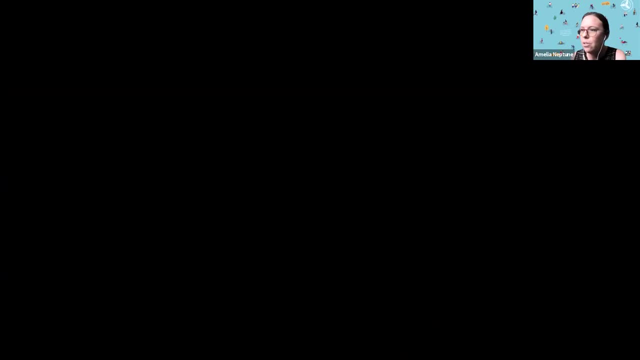 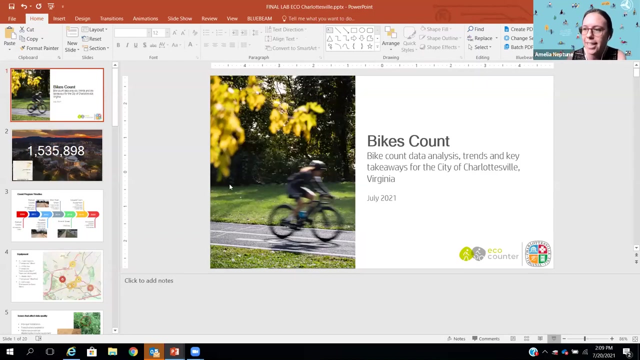 So I will stop sharing my screen, and first I'll be handing it over to Amanda, And so, Amanda, feel free to get your screen up and running, And while you do that, I will introduce you. So Amanda Poncey has served as the bicycle and pedestrian coordinator for the City of Charlottesville for nearly 10 years. 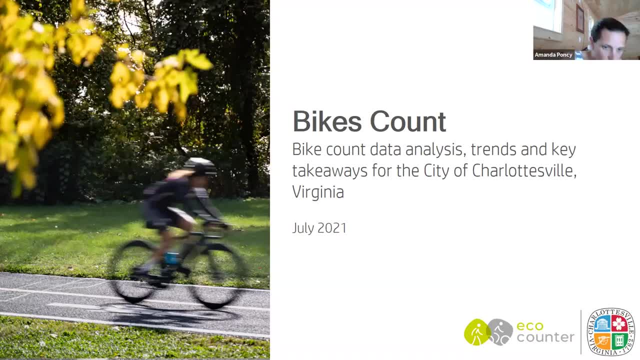 where she continues to pursue her interests: creating vibrant and healthy communities through sustainable transportation, and planning And community design. She is an adjunct faculty member at the University of Virginia's Urban and Environmental Planning Program and serves on the board of Smart Seville, a citizen-driven organization that promotes the use of technology to make cities better places to live. So thanks for being here, Amanda, and take it away. 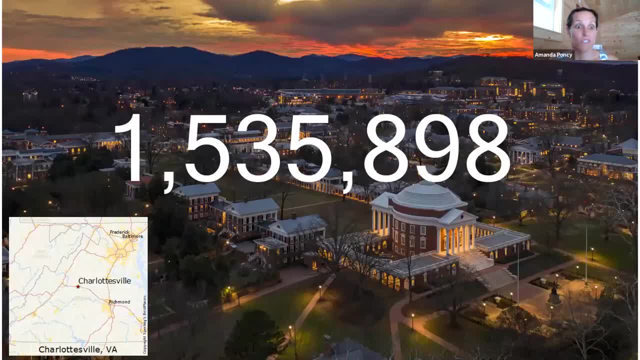 Hi, thank you. So 1.5 million people. Can you believe that in a city of 1.5 million people, Can you believe that in a city of only 10 square miles and 50,000 residents, that we'd be able to count 1.5 million people? 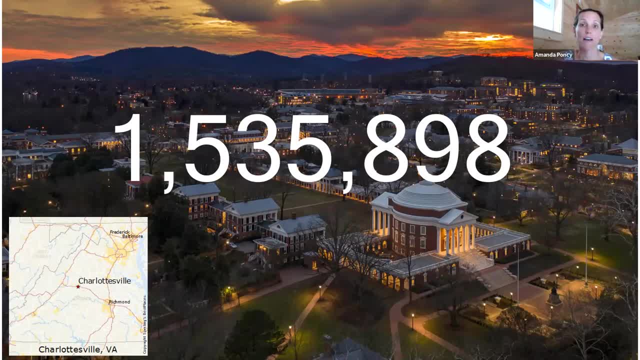 This number is really staggering to me, especially when you consider the fact that this doesn't even include our two high pedestrian activity destinations: the University of Virginia and our city's downtown mall. So what does this number mean and how do we communicate this data? 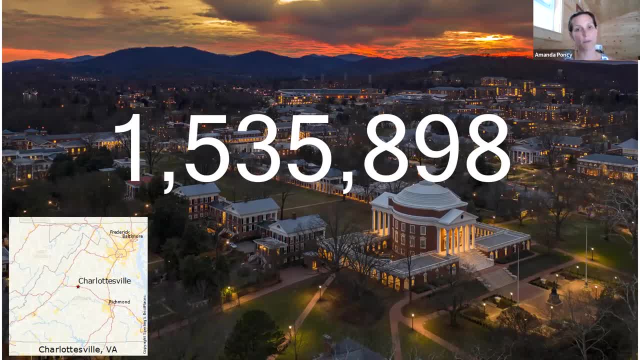 to support investments in walking and biking? That's the question that I wanted to answer with this. Bikes Count, data competition. My name is Amanda Ponce and I've been the bicycle and pedestrian coordinator with the city of Charlottesville for almost 10 years. We've been 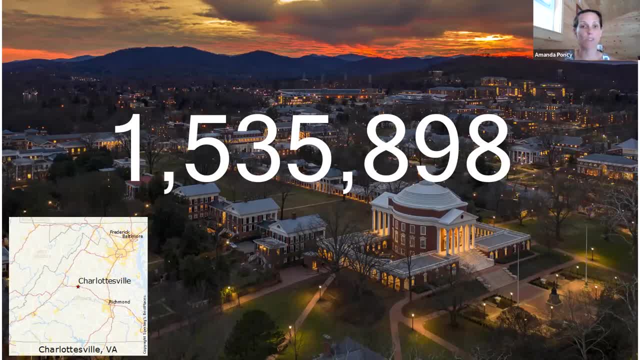 working with EcoCounter for the last six years and have really only scratched the surface with our data analysis. I'm a planner, not a techie or an analyst, and so I've really relied on the built-in reports that the EcoVisio software provides, And so I was really, really, really. excited that we were selected for this award so we could get professional health care workers to participate in this data competition, And so I was really, really, really excited that we were selected for this award so we could get professional health care workers to participate in this data competition, And so I was really, really, really excited. 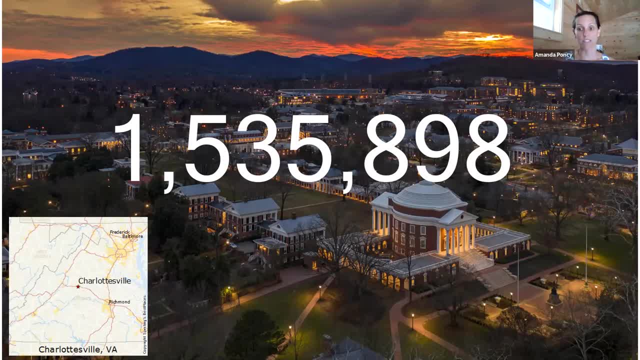 to help cleaning our data and dig deeper into what some of this data is telling us. to help cleaning our data and dig deeper into what some of this data is telling us. So, before we begin, I'd just like to orient the audience a little bit. I'm sure many of you have. 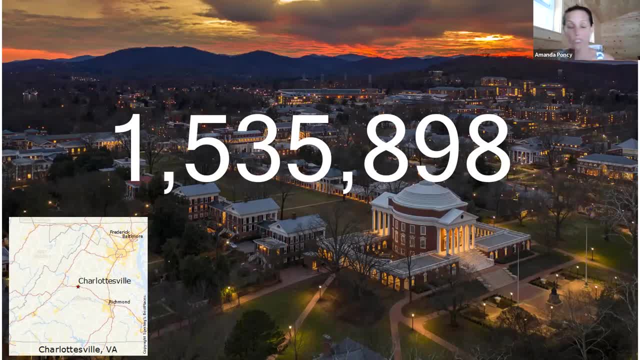 seen some pretty ugly pictures of Charlottesville over the last few years, but we're really a beautiful place. We're located in central Virginia, in the foothills of the Blue Ridge Mountains, about 100 miles southwest of Washington DC and 70 miles northwest of Richmond Virginia. 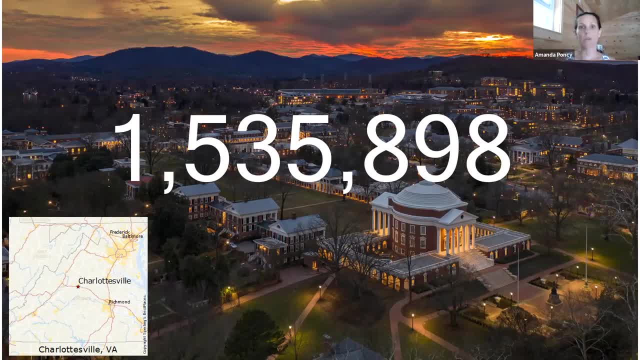 We're a college town, home to the University of Virginia. We have a very silly topography: hot and humid summers as well as pretty decently cold winters and occasional snow. But despite all those challenges, 25 percent of our population commutes either by biking. 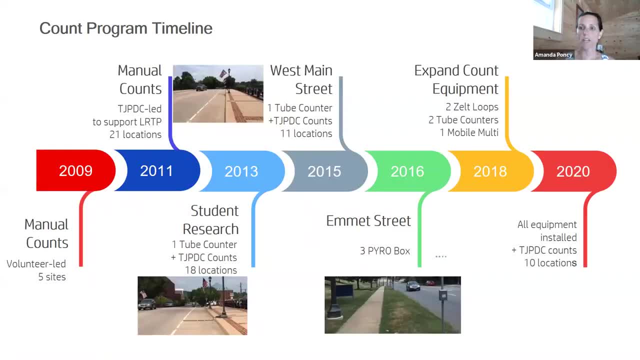 walking or transit. So I wanted to share just a little bit about our count program and how it has evolved over the years, starting with some volunteer-led count efforts into 2009.. Two years later, the Regional Planning District Commission took over that program to. 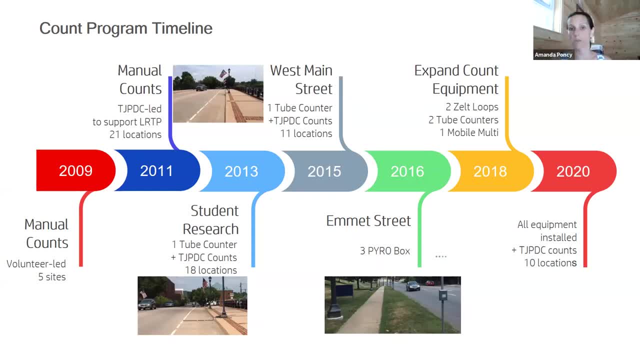 support the region's long-range transportation plan effort And for the most part, those have been continuing every two years since then. Our experience with EcoCounter started in 2013 when a PhD student- actually at UVA- purchased a tube counter for a research project about. 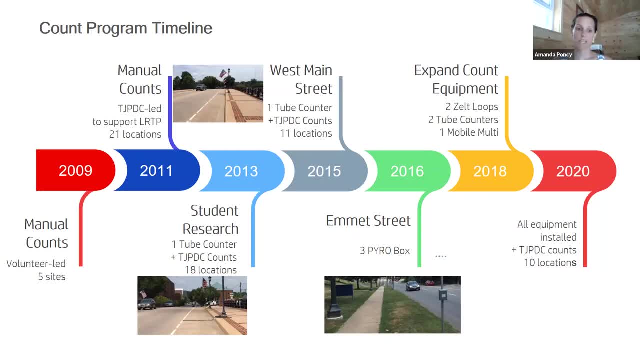 bicycle and bicycle travel demand. Both the city and the PDC were interested in that research and from there our plans to start an automated count program started to take shape. Unfortunately, due to the length of time it took for us to navigate the procurement process and some staffing changes at the PDC, the city became the owner. 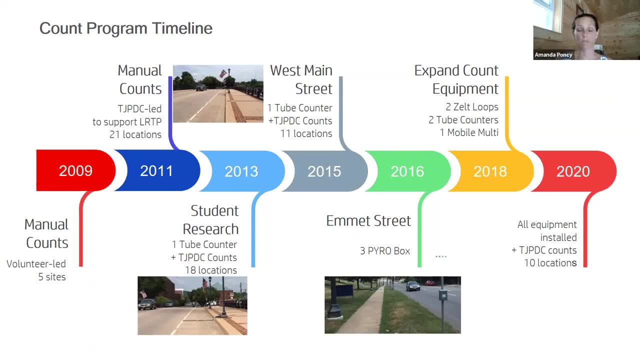 of the new equipment. Our intention originally was that the PDC would be the home to all of the data for the region, but we took this over In 2015,. we put our first two tube counters on the West Main Street corridor. This was a really important 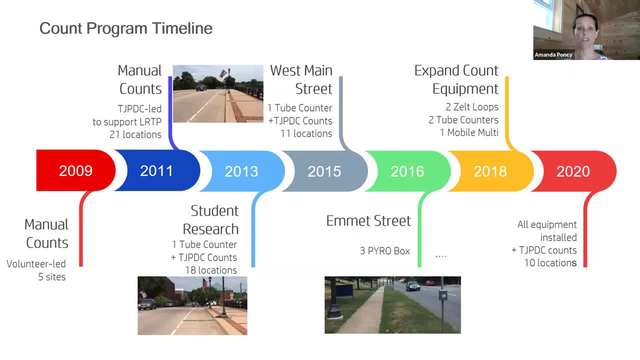 step for us because we had just completed a very contentious two-year planning study for the corridor and we wanted some good data to support project implementation. We expanded our equipment two other times, both in 2016 and 2018, with the help of our Bicycle and Pedestrian Advisory Committee. 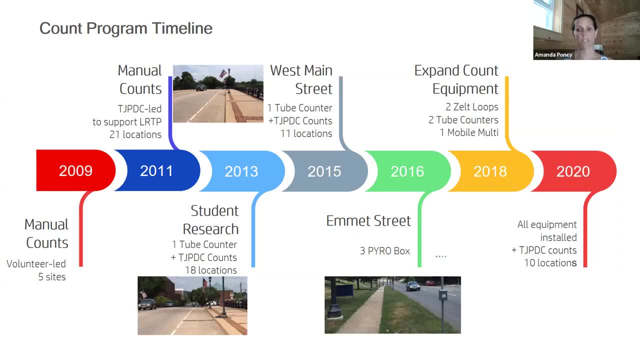 and with the hope of collecting before and after data for some of these projects that were under development. All but one of our counters were installed in 2019 and have been counting continuously ever since, and our last counter was installed in October of 2020.. That was a permanent. 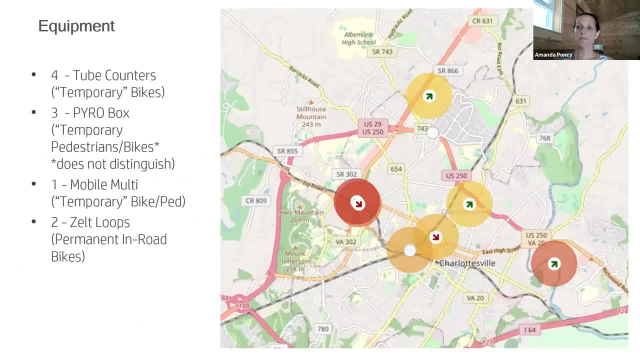 ZELT counter. This is a map showing the location of our equipment and some of the details of the type of equipment that we have. We have 10 total counters with a mix of both temporary and permanent counters. Some of them count bikes only. The rest count both bikes and pedestrians, but only. 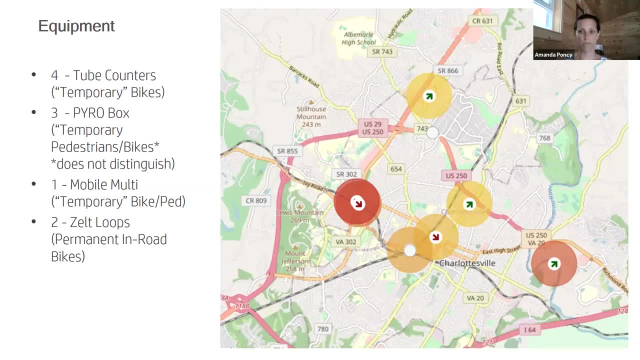 one of those distinguishes between the modes, and that's the mobile multi. They're installed on both shared use paths as well as on-street facilities, and two of our counters automatically send data to a cloud daily. The rest require that I visit the site and manually download the data. 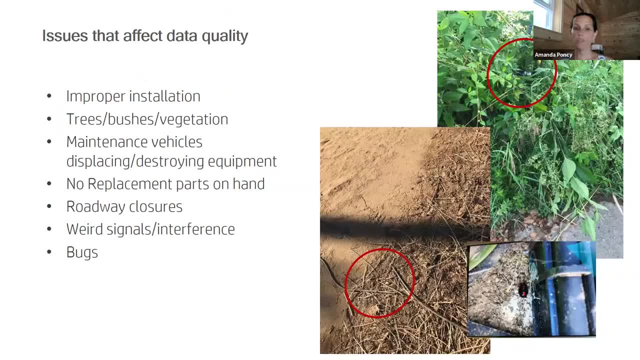 periodically. So one of the reasons why this competition was of interest was because we had some gaps and data inconsistencies that we wanted some help with cleaning. Some of the reasons for these inconsistencies include instances where the tubes weren't installed properly. If you don't have enough tension on the tube, the devices won't count. 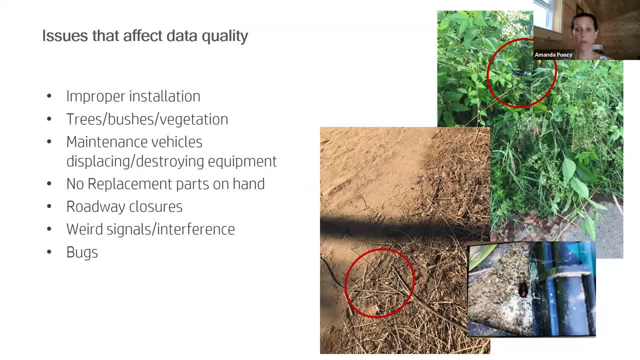 properly. We also had situations like in the back where our pyro sensors were counting vegetation and not necessarily people walking by. We've also had lawn mowers and snow plows and street sweepers damage our equipment. You can see a picture there on the bottom left. 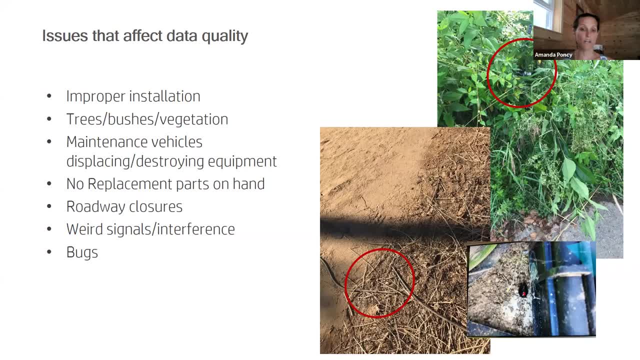 And you know that has led to some instances where we have gaps in our data because we didn't have a replacement part to be able to, to be able to address those damaged, damaged equipment easily. We've had some roadway closures. you know signs are placed in the bike. 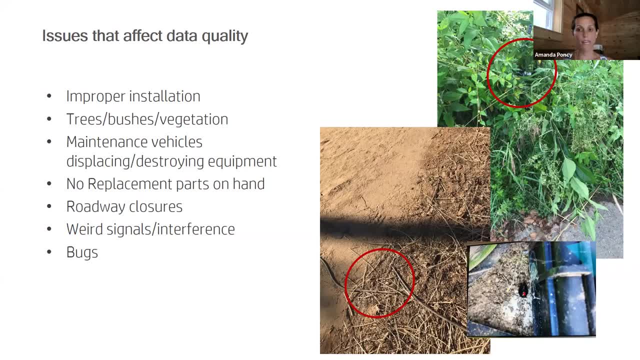 lane where our counters are located, and so we don't get accurate data that way. And most recently, we had to contend with some ants that created a home in the holes of our the sensor holes. I wish I could have shared a picture of that, but instead opted to share this picture. 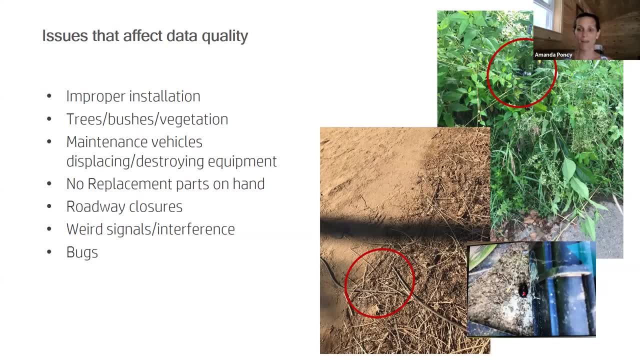 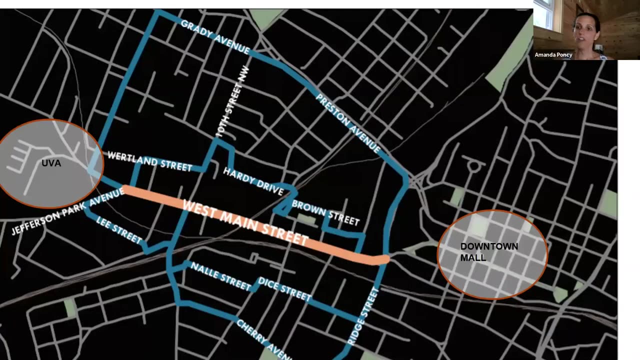 of a black widow spider that greeted me one October morning last year. You know we haven't had issues with spiders in our equipment or affecting the data quality, but I know that's something that some other people have had issues with. So I mentioned that our journey began with 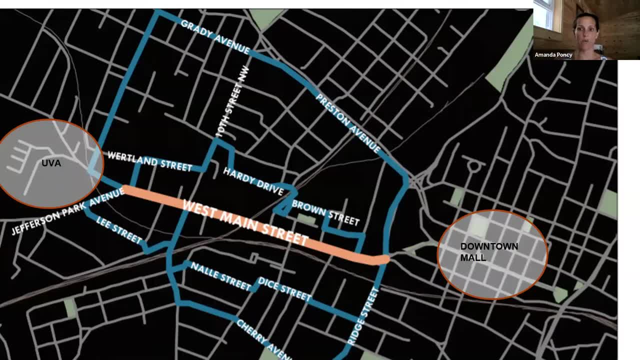 EcoCounter as a result of this West Main Street planning effort, and I wanted to share a few of the insights that we uncovered using EcoVisio's built-in reports. West Main Street is an emerging mixed-use corridor and has seen significant redevelopment in recent years. You can see: 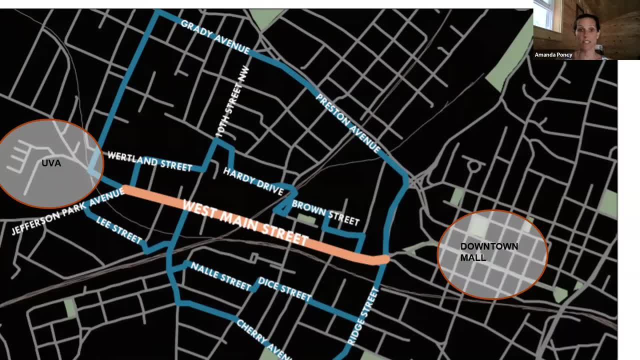 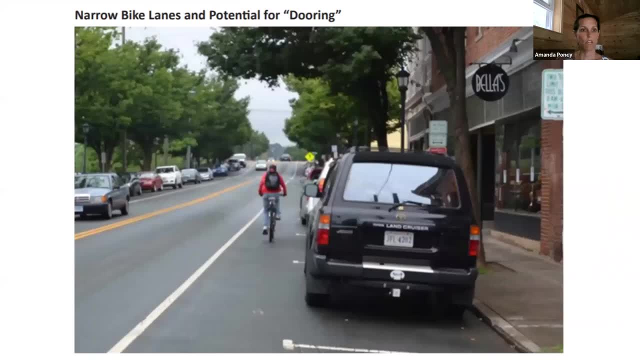 it provides a vital link between two of the cities and you know, in fact, the Commonwealth's important destinations, both the University of Virginia and the Downtown Mall. The existing conditions for bicyclists on the corridor are pretty terrible, as you can. 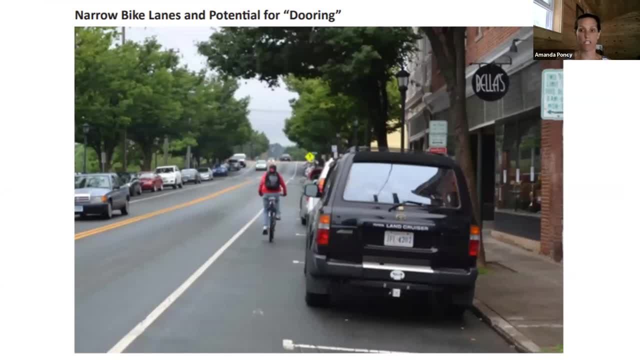 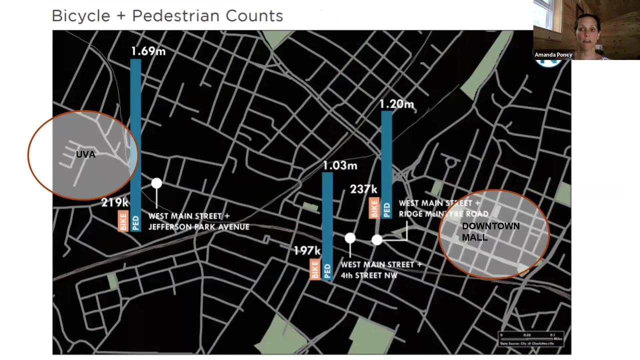 see, And you know, of course, during the planning process staff and local advocates were very vocal that you know we needed some improved facilities here on this corridor. The consultants who were working on the plan estimated about 200,000 bike trips using the manual counts. 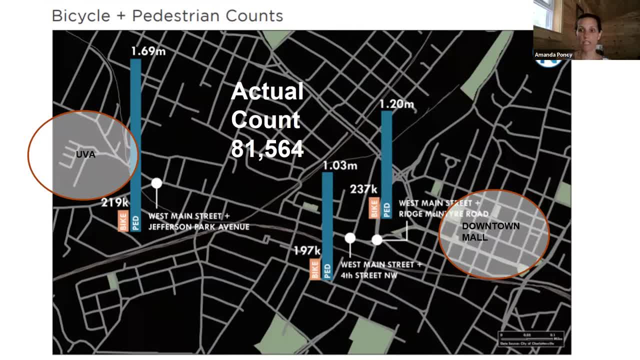 conducted by the PDC, And when we counted in 2015 with our EcoCounter tubes, we found that closer to 81,000 people were biking along the corridor annually. And this makes sense, right? You've got seasonal factors, You know. we also have found that. 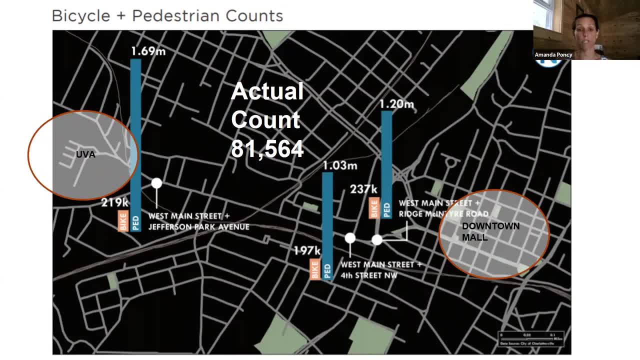 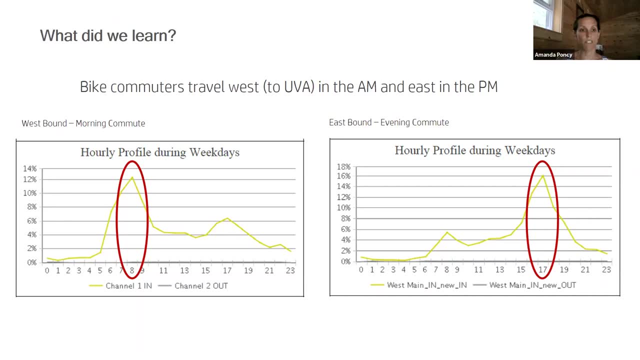 our counters are—our biking is heavily influenced by the academic calendar and so there are—it's not easy to make a straight-line projection using manual counts, So these are much more accurate. So I mentioned that we relied on the built-in reports and the EcoVisio software, and you 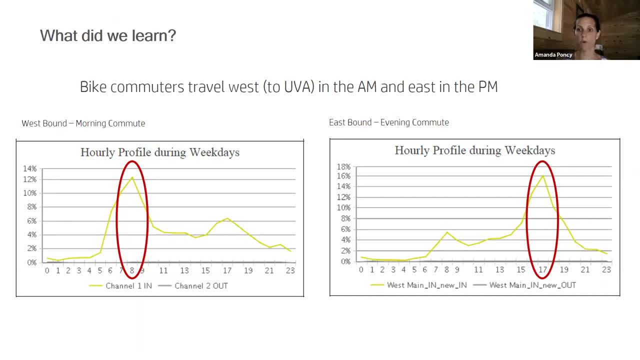 can see a couple of examples here, and the next few slides will show some more. What we found was that we confirmed our bike trips and we found that there was a significant increase in the number of people biking along the corridor. Then we confirmed our suspicion that this is a commuter corridor with bicyclists traveling. 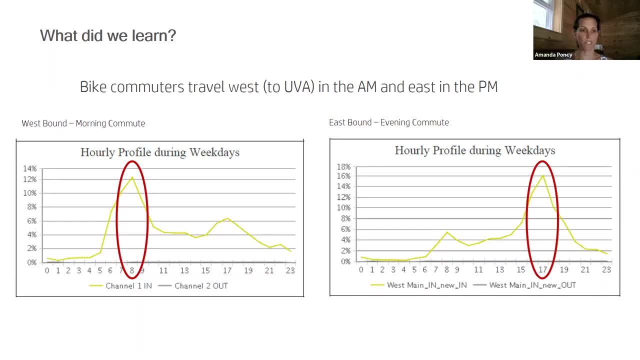 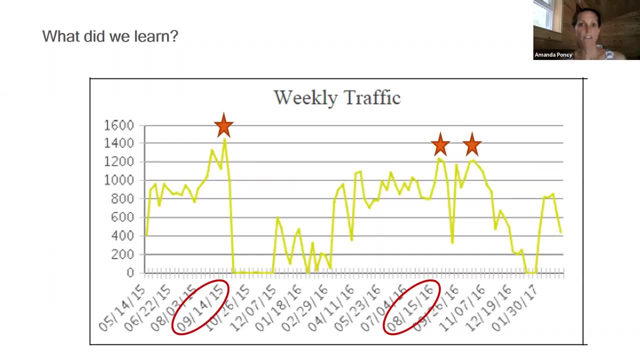 towards UVA in the morning and you found, in the afternoon. you can see the spikes at 8 am and 5 pm in the day. We also found that bike traffic is influenced by UVA's academic calendar. However, the commuting pattern does exist year round, which suggests that full-year 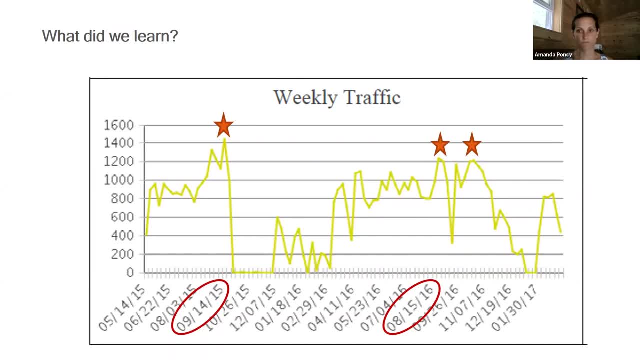 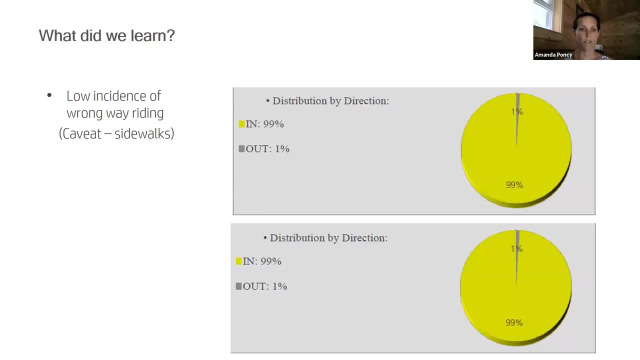 employment at UVA really drives bike traffic in our city. We also found that there was a low incidence of wrong-way rickshaws, wrong way riding on this facility. I do want to note the caveat, though: These counters were placed in a bike lane that was directly adjacent to the sidewalk and didn't necessarily count. 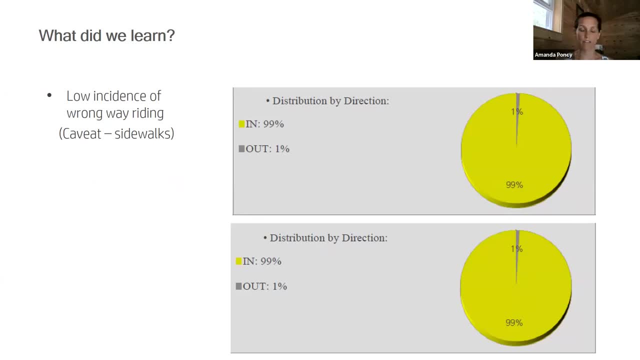 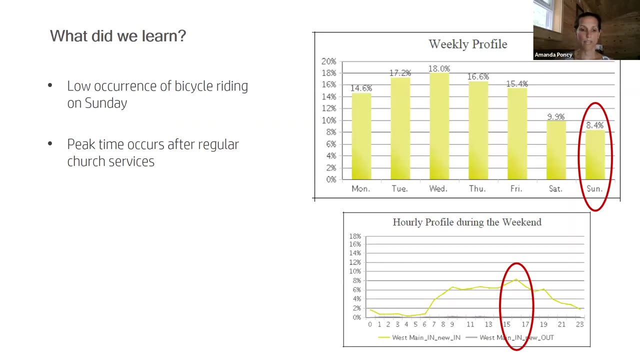 people who were riding on the sidewalk. So these are just the people that are riding in the bike lane. Lastly, one of the major stakeholders for the planning process on West Main Street was the oldest African-American church that was located directly on the corridor, And many of the church. 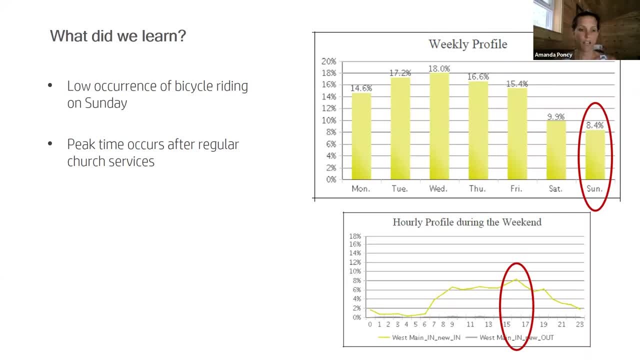 leaders were concerned that people riding bikes would be zooming along in front of the church on Sundays while people congregated before and after services, And with our EcoCounter equipment we were able to show that there was a low occurrence of bike riding on Sunday and that 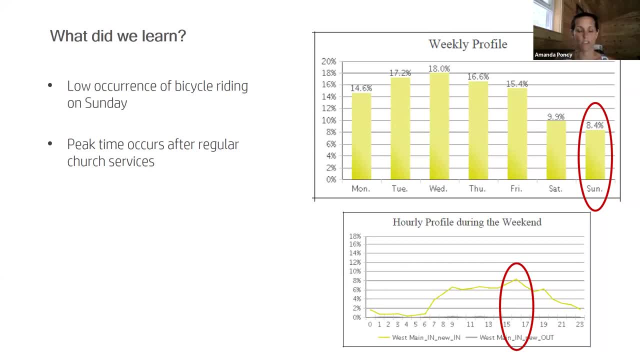 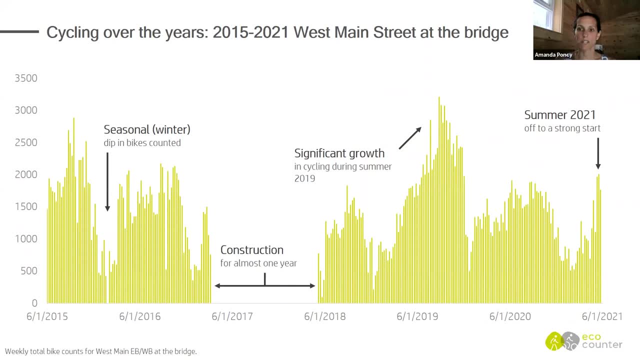 peak usage actually occurs after church services, which is the graph down on the bottom. So the next few slides show some of the analysis that EcoCounter did for us as part of the competition. One of the questions that I wanted to answer is: what is the change over time on West Main Street? So you can see here in this graph that 2015 was. 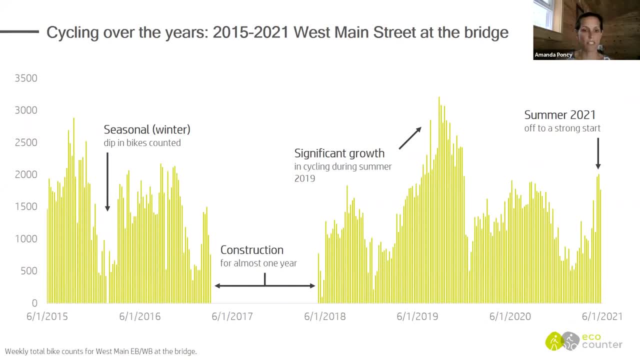 our base year and we had pretty good counts. You can see throughout the years that there's a seasonal dip in the winter. I think that this is certainly weather-related, but in some cases, related to the academic calendar, as well as the fact that we often will take our equipment off of. 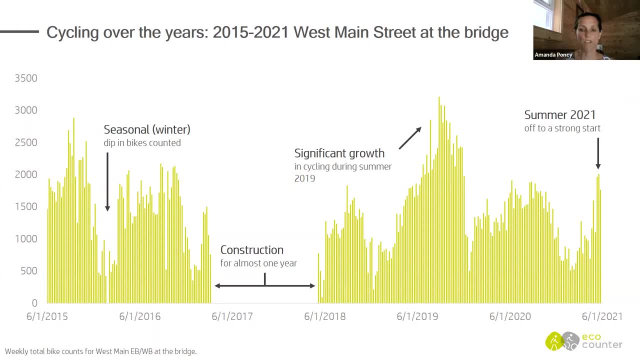 the streets when we predict snow is coming. We also took the counters offline and we also took our equipment off of the streets when we predict snow is coming. We also took the counters offline in 2017 to 2018 because we had some construction. Again, we saw significant growth in 2019,. 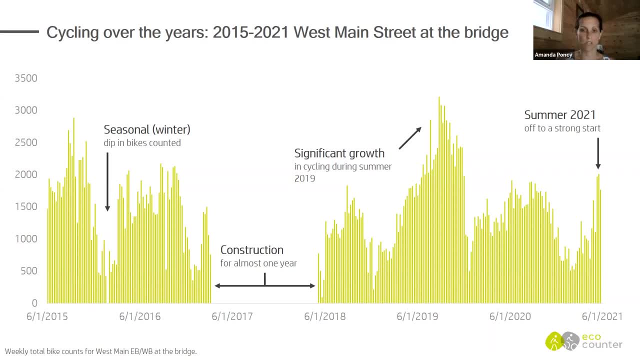 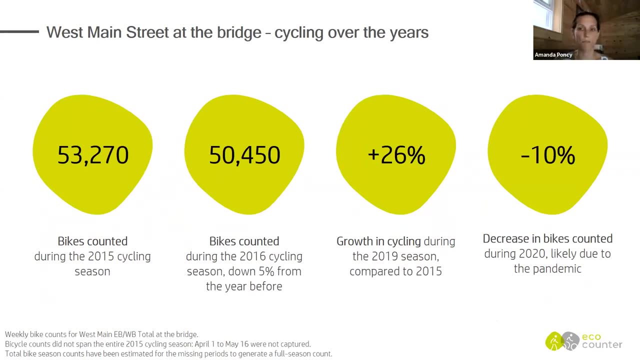 and then a dip in 2020 due to the pandemic and people not commuting to work. This slide tells a similar story, but focuses on the months of April to October. The base counts in 2015, during our cycling season, was about 53,000.. They dipped to 50,000 in 2016,. which represents a 5.5 percent drop in the last year And that took a lot of time to develop. The base counts in 2015, during our cycling season, was about 53,000.. They dipped to 50,000 in 2016,. 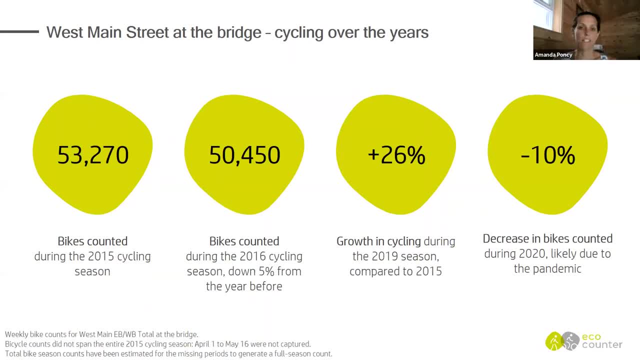 which represents a 5.5 percent drop in the last year, And they took the counters offline in 2017 to 2018 because we had some construction percent decline. You know, in reality, I think this decline probably doesn't represent a decrease. 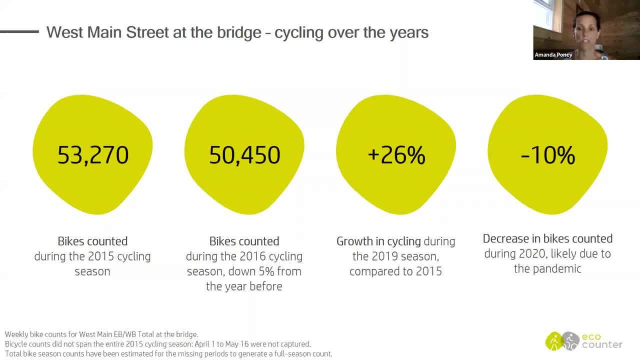 in people biking, but a decrease in the number counted just simply due to the construction work adjacent to the corridor. People were likely either sharing the travel lane or they found an alternative route. We also saw significant- or you know I mentioned we saw significant- growth. 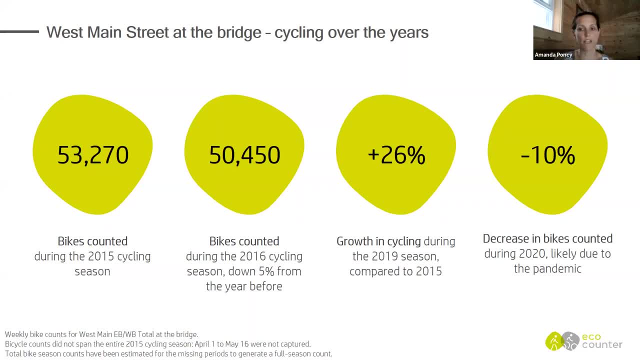 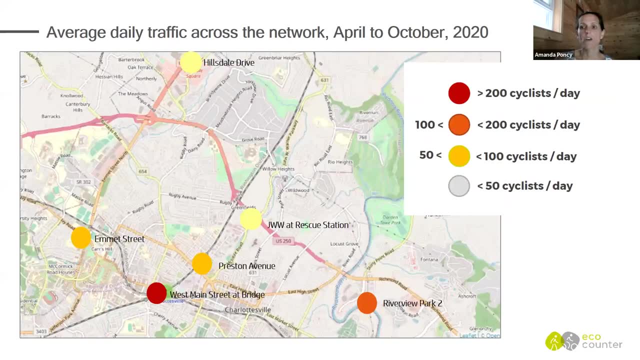 in 2019, with a 26 percent increase compared to 2015, and then a 10 percent decrease in 2020 due to the pandemic. I also wanted to find out overall how our count sites compare to one another. This is a snapshot of the average daily traffic across the network in 2020, and what you can see. 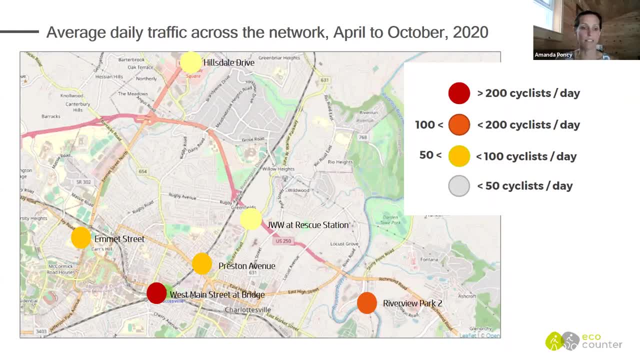 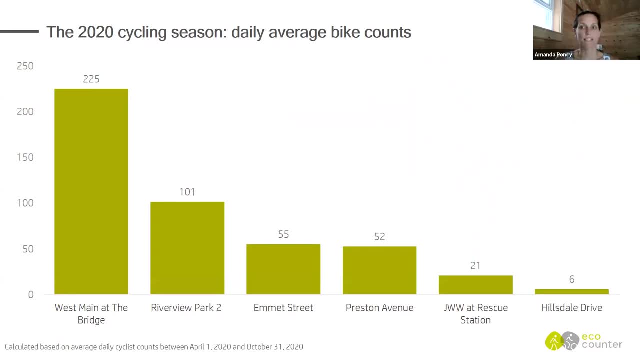 is that, even though the counts were down for West Main Street in 2020, it still is the highest bicycle activity corridor in the city. Bar graphs are another way to present the same data and this you know. when I look at this, it tells me that our commuter corridors West Main Street, Emmett, 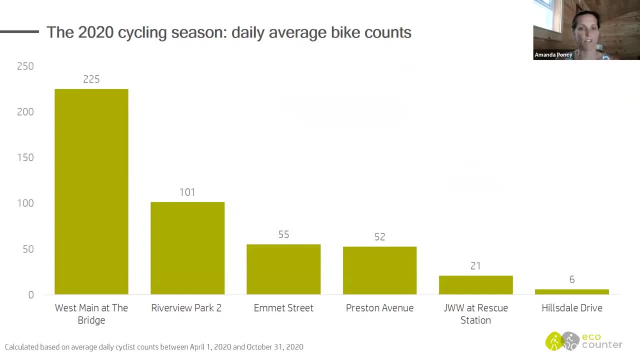 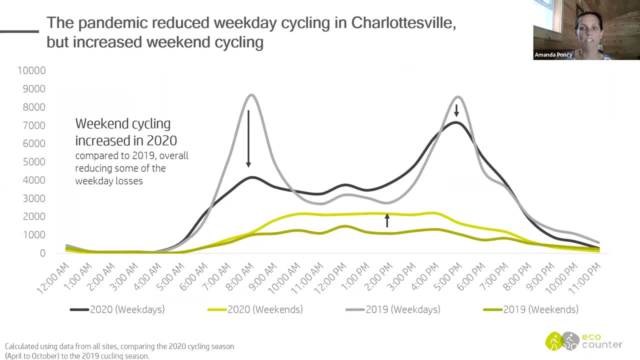 Street and West Main Street are the highest bicycle activity corridors in the city. Preston Avenue have higher daily bike traffic than our recreational corridors. EcoCounter has been analyzing commute trends worldwide during the pandemic and I wanted to know what those trends look like for Charlottesville. So the black and gray lines here represent the 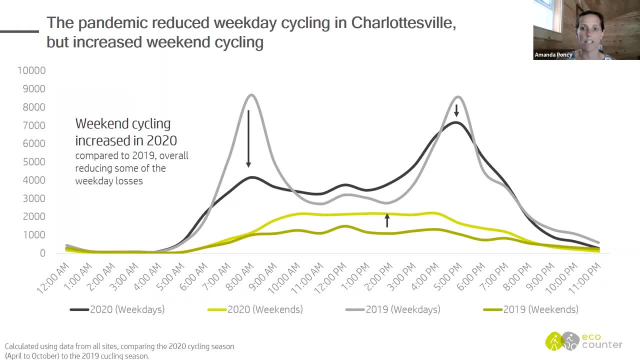 weekdays and the green represent the weekends. You can see here an increase in the weekend cycling and a decrease in the weekday cycling. However, the weekend increases didn't seem to make up for the weekday decrease, So I wanted to find out what those trends look like for Charlottesville. 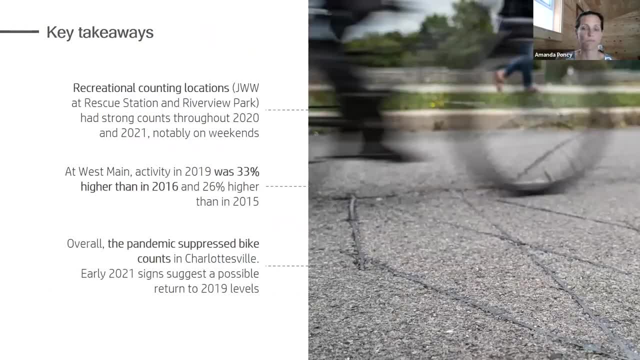 So some of the key takeaways from this competition. overall, EcoCounter found that our recreational counting locations had pretty strong counts through 20 and 21.. However, our commuter corridors still seem to be the primary source of our counts. in the last couple of years, Bicycle counts on West. 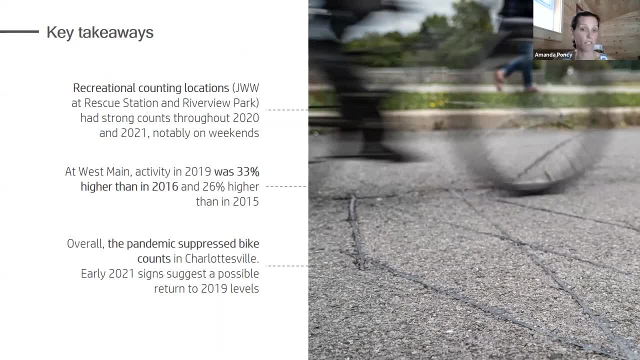 Main Street increased 33 percent between 2019 and 2020.. And so you know we've been seeing a lot of increase in the weekday cycling. So I wanted to find out what those trends look like for Charlottesville. So I wanted to find out what those trends look like for Charlottesville, And so you know we've been 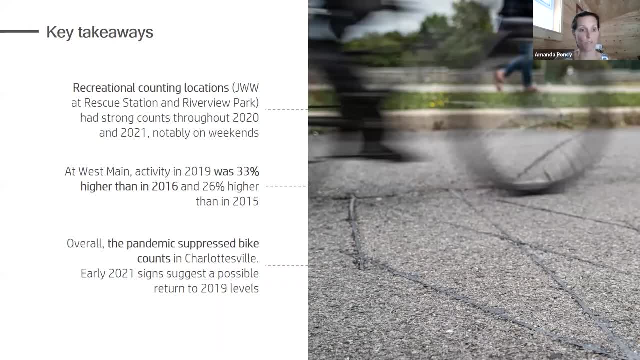 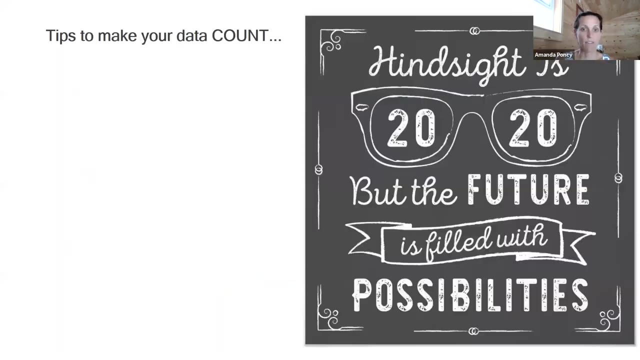 looking at 2019 and 2016,. and they were 26 percent higher than 2015.. And you know, as I mentioned, overall the pandemic suppressed bike counts in Charlottesville, But the early 2021 signs suggest a possible return to 2019 levels. The last thing I want to do before we end is just: 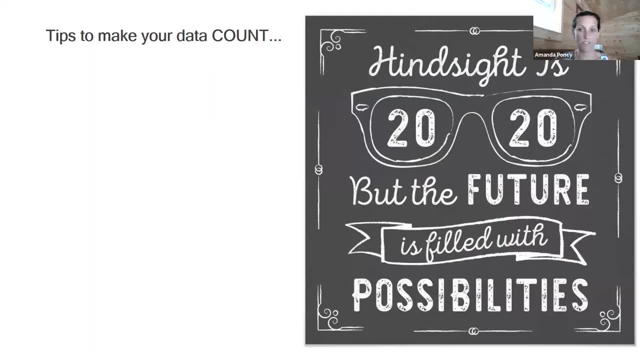 to share some tips to make your data count. So when you start an account program, there are going to be some things that you don't anticipate, But I wanted to leave you with some three tips that would help get your program started on the right foot. Tip number one: use the right. 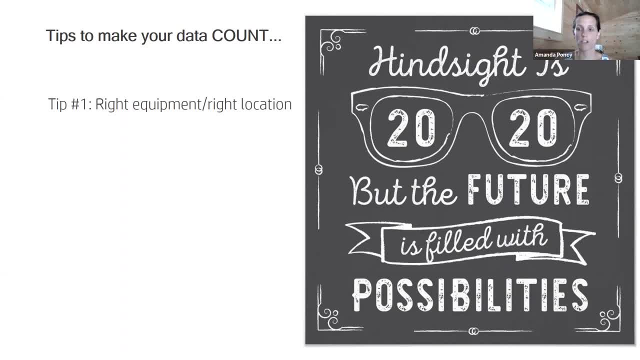 equipment in the right location. We've used our short-term counters for a year or more in some locations. This was more opportunistic than intentional, because I found I didn't have the time to continually move the counters from site to site and I'd rather be counting something rather. 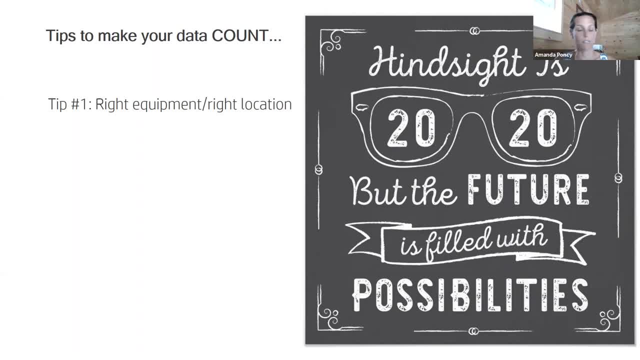 than having this great equipment sitting on the floor of my office doing nothing. I don't recommend this approach. Before you purchase any equipment, know exactly what you want to count, where you want to count and for how long you want to count. Visit the site, take pictures. talk to the staff. 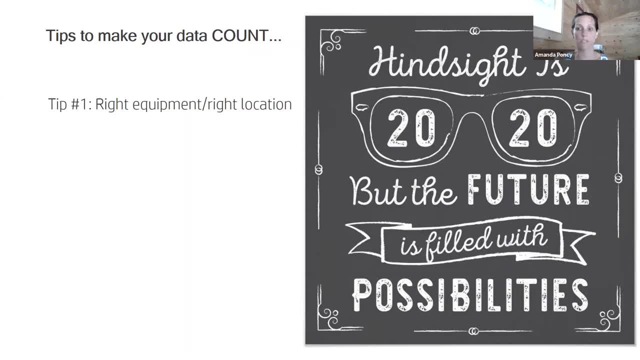 at EcoCounter. They can help confirm that the equipment you want to buy is appropriate for the site before you spend the money. This will help ensure you have valid data moving forward. Second tip number two: have a plan, Because our equipment slowly grew over time and I was eager. 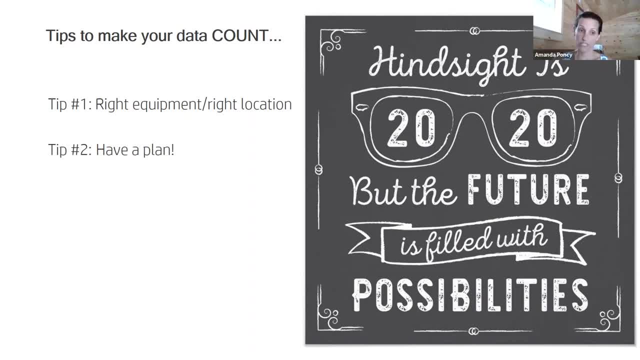 to start collecting data. when it arrived, I was more opportunistic again than methodical. Three years later, I found myself trying to recreate which counters were installed, when and where, And so, if you're using short-term counters, have a process to document. 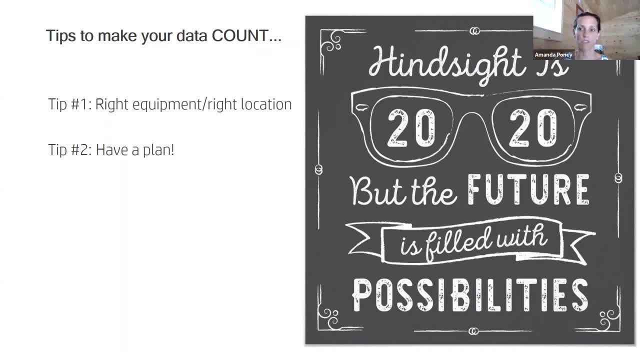 the dates and locations of the installations before you install them, so that you can have confidence in your data if you decide you're going to do any sort of historical analysis. If you're installing permanent counters, you know, have a plan to install the equipment when it's. 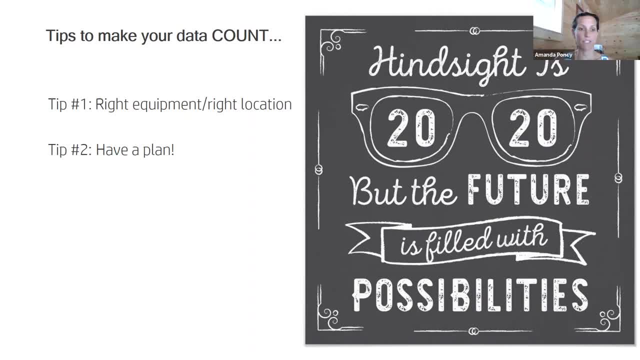 received. I had to get a replacement battery for a brand new counter that sat on my floor for two years. It took us that amount of time to figure out a place to put it. Lastly, validate your data. Take the time to validate your data Again. this is something. 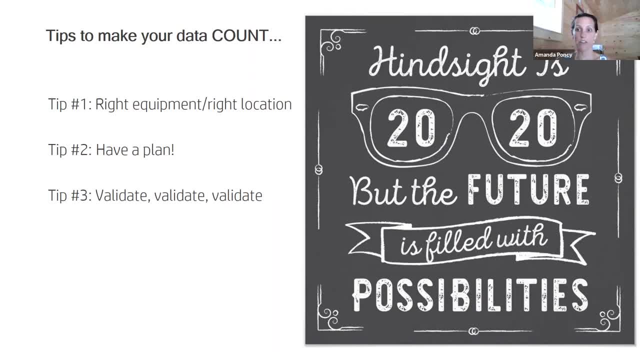 that we did not consistently do Schedule time to make sure the counters are actually working properly. Your count equipment could be overcounting or undercounting depending on how you installed it. This is also a really great time to observe the qualitative characteristics of your count population. Are they male? Are they female? Are they people of color? 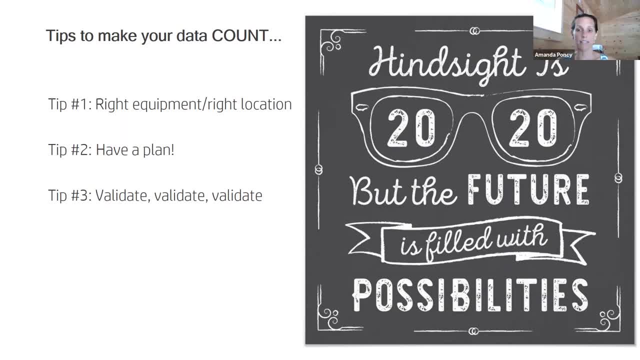 Are they wearing helmets? Are they riding the wrong way on sidewalks, Things like that? So hindsight is 20-20.. I wish I would have known all of these things when I started the program six years ago and I hope that if you're starting a program, that you find some of these tips helpful. 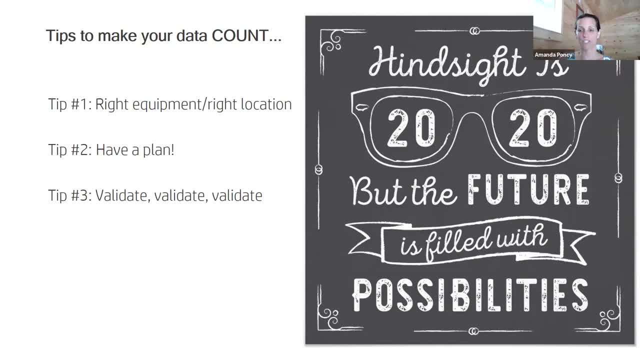 I know I'm looking forward to taking my own advice as we look forward to the start of the new school year, and I want to thank the League of American Bicyclists and EcoCounter for providing this opportunity and the inspiration to help make our data count. Thank you, 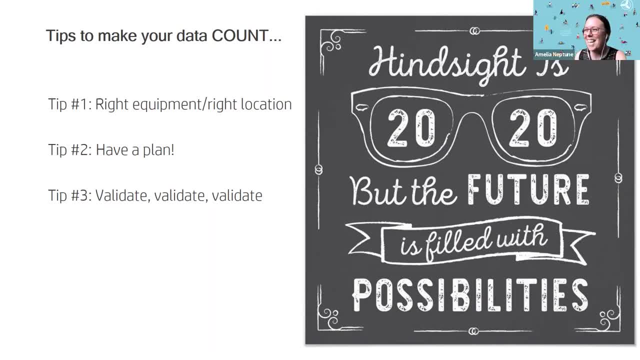 Awesome. Thanks so much, Amanda. All right, We're going to next pass it off to Mike- in Boise, I think, while he's getting his slides up and Amanda unshares her screen, which might need to happen before Mike can share his- I'm not sure. I just wanted to say that it. 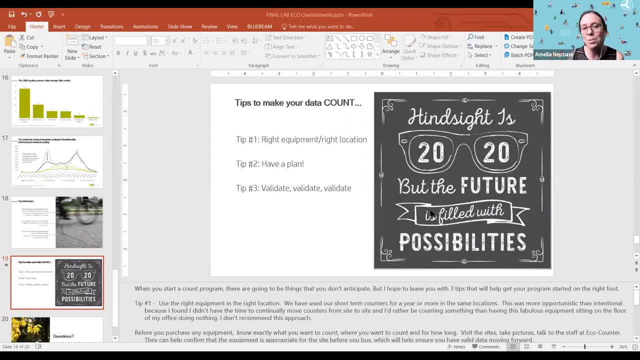 was fantastic to have some data that EcoCounter was really familiar with, but it wasn't a requirement for this competition. But it wasn't a requirement for this competition. But it was fantastic to have some data that EcoCounter was really familiar with, but it wasn't a requirement for this competition. 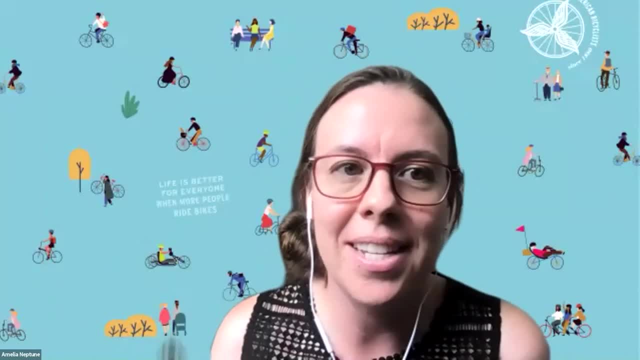 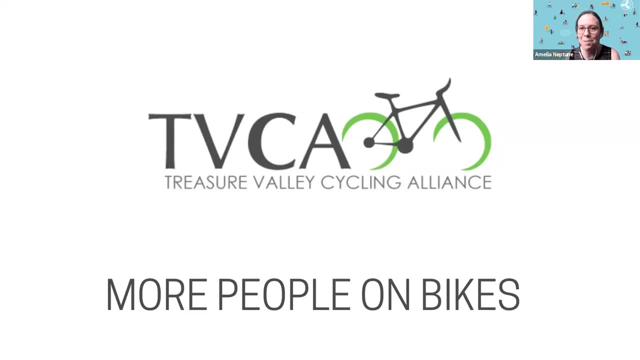 And so in our next presentation you'll see, The advocacy organization award went to a group with all manual counts, So and we're really excited for the opportunity to sort of compare those two. So Mike Jonas lip, who will be speaking next, is a volunteer board member of the Treasure. 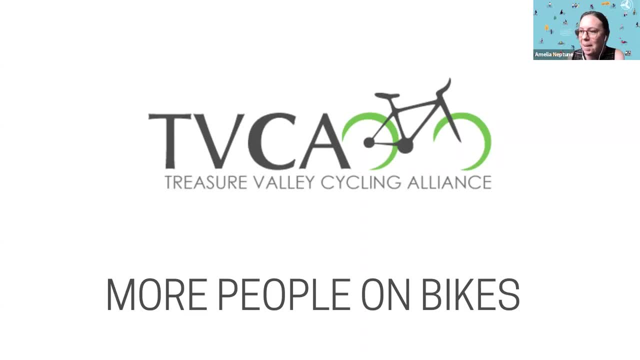 Valley Cycling Alliance in Boise, Idaho, and he creates empowering learning experiences that transform our communities for greater inclusivity. Adam is an established executive officer in the founders ofidian banking. He in his day job at Boise State University Through his own engagement. 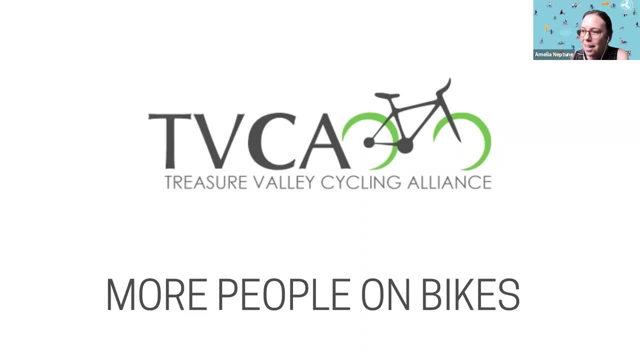 he is a regular at neighborhood, city and bike events that make the community more complete and vibrant. Mike sees bikes as a vehicle for social change and strives to make biking more accessible to all. When he's not advocating for bikes and infrastructure, he's riding with his family. 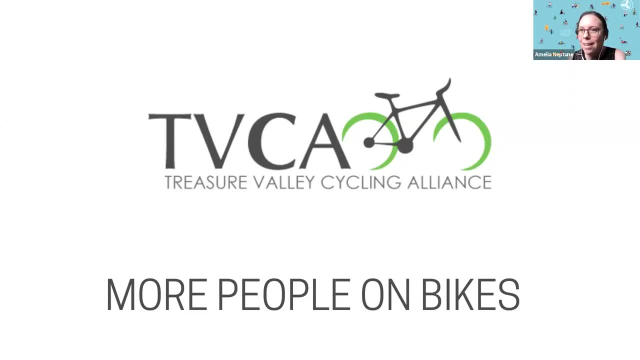 So thanks, Mike, And I will pin you so that everyone can see you put the spotlight on you- Awesome. Thank you very much, And thanks to the League and EcoCounter for all of their work in selecting us. We feel very honored. 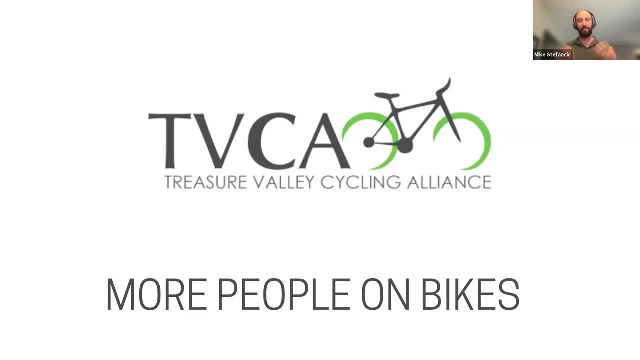 We feel like the little folks out there, And so it's great to have that honor and recognition. So it really gave us an extra boost of confidence in the work that we're doing. So thank you for that. So I want to share a little bit about our organization. 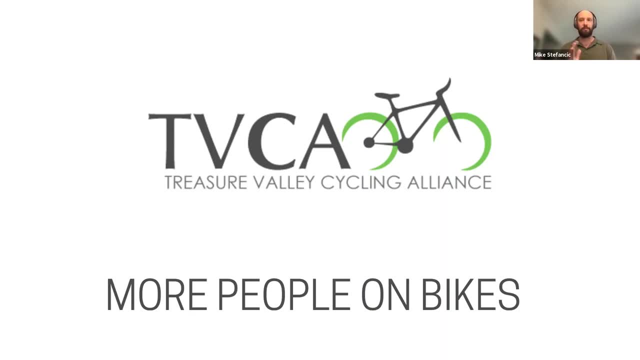 And then I'll jump into some of the analysis that we received here. So I'll have to do a quick. so bear with me on that. So there will be a down second in between here. So we're a small organization of all volunteer run. 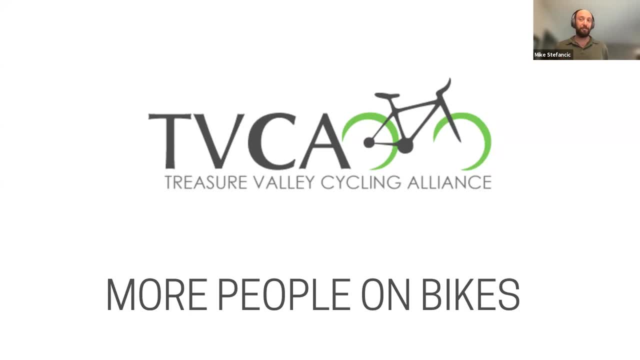 no paid staff. We'd love to find some paid staff, And hopefully some of our data will help us advocate for that, And so this might actually push us into that realm, And really we're just trying to get more folks on bikes. 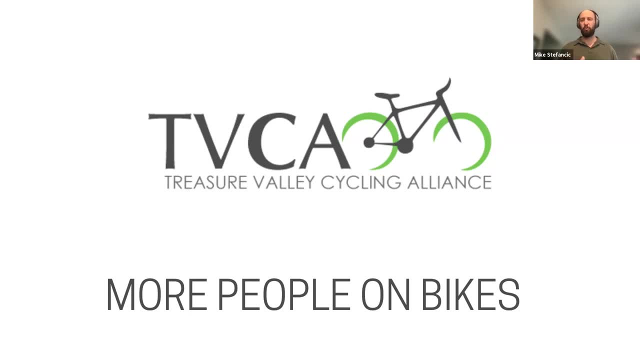 The Treasure Valley is located in southwestern Boise, Or Idaho, sorry, And Boise is the capital of Idaho there, And we are one of the fastest growing places in the United States. right now Things are booming in our town And we are growing faster than our infrastructure. 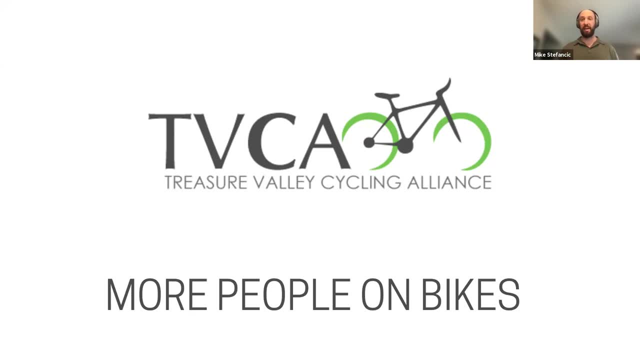 So at this time it is so important that our bike count data has that impact and help our planners really make the best decision so we can have a connected city. And you'll hear me talk about that and really emphasize how we look at our network. 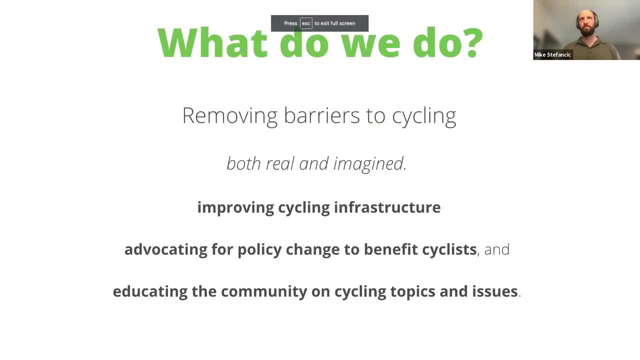 So really getting more people. So we try to remove these barriers to cycling, both real and imagined. We realize that some of that is that what you see, but there's also some imagined barriers to that And so we try to improve that cycling. 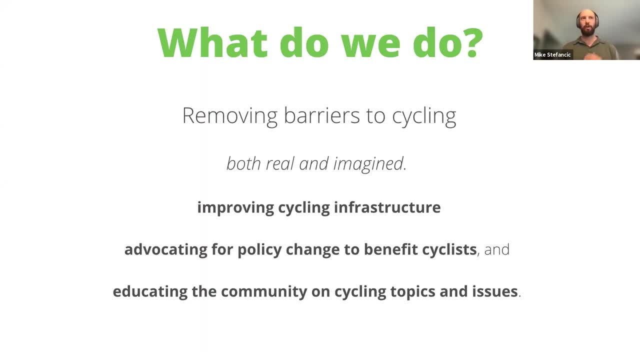 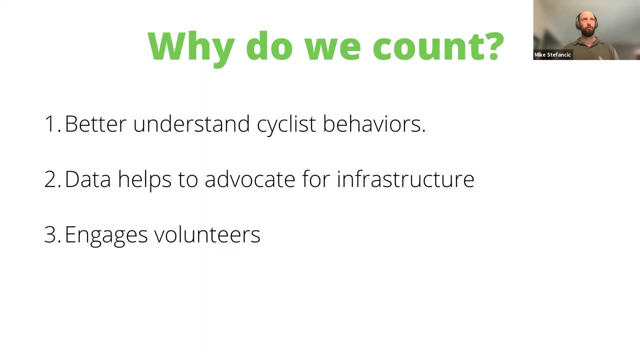 We do a lot of advocate work for policy change And we do a lot of education, And that's a big part of the work that we do as an organization. So why do we do counts? We actually really try to help better understand cyclist behavior. 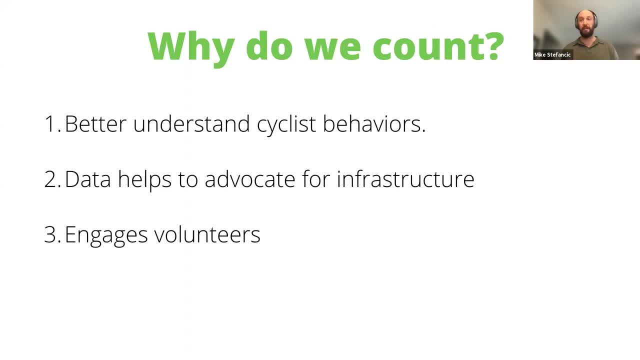 It's really easy to go out there And be at an intersection and just see somebody fly through and be like, oh, that's the one person they represent all cyclists. But the more time we sit out there and we observe cyclists we see these trends. 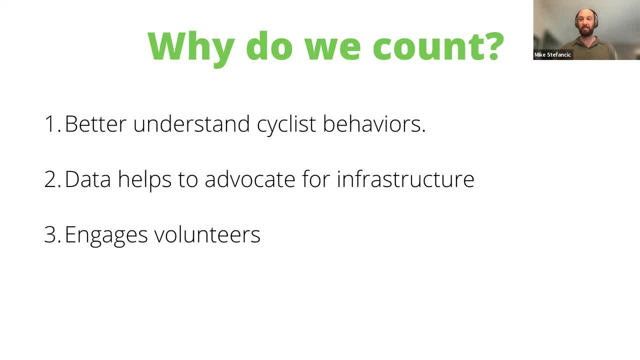 And it really helps us engage our volunteers to see those things. So we don't just have all this anecdotal information about how we're behaving, And so then this data helps us advocate for infrastructure, And we've had some great success in our Valley. 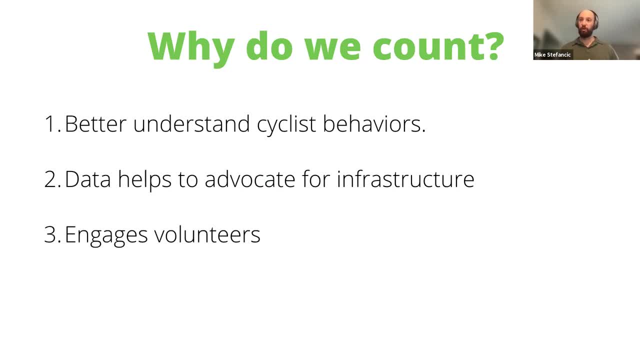 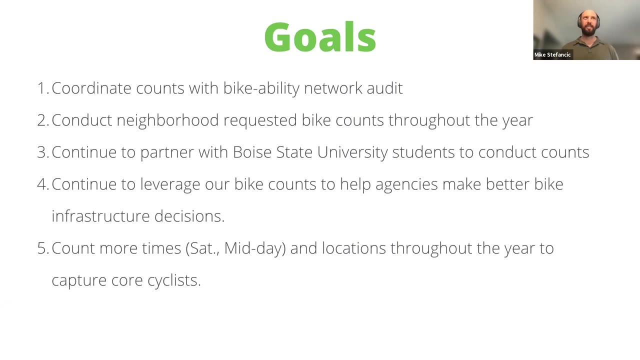 and then engaging volunteers into the work, Because when they see it, when they're engaged, then it helps them become advocates. So we're actually helping to empower our community for that change. So really some of our goals around using bike count data is really looking at our bikeability network. 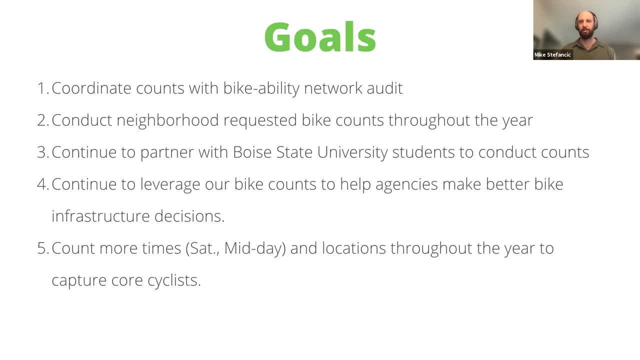 And we do these audits, where we bike around in the community and we take pictures and we talk about the experience And bike counts, help us better advocate for that connectivity in our community as it really grows. We can then also, if we're able to, 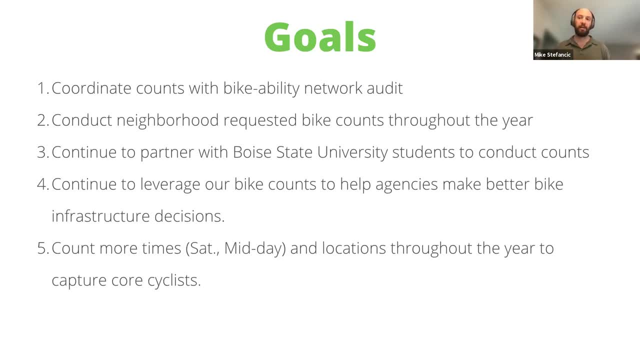 respond to our neighborhoods that are requesting bike counts because they develop community plans So we can get in there and we can say what is really happening within your community in cyclists. So we offer that We can also partner and hope to continue to partner. 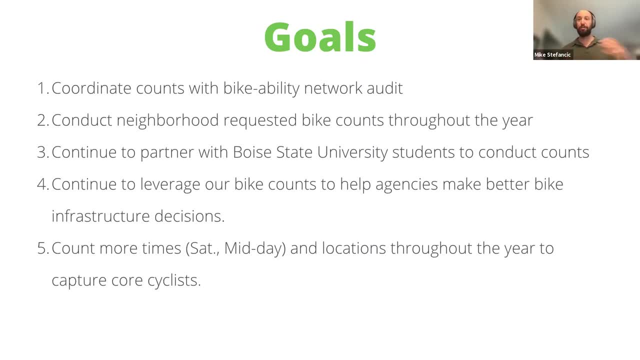 with Boise State University. I'm- luckily I work there, as you heard in my introduction, and it really helps us leverage that resource in the community and the research and the insights that come from there. So you'll hear me talk a little bit about that too. 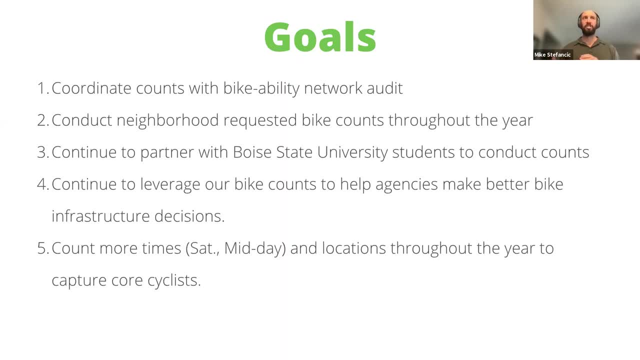 And then we also have the opportunity to talk about and leveraging these to make help our agencies make better bike infrastructure decisions. And Boise is unique in that the city doesn't own the roads. We have a separate highway district. We're probably one of the only towns that does. 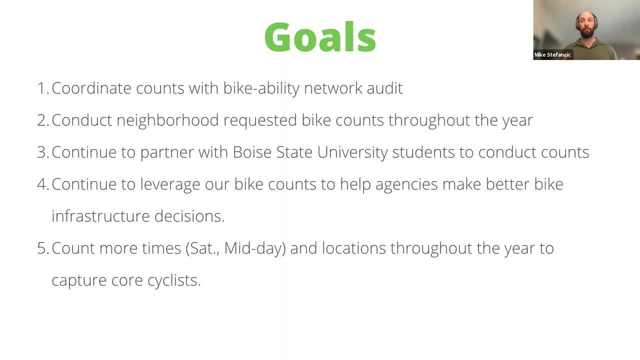 and it makes things a little complicated And when we advocate for that and they're both elected officials on either one of those And then we wanna really count more And you'll hear about this in this data that we had analyzed by EcoCounter really helped us. 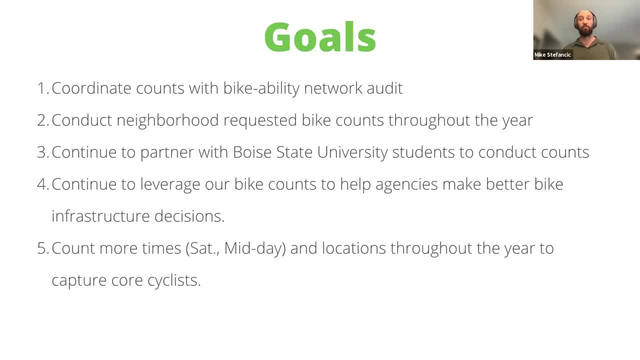 solidify that. the choice to count more is gonna really help us because we have no permanent counters for our organization. The valley does and we have a regional planning authority that does put out tubes and has some permanent counters, but there's only a handful of those. 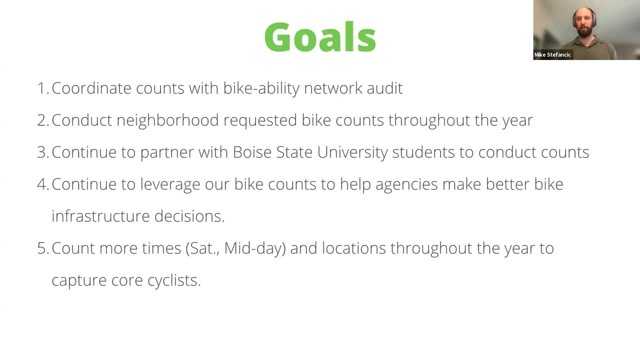 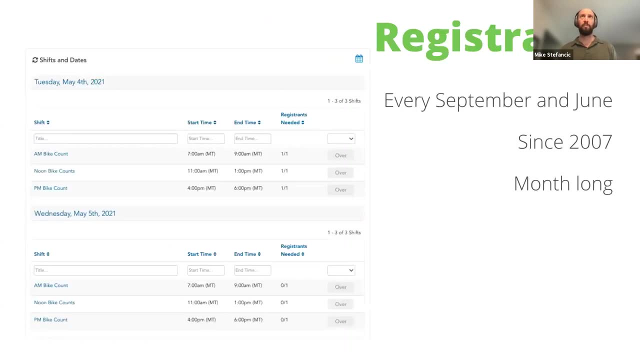 And so we need to count more to get a better trends and ideas, And so EcoCounter were able to actually help us. really need our solidify this as being an important goal And, as I mentioned, I wanted to share with all the folks is how you engage volunteers, because that's so easy. 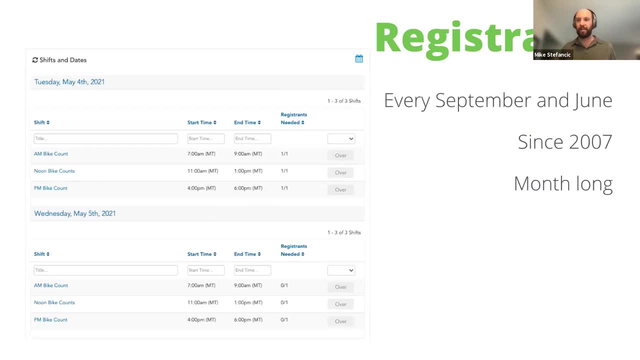 When you don't have funds, you don't have equipment. how do you do bike counts if you have a small group? So it was really important for us to come up with a system to do that, And so we use a registration system and we count every September and every June. We used to only count for three days of those months, but now we're increasing that to be month long, And we've been doing these counts since 2007.. So we have a lot of time to do that. So we have a lot of time to do that. 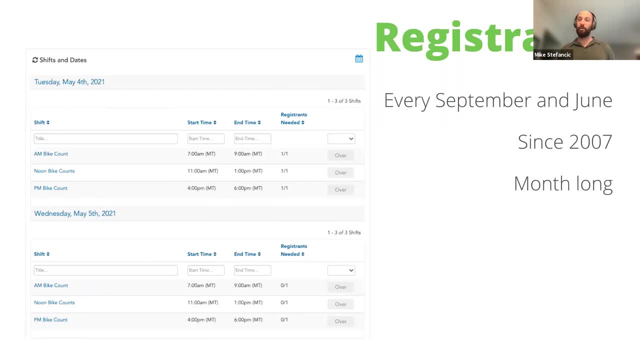 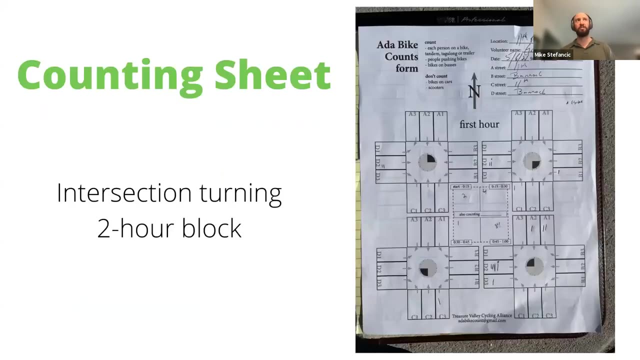 We have a lot of data and sometimes it's overwhelming on how we should do that and how we should tell our story, And EcoCounter is really able to help us do that. So we have a registration process so we can engage volunteers. We do all manual counts. 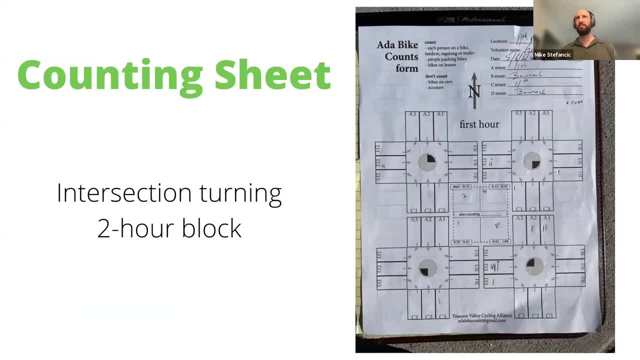 This is what our one of our data sheets look like And this was actually most recent and an important corridor And we identify that and pick locations based on what kind of construction or infrastructure is happening or is not happening. So this 11th street they're putting in a whole new bikeway. 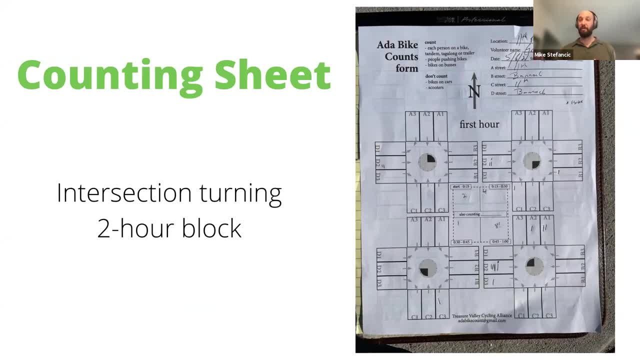 and we're trying to do a lot of pre-counts to find out what it's like before and after, And so we can offer that up to agencies so we can get that insight into there. So we use intersection turning and a two hour block. 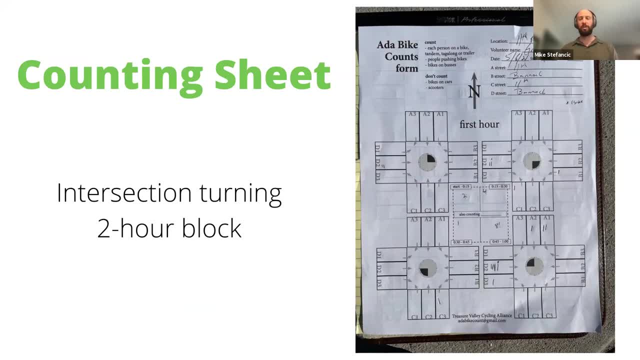 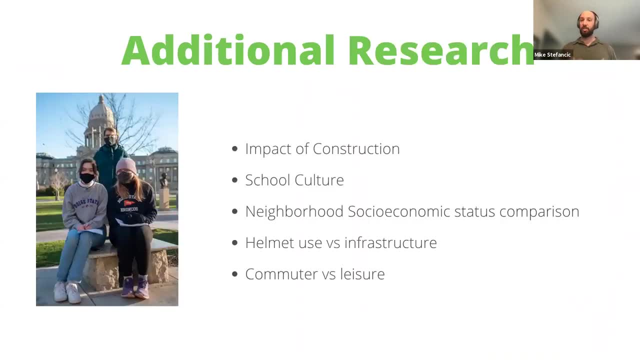 If you have questions about our methodology, I can share that, but I'm not gonna dive into that right now. but all manual counts. And then we're also been engaging the university, as I alluded to as one of our goals, and doing additional research. 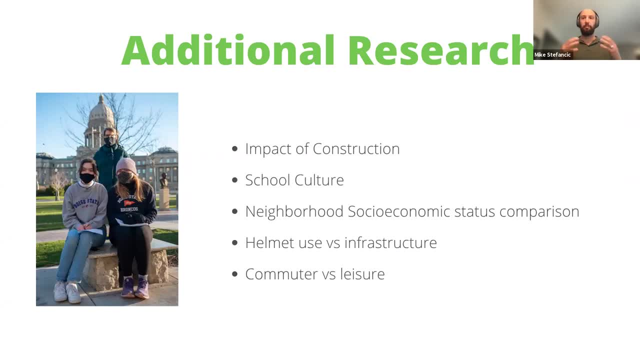 We worked with a class this past summer, last spring, and they came up with a bunch of different inquiries and things that they see as students and faculty members that they would like to better investigate, And so they did some real observations, And so these are some areas. 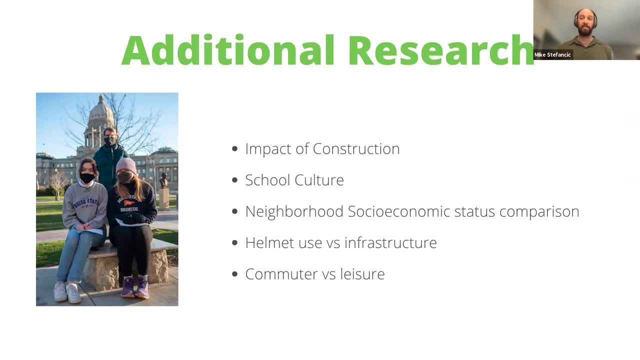 that we're looking to dive in even deeper And some of the eco counter analysis has helped us look better at some of these topics. So students looked at the impact of construction. How did cyclist behavior change when construction was around or around schools? Is there a culture of cycling at schools? 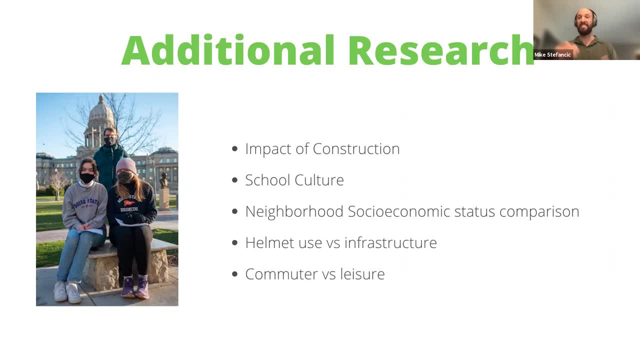 And is there infrastructure that supports cycling to that schools, and did bike counts align with that? We also looked at and compared socioeconomic status in different neighborhoods and what bike rates were in that area, And those are important things that help us find better connectivity around our community. 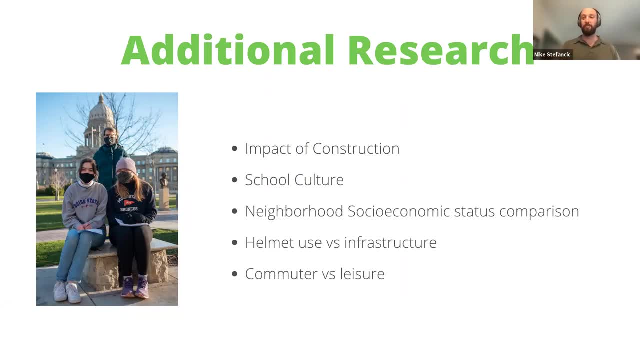 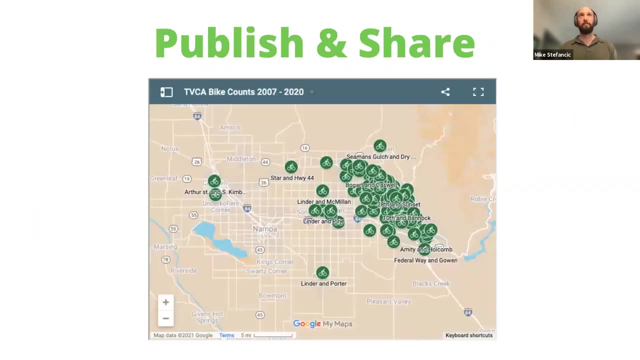 They also looked at helmet use and whether that was used within infrastructure or not, and then commuter versus leisure And this was a really interesting piece because we majority the majority of the time we are counting during commuter times, And I'll get to why that is changing for us. 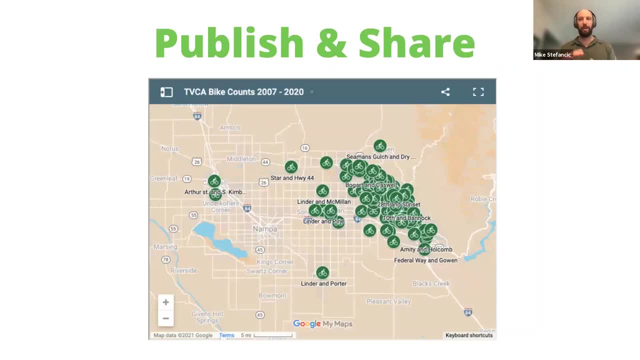 So we take all the data, we publish it out there. Like I said, we have. we don't have a lot of money as an organization. We just put some information out there in Google maps And so we post this on our website. 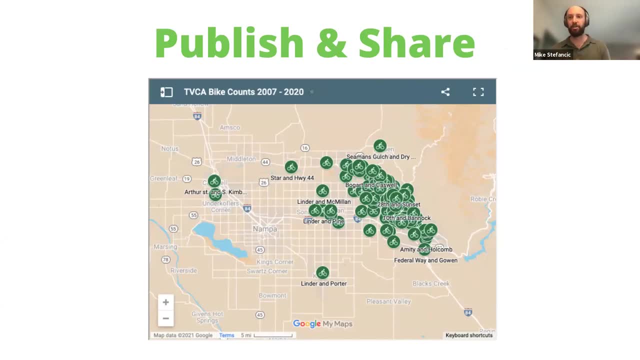 and agencies will reach out to us and ask us: what kind of bike count data do you have for this area? We're looking to make a decision And so we can share that with them. they can go to this website. they can click on them and find out how many times we've counted. 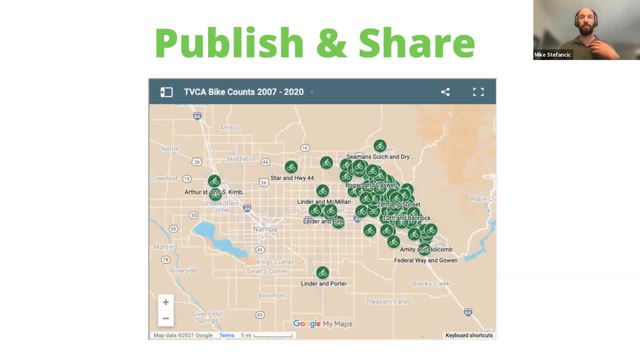 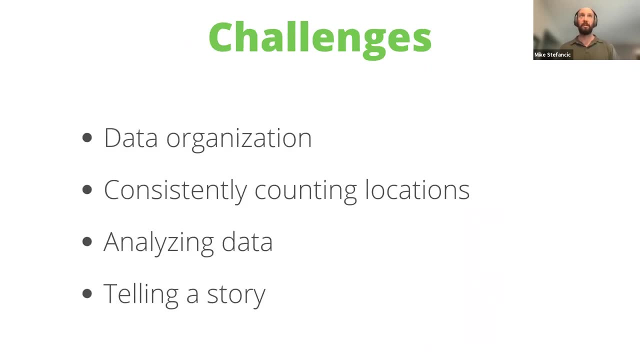 and where we've counted. So we try to share that data, but we don't really have the benefit of being able to put together really nice resources to be able to tell that story. So those are our challenges. really is organizing our data. Like I said, we've been counting since 2007 and we have 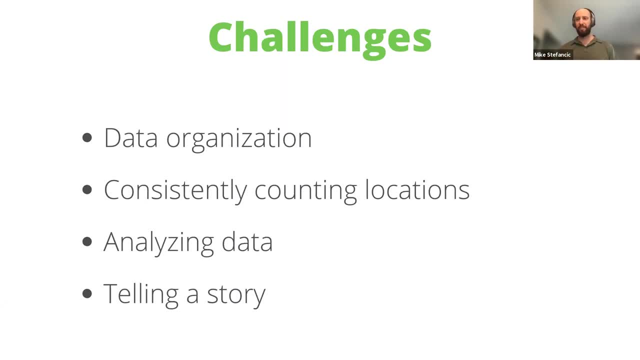 spreadsheets upon spreadsheets, as I'm sure many of you here on this call today have that And you're like: wait, how do I analyze that? And when we started to get to that point, it was overwhelming. We're not statisticians, we're not data analysis. We do things all differently, for 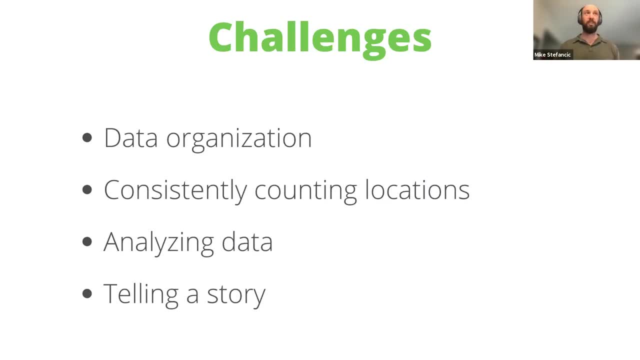 our day jobs and trying to come together and analyze that as a gap and a challenge that we have Then also consistently counting at the same location. Since we all work with volunteers, our volunteer engagement goes up and down, up and down throughout the year. Sometimes we get 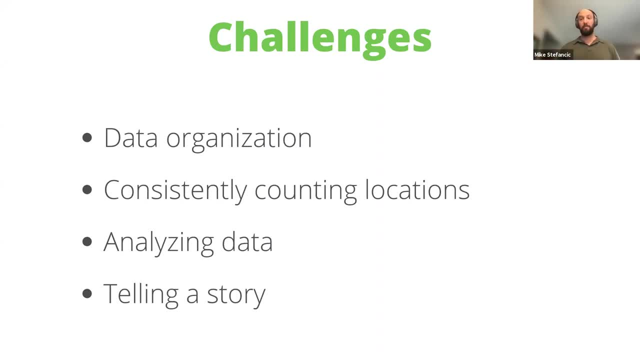 12 counters, other times we get 40. And so trying to manage that and the consistency of that and better being able to communicate the importance of that. Obviously, I talked about analyzing our data and telling our story, trying to get that out there as a small grassroots group of individuals who are 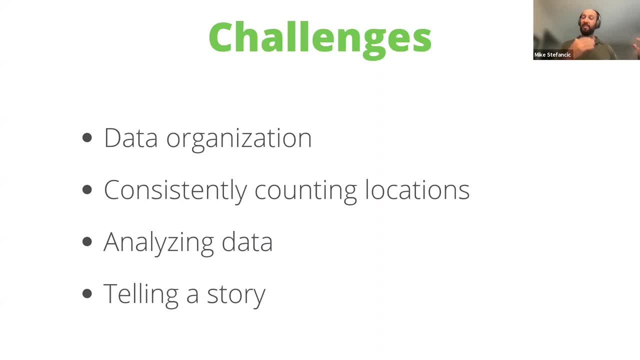 passionate about biking. How do we make sure that our data and the things that we're sharing at board meetings, at council meetings and all of those things are taken seriously? And we do have that, And some of that comes with how you present it. 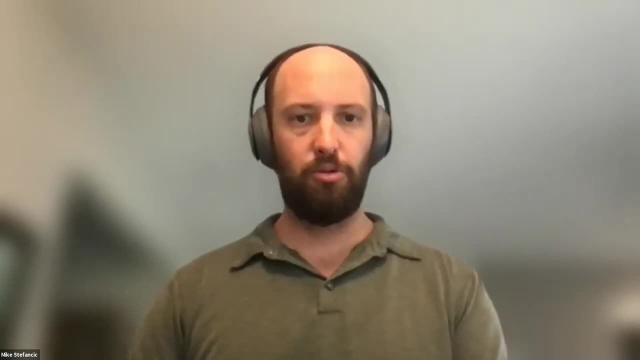 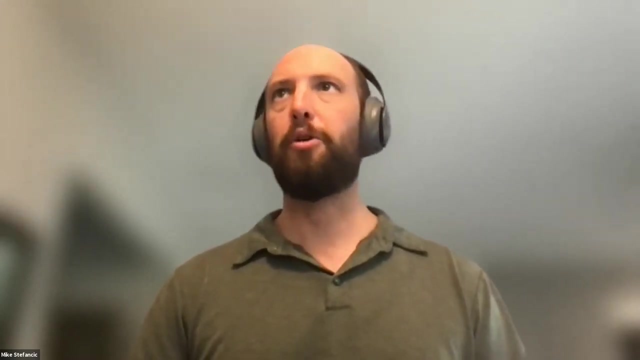 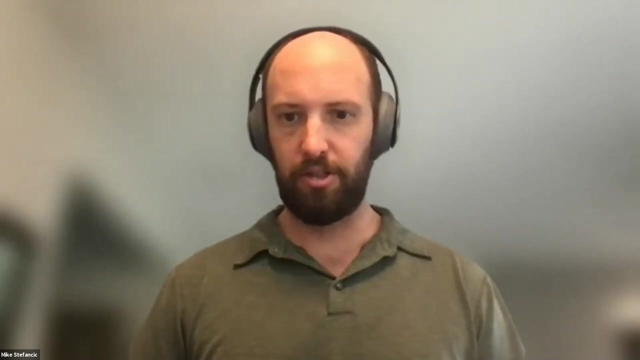 All right. So I'm going to jump out of this and into what information that we were able to gather from EcoCounter, And so, if you bear with me just one second as I switch between these, I hopefully am able to do this pretty smooth, So you should be able to see a map right now. 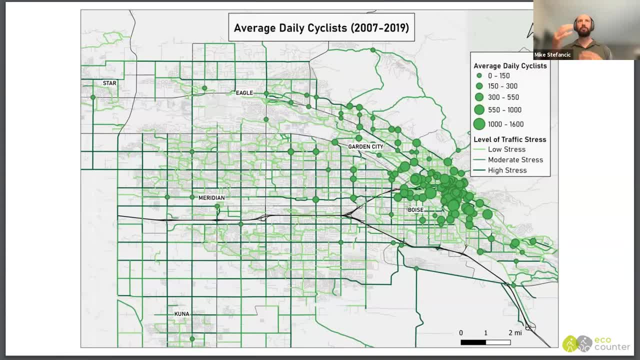 and you see some different size circles and things like that. So you can start to see that map that I showed you before. You saw those counting locations, So you kind of see some of the different size circles and things like that, So you can start to see. 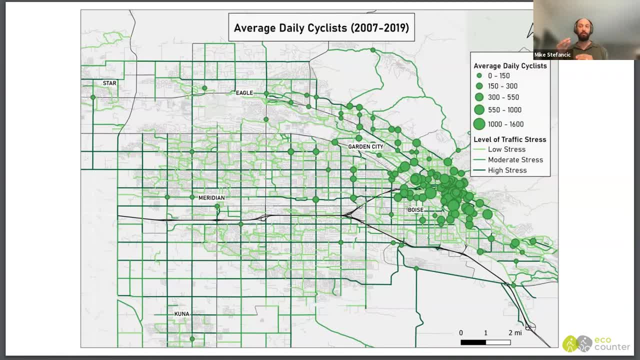 some of those transferred, But now, through EcoCounter, they were able to represent those in different sizes based on what are average daily cyclist ranges. And you'll notice this data only goes to 2019 because in fact, we saw a drop in 2020.. And the reason why is because we 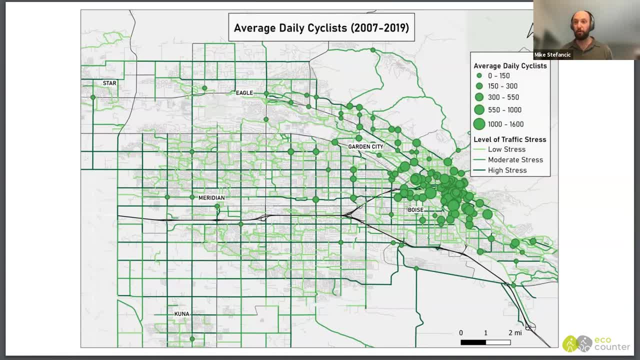 were only counting during commuter times. People weren't going to work, We were missing a whole group of core cyclists out there, or recreational cyclists, because that's how we were set up. We were only set up for a few days, And so we were able to represent those in different sizes based on. 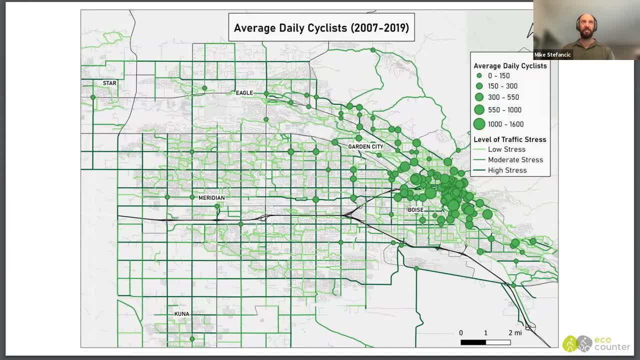 what are average daily cyclist ranges, And so we were able to represent those in different sizes based on that way. So some of this data helps us see that and also see where the frequency is, And, as I mentioned before, one of our goals that we're working on in the Valley is trying to have a 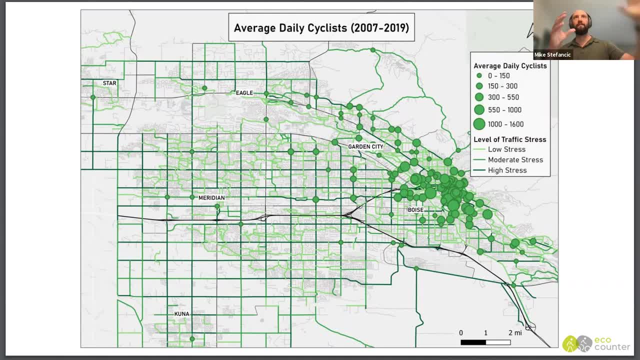 better network And so we were able to start to just really emphasize where are folks coming in? They're coming in from out here in the Eagle, They're coming in off of the bench And these are growing areas And you can see as we spread and grow further out, further out in the Valley. 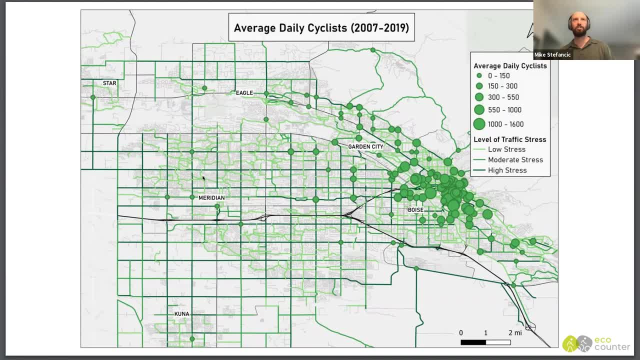 folks coming in to work in this urban setting And some of these corridors, these are highlighted areas And you can see that the green lines, these are some of the bike routes that there are infrastructure. They're not all the same infrastructure, But then this can tell a story right here to some of our land agencies that are 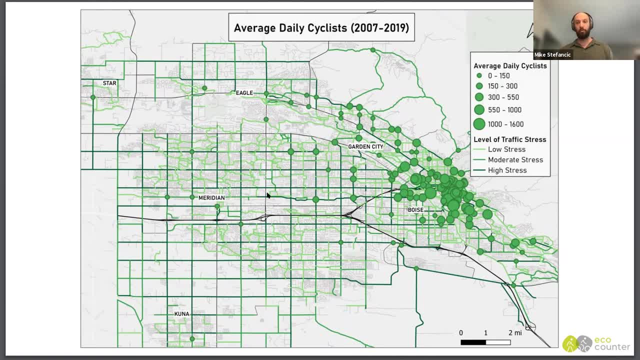 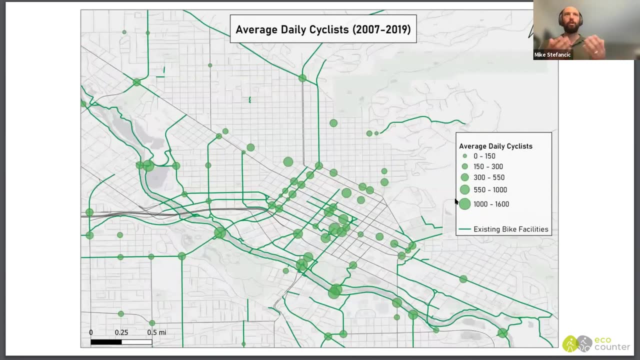 managing these roads is: hey, this is an important corridor. Look at, these increases over time as we grow. So then here's a zoom in. So this area where you're seeing all of these dots, now we're zooming into that So we can start to see where are some of these pinch points. And one of the 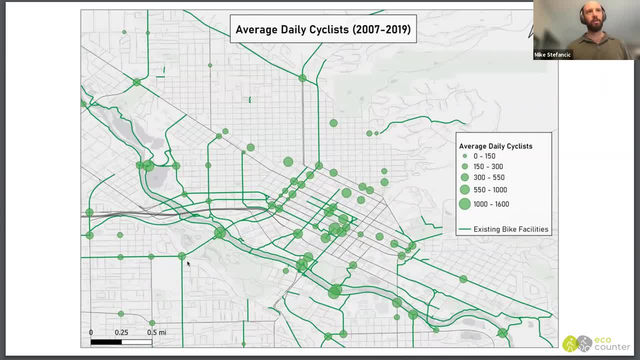 challenges here is you don't see some of this topography. But right here this is a bench, So there is some topography And there's only a couple roads down. This is one of the only ways to go down off of our bench down this hill. But there's all these other important things And the 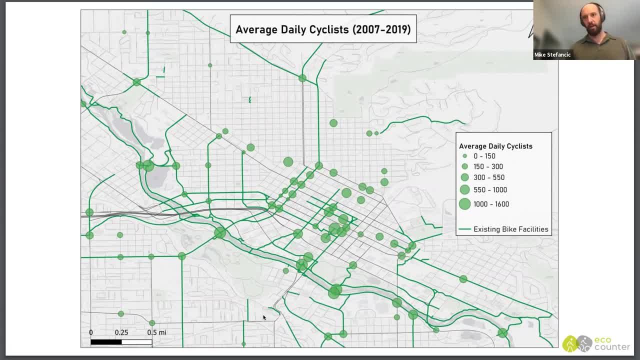 university is right here, But there's not a good way to get down here. So this is going to help us better indicate to our land agencies. This is where we need to put better bike infrastructure. Look at this bike lane. It ends right here. It literally ends on a cliff. It's like, okay, you put that there, But folks need to. 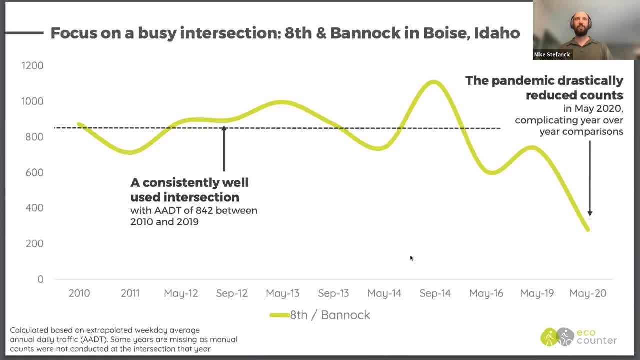 go down So we can use some of this information that's graphically represented here. So, as you imagined and I alluded to, we had a big drop off here in 2020.. Pandemic set in, Folks weren't communicating to work And we had a big drop off here in 2020.. And we had a big drop off here in 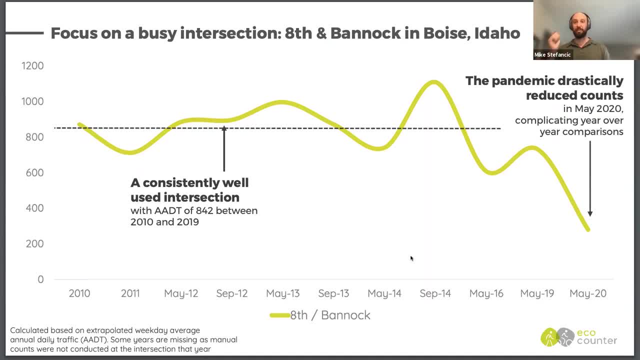 2020.. And we saw that Now this reinforced this graph. when I saw this, I was like yeah, But you know what This really emphasizes: how important it is for us to count at more times and at more days. We only would count Tuesday, Wednesday, Thursday, from 7 to 9 and from 4 to 6.. Only at 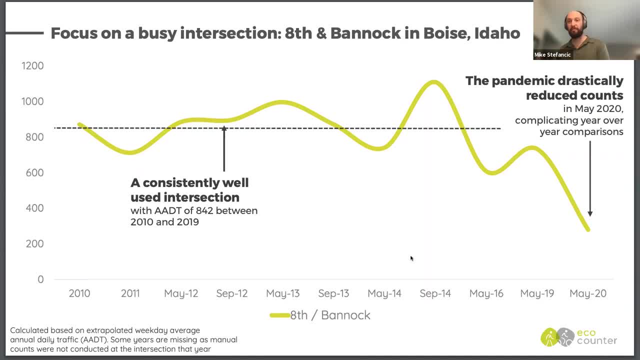 those times. So those are only the commuters. So of course it's going to drop off, But in many of our communities and national data and international data, we saw that numbers actually increased. In some of our permanent counters they saw that numbers actually increased And we saw that numbers. 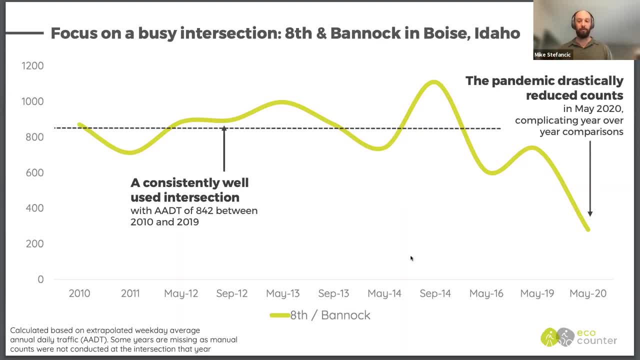 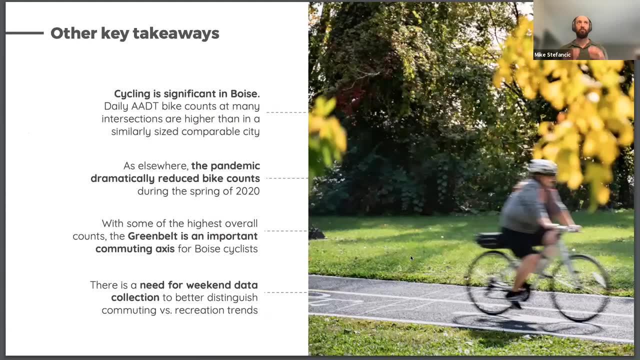 actually increased And we saw that increase. So we're not really counting all of the folks that we need to count And therefore we're not advocating for all of the right infrastructure with some of our data. So really, some of these key takeaways that we got from EcoCounter was: 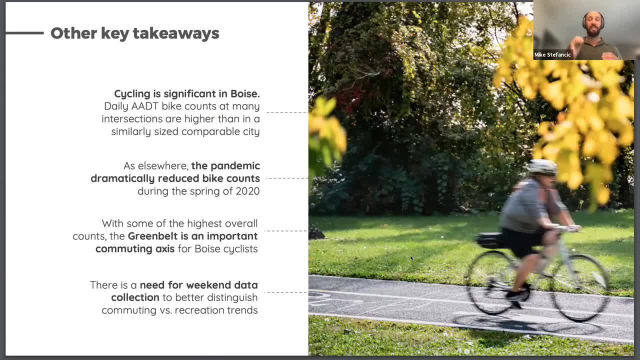 really important for us to say that. you know, cycling is significant in Boise. We've known that. That's why we have an organization, The pandemic dramatically reduced bike counts because we were only counting commuters who weren't going to work. So we need to expand that And we need to 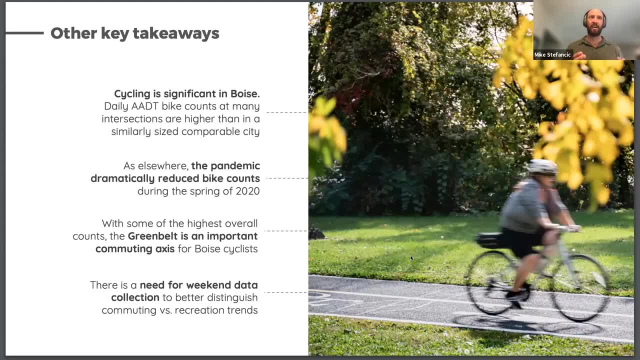 expand our counts. So that was really good information to gather and to see that represented. And, as I mentioned, there's a couple of these pinch points: This green belt and that was right along the river. I didn't emphasize that on the map, But that's a really well-structured 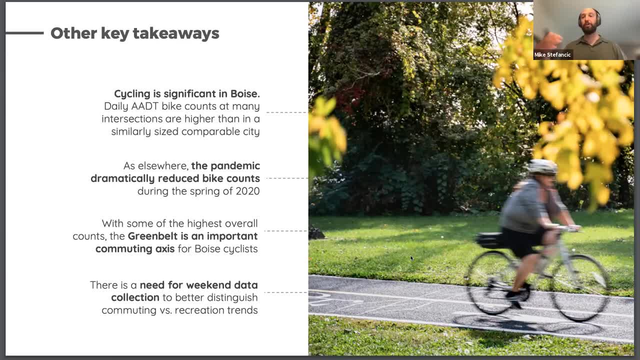 corridor for cycling. How do you get there? How is that part of the network? How do folks get on and off that green belt area And, as I've been mentioning, counting more in the weekend, recreational cyclists or cyclists who aren't in a traditional 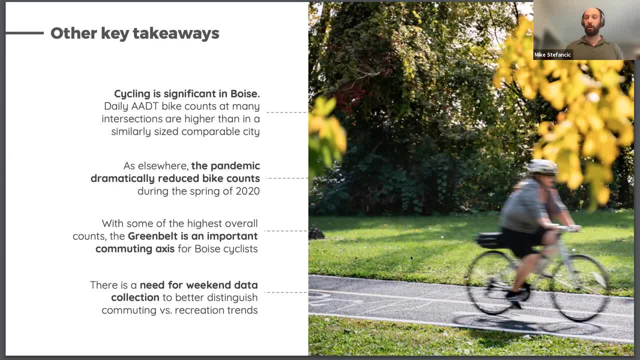 nine-to-five commuting job. So EcoCounter really helped us better emphasize that And we really thank them for the time and the effort that they put in to help us better realize and feel confident in the data that we're using as non-professionals and how we can advocate for. 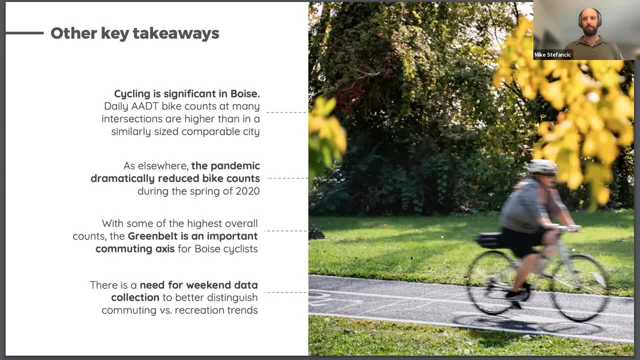 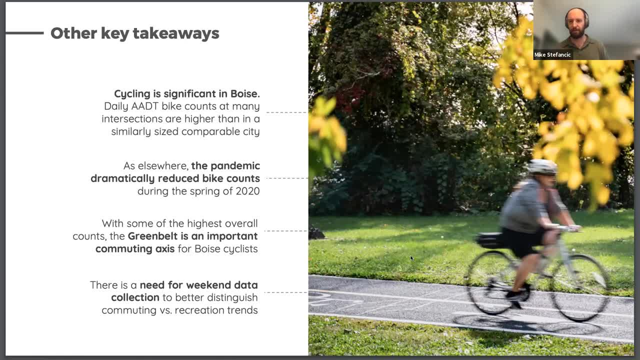 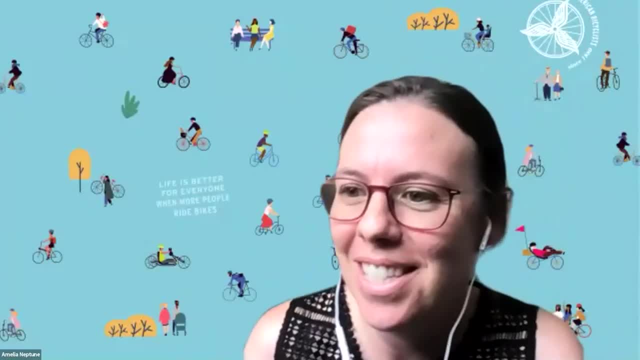 be a time to do that And I'll turn it back over to Amelia. Thanks, Awesome. Thanks so much, Mike. All right, Our third and final speaker I'm excited to introduce is Andrea Shalolo from EcoCounter. She's a client consultant with EcoCounter, where she works with 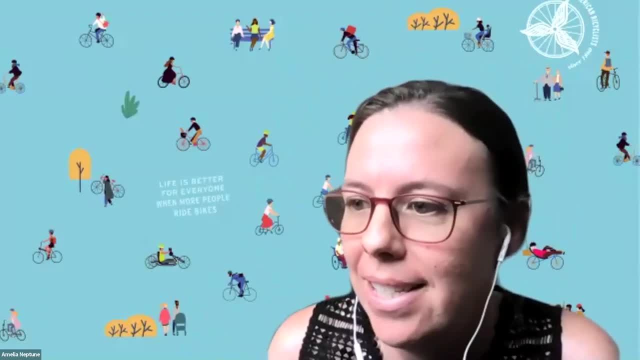 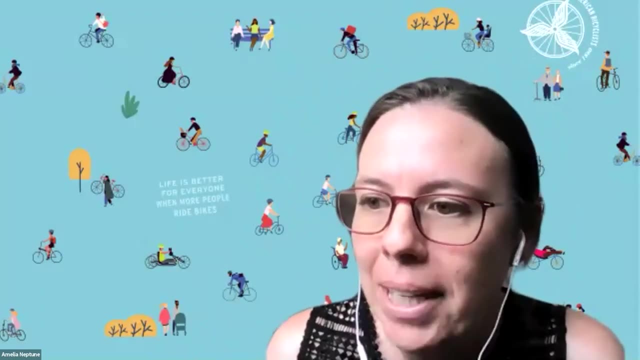 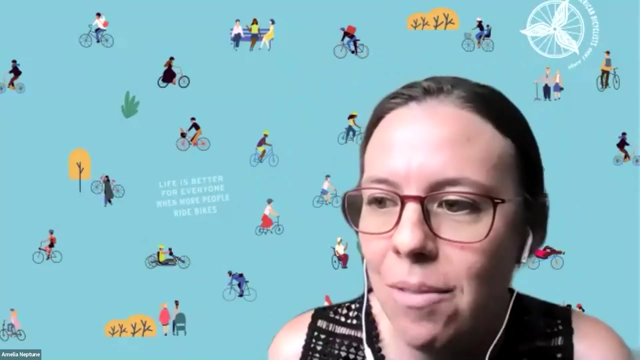 public, private and nonprofit organizations across North America to help them collect, analyze and communicate cyclist and pedestrian count data. As a trained urban planner, she has a knack for helping clients leverage their data to make informed planning decisions And advocate for active transportation initiatives Outside of work. she can be. 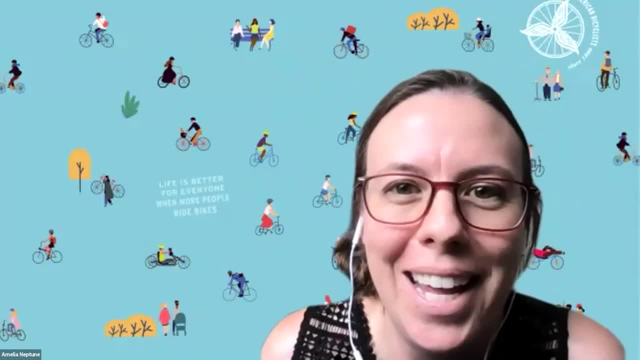 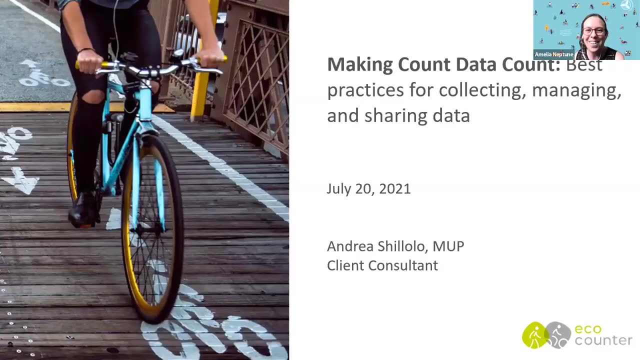 found exploring Montreal and surrounding regions by foot and by bike. So, Andrea, you can go ahead and share your screen And we're looking forward to hearing the important lessons from EcoCounter. Thanks a lot, All right. Thank you so much, Amelia. I'm assuming everyone can see. 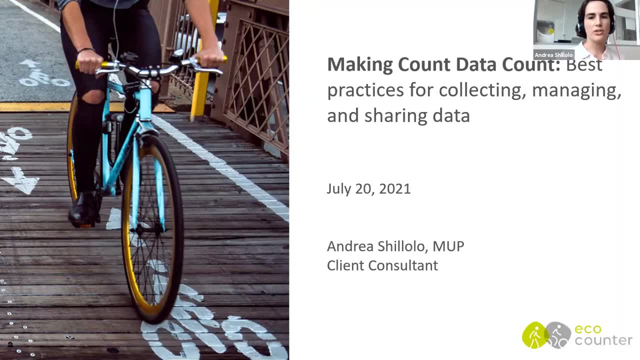 my slide presentation. I'd also like to thank Mike and Amanda for those great presentations. I feel like you just gave some kind of on the ground examples of everything I'm going to discuss. So a variation on a theme: making count, data count. I'm going to talk about actionable. 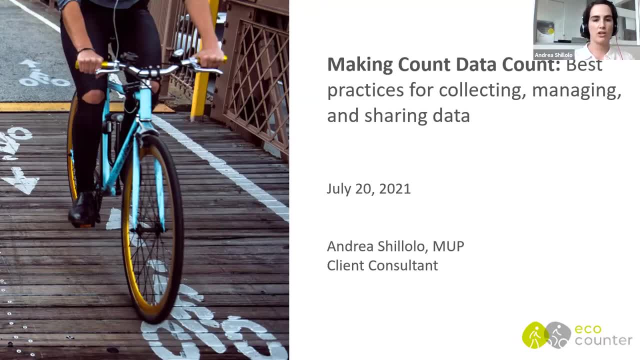 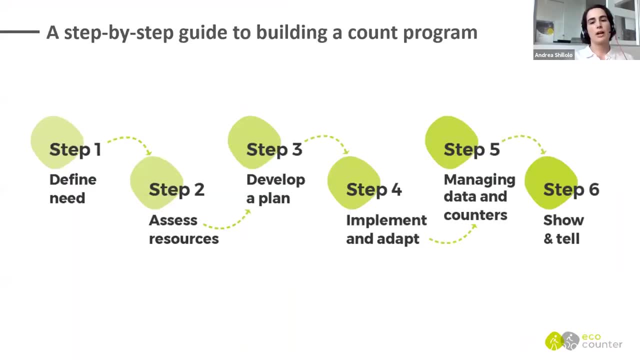 best practices for collecting, managing and sharing your data. So I work with EcoCounter, where we help our clients build bike programs every step of the way. So count programs have a variety of steps. I'm going to be focusing more on the last three pictured here. So implementation and adapting. 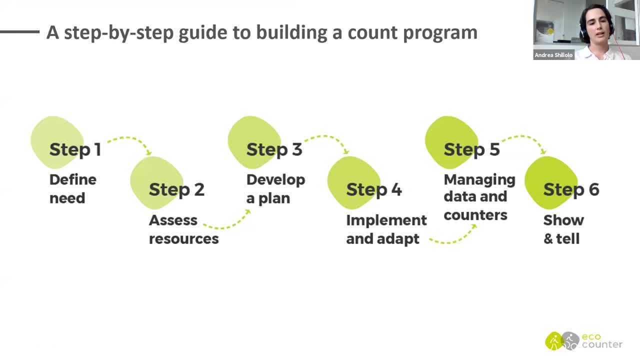 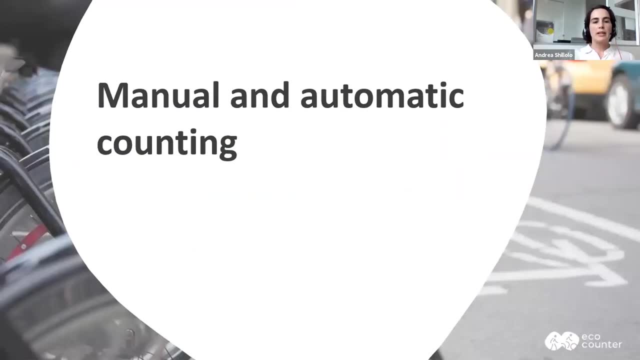 managing your counters and your data and then, finally, that show and tell piece, the communicating your data. So I'm going to talk a little bit about manual and automatic counting, And I think we just had that- Two really great examples of how those are two valid ways of collecting bike count data. 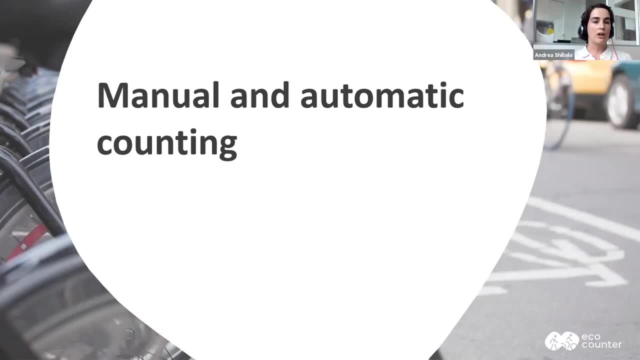 EcoCounter is a world leader in manufacturing automatic counters for bicycles and pedestrians, as well as software to analyze that data, But manual counting is also extremely important and a valid way of collecting data. I'm not going to focus too much on the implementation of 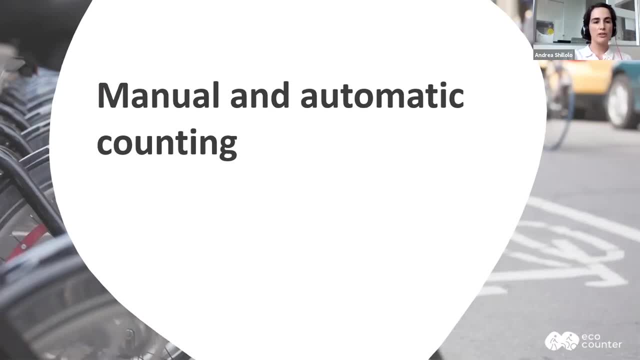 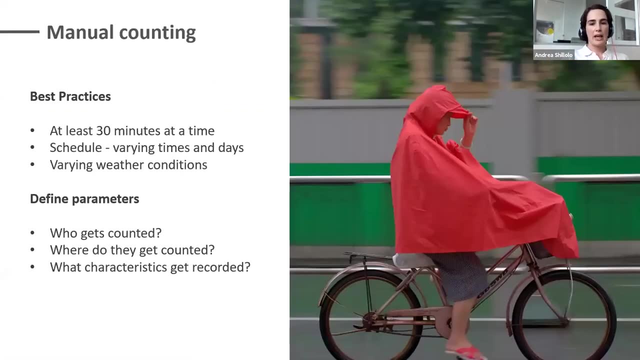 of count projects, but I will just go over each briefly because it will kind of feed into what I talk about later on in the presentation. So manual counting, It can be a great way to collect data. It can also be a great way to begin a count program. Sometimes it is a way to 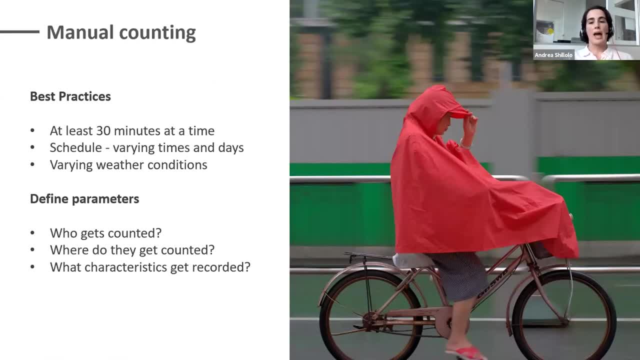 justify investing in automatic counters. This has already been really well demonstrated or described, but I think it's a really good way to start. So I'm going to talk a little bit about manual counting. So manual counting is a really good way to start, So you can start by doing a manual count. 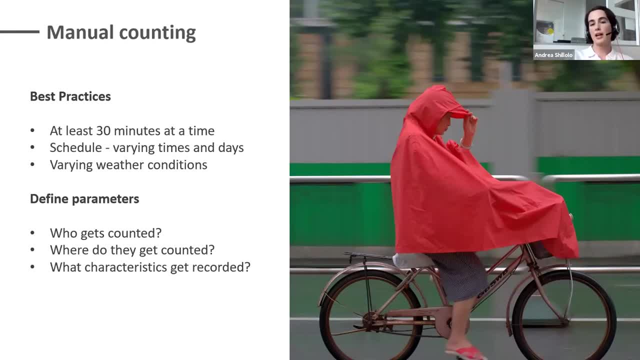 by Mike. When you're doing manual counting, you really want to make sure that you're doing it at the right times and planning a schedule. So you want to do it for at least 30 minutes at a time, if not longer, And you want to schedule it for varying times, So times of day, you know. 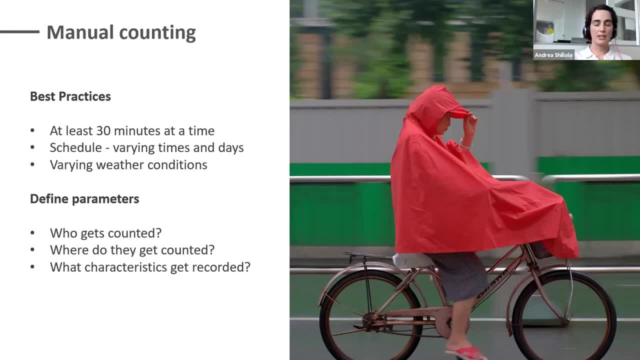 rush hour is not going to be the same as nighttime traffic. you really want to do a variety of different times to collect data that represents different traffic. On that note, varying weather conditions is also extremely important. I'm sure that all of you know that non-motorized traffic is just much more sensitive to different weather conditions. 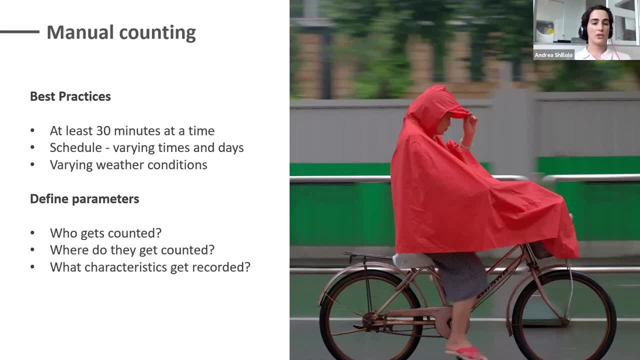 be that summer versus winter or a rainy day versus a sunny day. And when you're doing manual counts, you also want to define your parameters. For example, who gets counted? Are you going to count someone on a scooter as a cyclist, or a pedestrian, someone with a stroller? How are they actually? 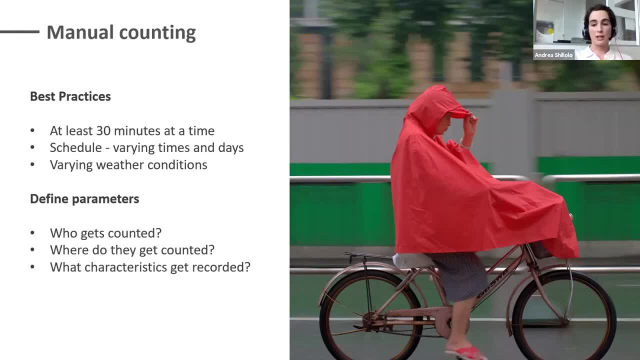 categorized. Where do they get counted? Sometimes you might be choosing, you know, a kind of complicated intersection, because that's where you want to, you know, learn about bike safety. So you might want to have an imaginary cordon count line. 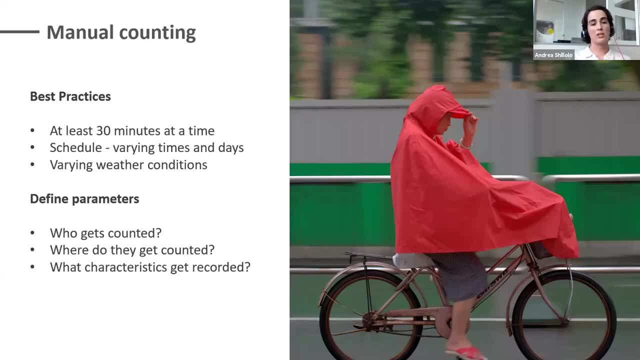 Or an actual physical barrier, But just defining those parameters so that everyone who counts is counting people along those same criteria. Also, what characteristics get recorded. A really valuable part of manual counting is that people can take note of someone's demographic characteristics, So things like age or gender. 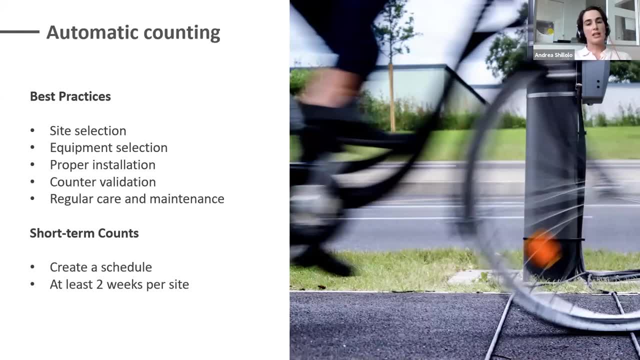 Automatic counting is kind of a different ballpark And, like a man, I think is a really important part of manual counting And so, as Amanda mentioned, there are some tips and tricks to keep in mind. You really want to be careful about site selection. 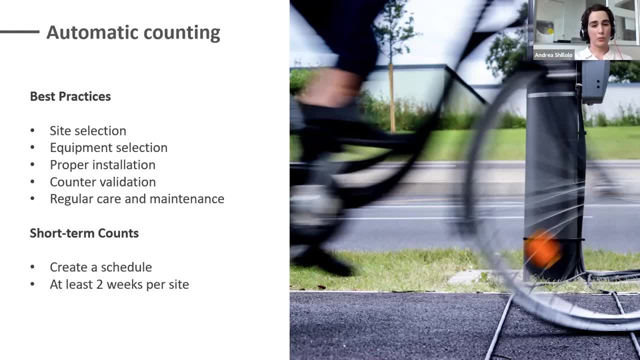 First of all, it needs to be a valuable site in terms of the data you're collecting, But also you want to make sure that the counter is actually going to work at that site And, like she mentioned, at EcoCounter. we're here to help you make those decisions. You want to make sure that you select. 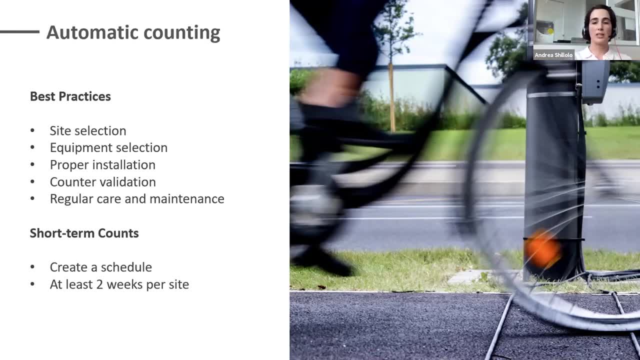 the right equipment. So things like range of the sensors for the width of your path is really important, And are you collecting the right data for the user groups? Do you want a bike counter? Do you want a pedestrian counter? Do you want one that can do both? I'll talk a little bit about counter. 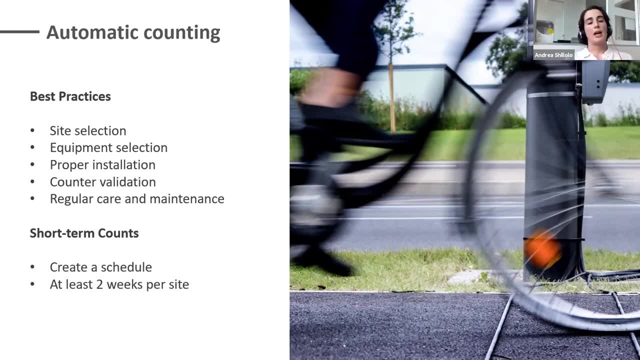 validation later, as well as care and maintenance And then kind of like manual counts. if you're using a counter you can move around, an automatic counter that you can move around. you're also going to want to create a schedule And you want to have it in place at least two weeks at a time. 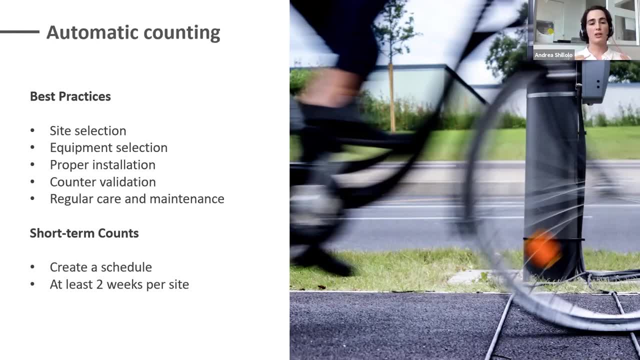 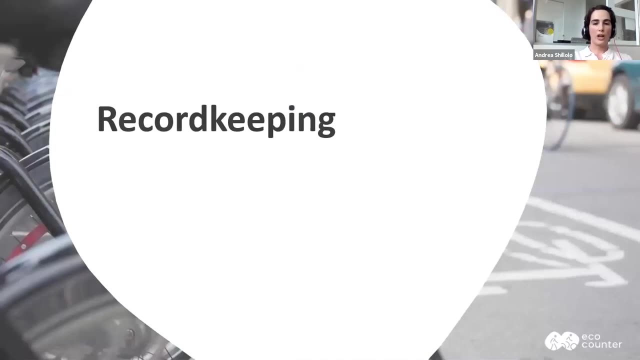 Same idea as before. you want to be able to get a good representation of weather and how it might impact traffic. So if you were to put a counter in place for two weeks, you're more likely to get a variation in weather Record keeping. Okay, so count data is really all about trends over time. 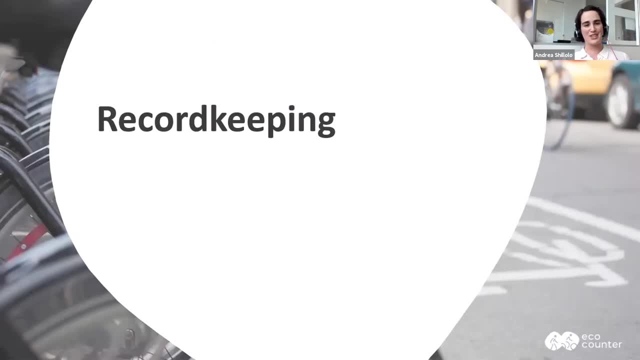 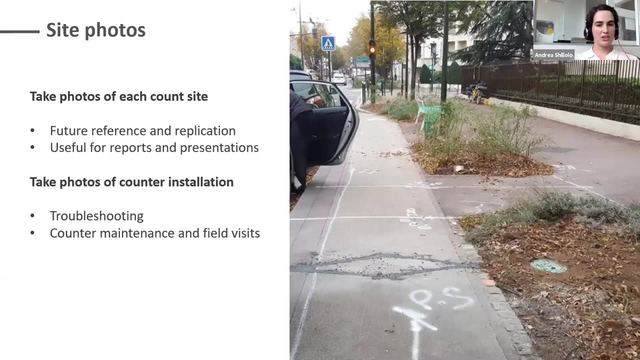 and I highly recommend you do your future self a favor and keep track of all of your work, And you can do this in a number of different ways. I recommend all of them. So site photos: This probably seems very basic, but it's very important. You can use them for future reference. 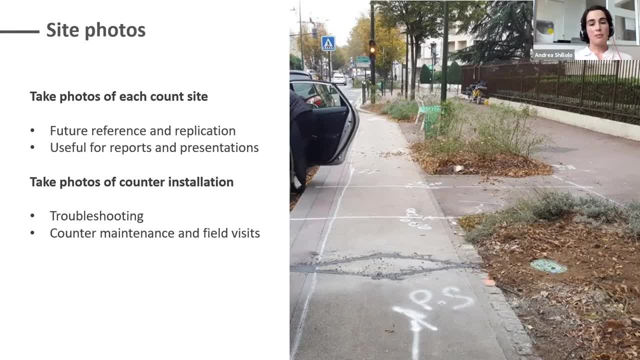 as well as replication, You can use them in reports and presentations And also you might be able to use them when you're troubleshooting a physical counter or doing field visits and maintenance. You can actually see in this photo that there is a zelt counter. This is a cyclist counter. 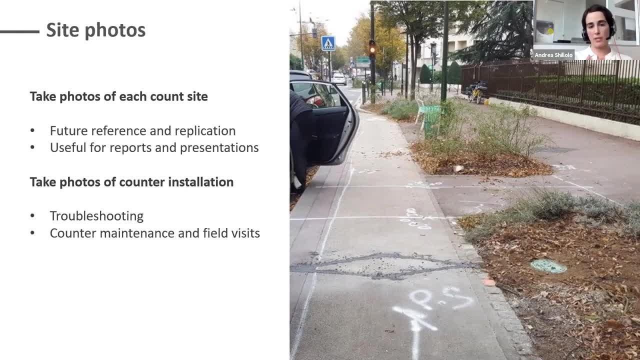 with a manhole. The little green disc is the top of a manhole which, after it's there for a couple of years, can easily be covered in grass. It's just really helpful to go to the site and have an idea where you're going if you're switching out a battery or something like that. Another. 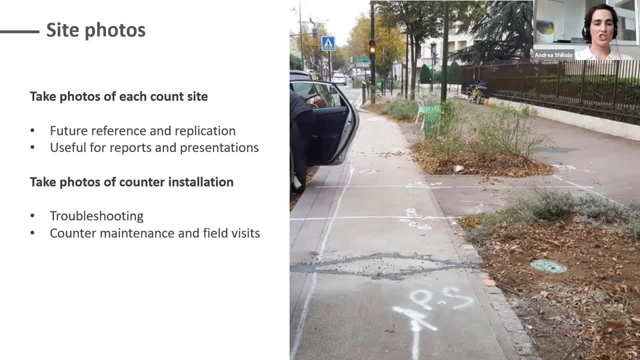 thing in this photo is some spray painted lines. I'd also mention that you might want to draw some diagrams, Especially if you're doing a manual count and using an imaginary cordon count line. it's a way to keep track of that. So if you were to go and replicate the counts people know, 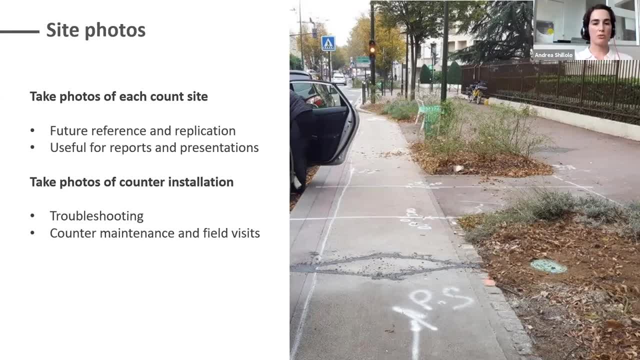 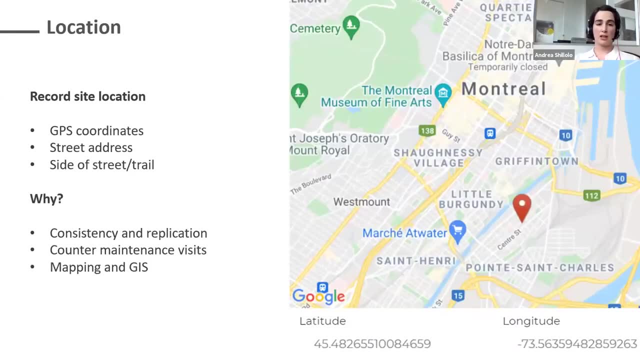 exactly what threshold someone has to pass in order to make a tick and count someone. Recording the location also very important. There's a lot of different ways to record the location. This image here is taken from Ecovisio, EcoCounter's online software. You could use lat-long coordinates. You can drop a pin on the. 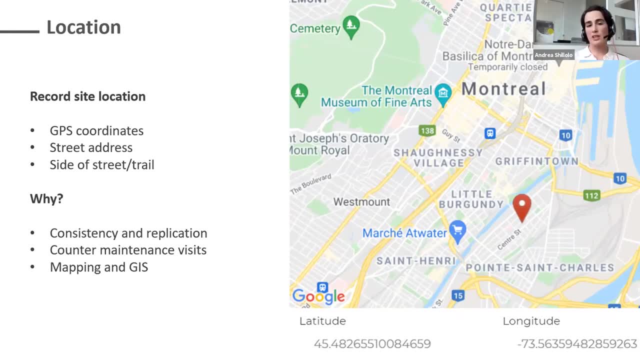 map or just put an address into Google. If you're recording this yourself, you can do similar things. You might also want to make note of what side of the street you're on. So this is really important again for that consistency and replication piece. Also: counter maintenance visits: New staff- new. 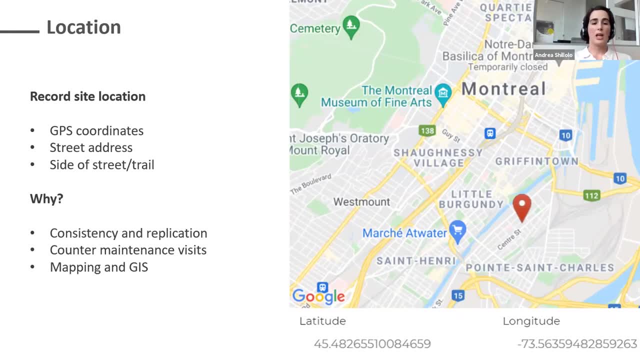 volunteers will want to know where they need to go. This is really important again for that consistency and replication piece. Also, counter maintenance visits, New staff, new volunteers will want to know where they need to go. Also, you can combine this data like GPS coordinate data, for example. 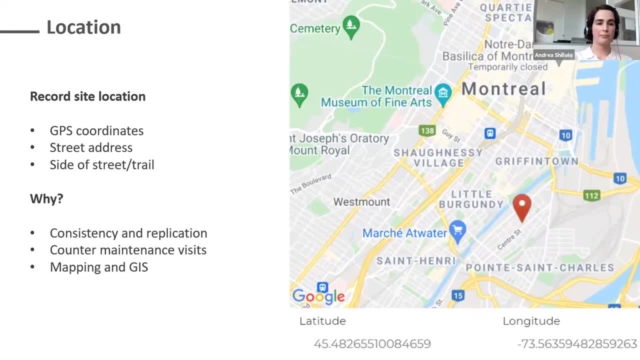 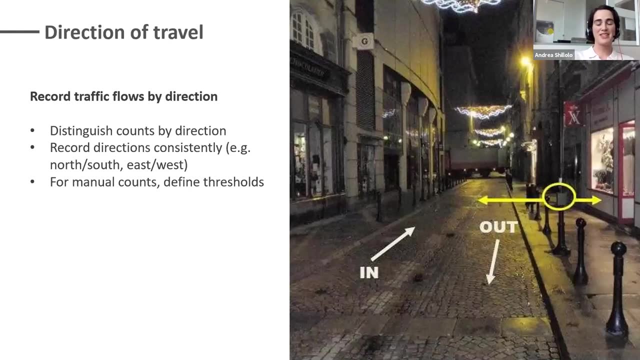 with GIS software and use it for mapping Direction of travel. Okay, so this has already been mentioned a couple of times as an important indicator of your bike traffic trends. You can imagine a path that's heading to a downtown might be busier in one direction. 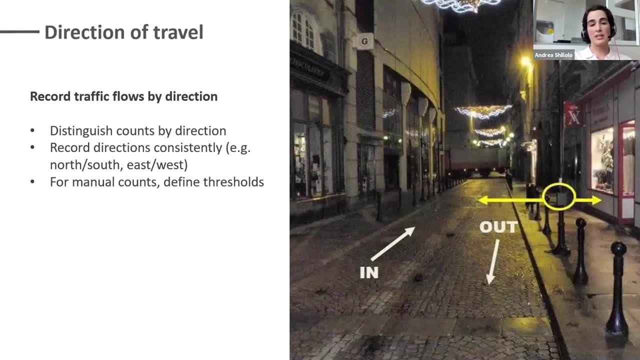 during rush hour in the morning than it is in the evening. It's also a really good way of capturing wrong-way riders, as Amanda mentioned. So you want to keep track of directions and you want to do that consistently, So you want to label your directions. north, south, east, west is a really 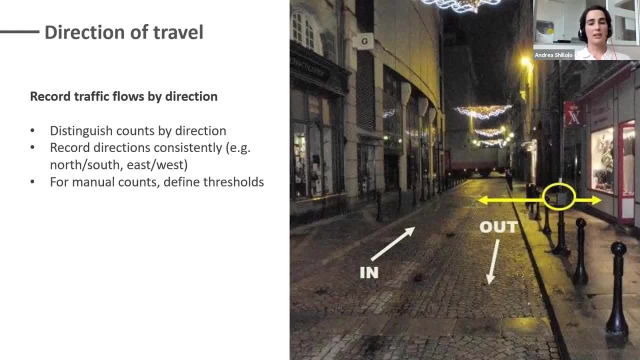 obvious way If you want to say something like toward downtown, away from downtown, as long as it's clear and can be later referred back to and understood. that's the key. And then again, with manual counts, you want to be able to define the actual thresholds that people have to pass at. 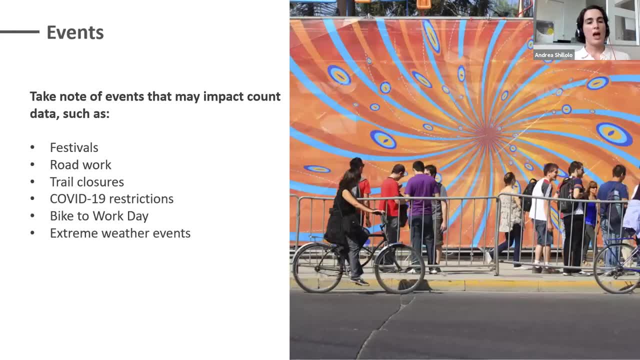 in order to be counted Events. This is another really important thing to keep track of- that's already been mentioned- Any event that might have an impact on count data, so a festival, road Roadwork closures, extreme weather events. also COVID-19 restrictions, which has been brought up. 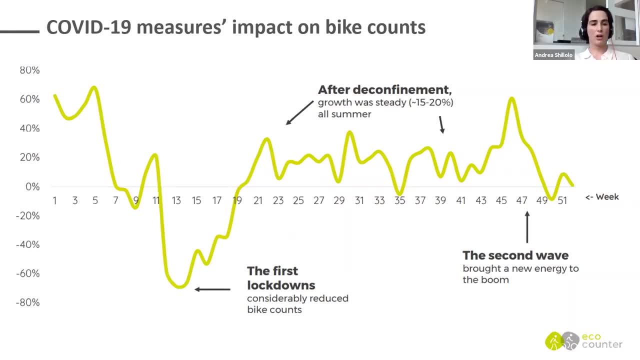 This is an example. Actually, I stole this slide from a colleague of mine. in Europe, This is obviously an event that has had global impacts And it shows the way that COVID-19 restrictions, like the lockdowns and then deconfinement, have affected bicycle traffic. 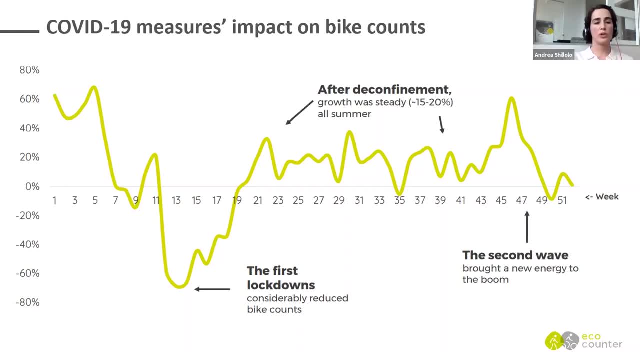 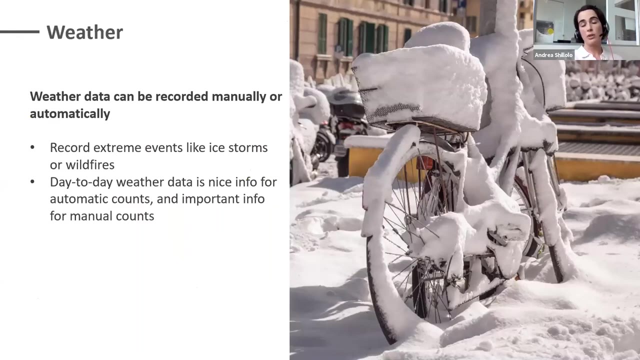 I believe this was in Spain, France and Germany. But you can see some real steep declines and then some more spikes once people were deconfined Weather. So weather can be recorded manually. I say automatically, because we do at EcoCounter offer weather as an added service. 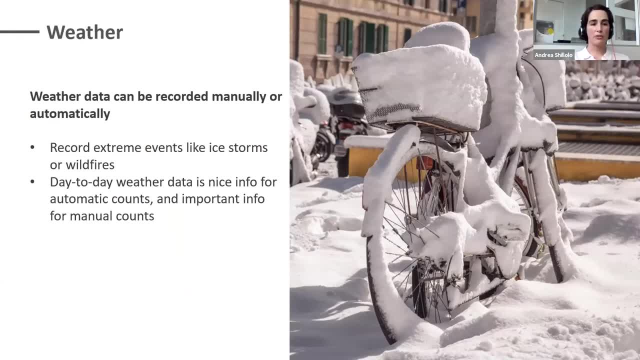 You can actually have satellite weather information that we lay on top of your count data. Like I said, non-motorized traffic is really sensitive to different weather conditions. You also have extreme weather events, like an ice storm or wildfire, that you would want to record. 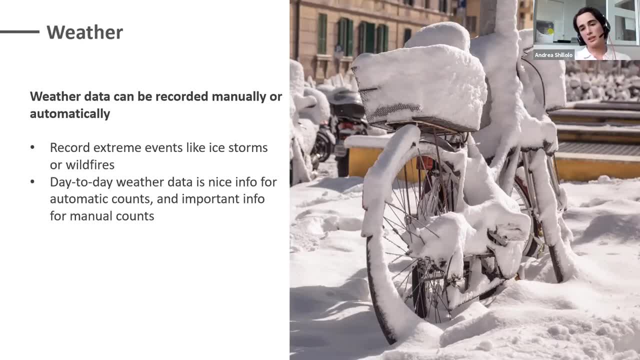 So the day-to-day weather That we can provide via satellite is kind of a nice-to-have when you have automatic counts, But it's really important for those manual counts. Like I said, if you go out on you know only rainy days, you're not going to see a full picture of bike traffic. 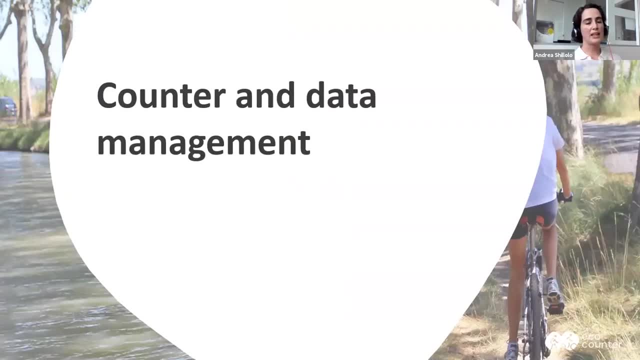 Okay, so counter and data management. I like to think of count programs like a garden. It's something that you continually need to tend to. You can, you know, plant your seeds, just like you can install your counters, But if you're not checking on things and tending to things, things don't grow as well as they could. 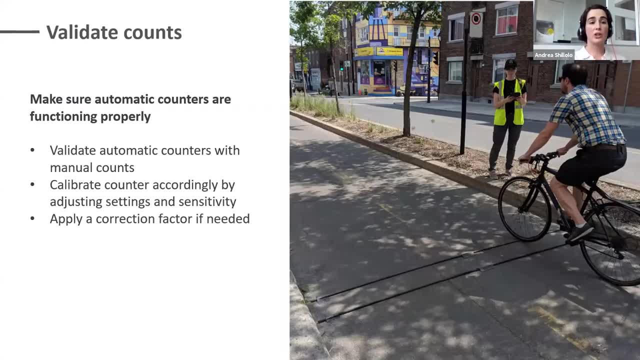 As has already been mentioned, this includes validating your counts. If you're using automatic counters, you want to make sure that each time you install them at a new site, that you're making sure that it's working, That they're working properly. 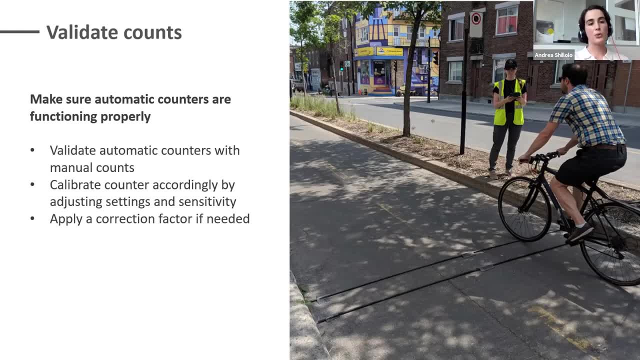 Each site is unique and has different traffic, So you want to calibrate the counter, adjust the settings and sensitivity, And then you can also apply a correction factor if needed. I won't get too detailed in data corrections, but it is a possibility. 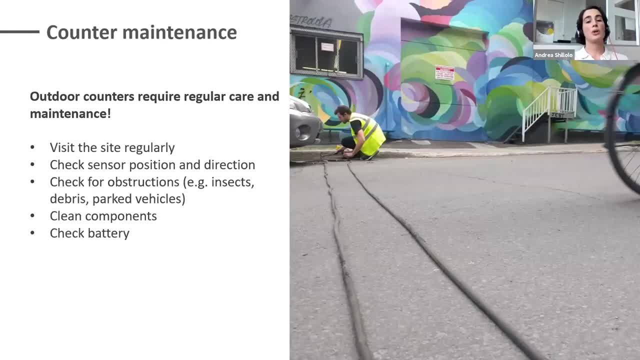 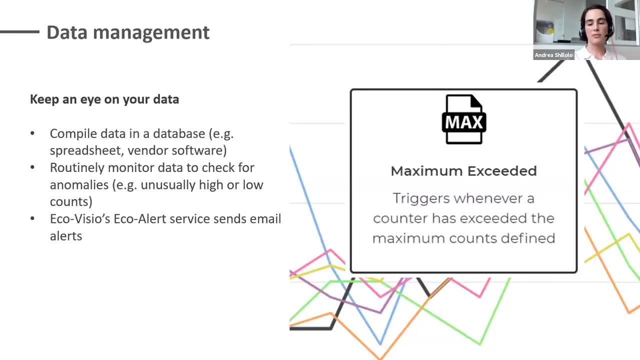 Also counter maintenance. So our counters are designed for outdoor use. They have a long battery battery life, but you don't know what's going to happen to them in the wild. They really need regular care and maintenance. The counter- oops, the counter that's pictured here is a tube counter. 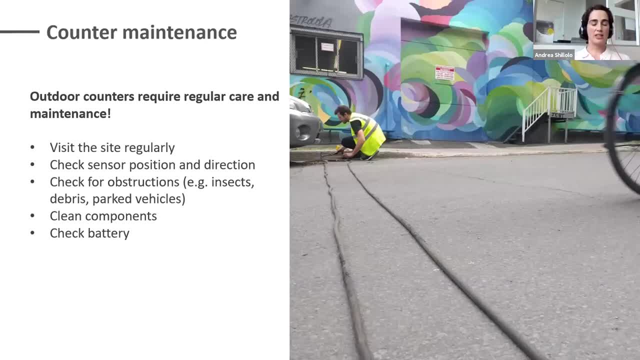 which Amanda mentioned, needs to be taut. It needs to be stretched at a certain tautness in order to function properly. And it's just on top of the ground surface So it can easily be moved around by passing vehicles if you're not careful. So you want to visit the site regularly. You want 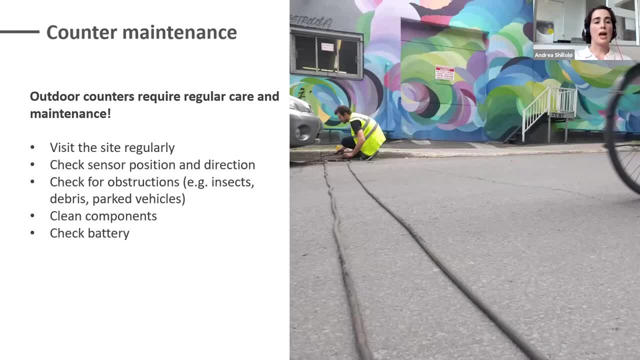 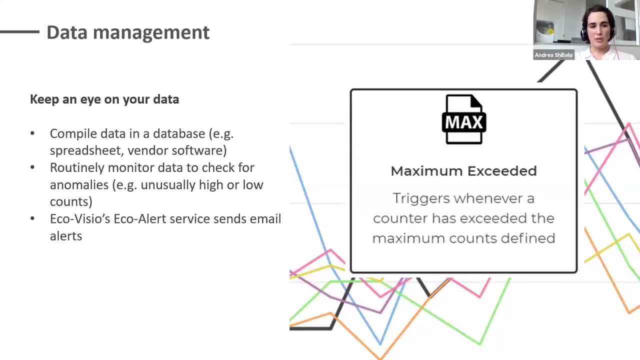 to make sure that the sensors are positioned where they're supposed to be positioned, Check for any obstructions, insects, like Amanda mentioned. Clean the components, Make sure the lenses are clean And do things like check on the battery, Data management, Keeping an eye. 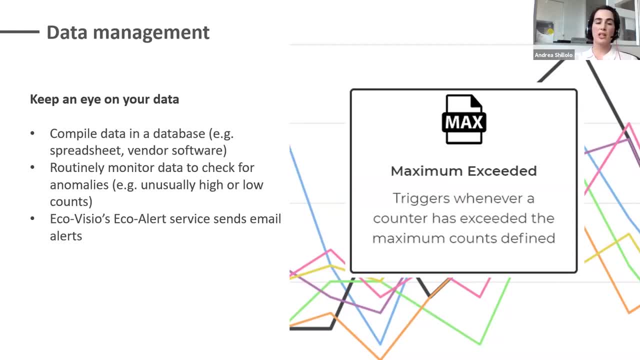 on your data. So, first of all, you want to keep all of your data in one place. whether you're using a computer or a laptop, You want to keep all of your data in one place, whether you're using a computer or a laptop. You want to keep all of your data in one place, whether 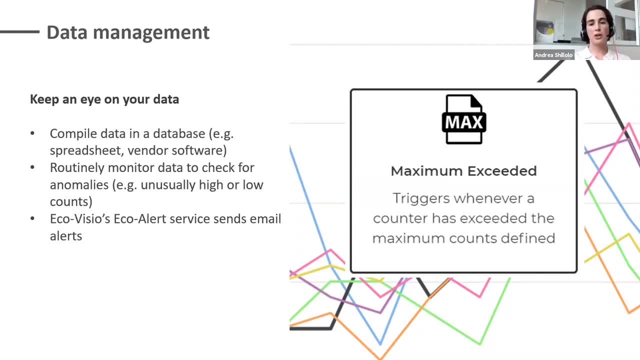 you're doing manual counts or automatic. You can keep all of your data in a spreadsheet or in the software the vendor provides And you want to check for any anomalies, Things like unusually high or low counts that can be caused by an insect on the lens or something like. 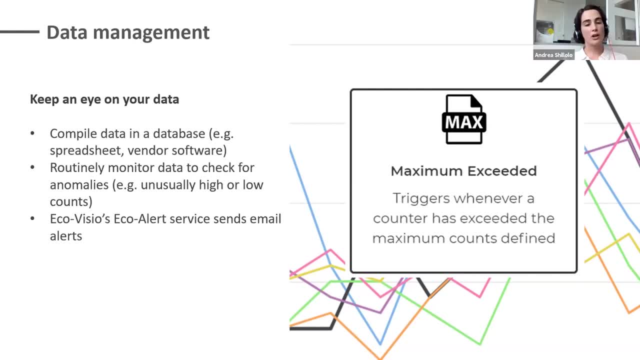 electromagnetic interference, a car parked in front of a sensor. You want to routinely monitor and check your data for these anomalies, And the image here is actually an eco alert, which is a feature of our software, Ecovisio, that will send you an alert by email whenever we detect any unusual data that strays from the 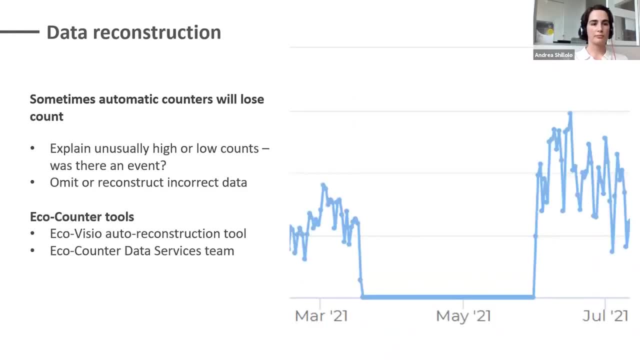 norm of your usual counts- Data reconstruction. So sometimes you will be missing counts for the norm of your usual counts: Data reconstruction. So sometimes you will be missing counts for the 하게 for natural and unidentified incidents. EXO, Biomania viruls. What is a через or 위? 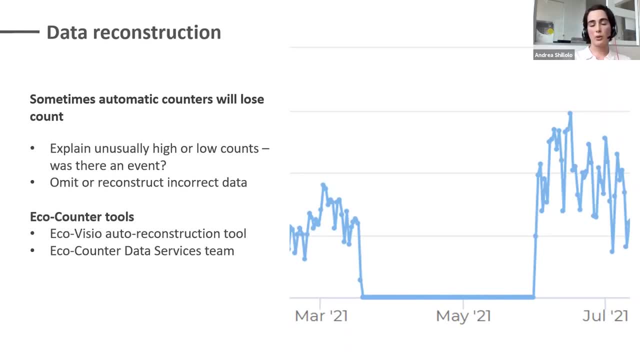 First of all, you want to determine the cause. Maybe there was an event that you'd recorded that would explain why suddenly no one's on a path or many people are on a path. But if it's not caused by that type of event or you know there's some other occurrence, You can either 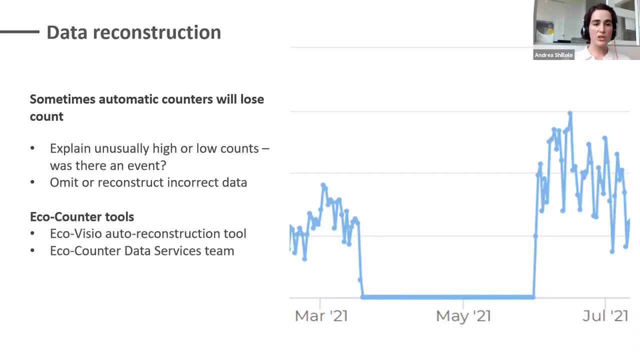 omit or reconstruct that data. So EcoCounter has some tools to help you do that, And EcoVisio, our online software. we can help with the same thing. But if you want to overcome the shield and cause any danger, You can either filter a sample as to why the event may have appeared Or, if you 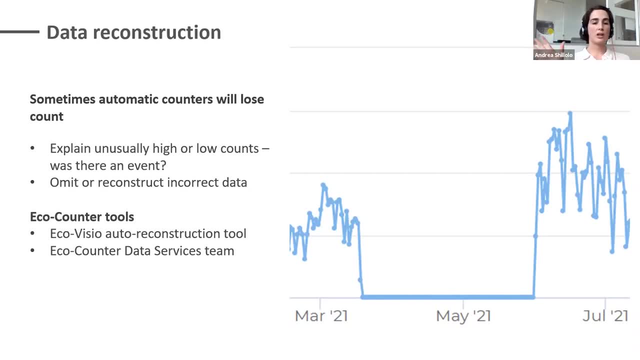 glitter in the media for a change. As I mentioned before, you can filter by having needles on the see suffered auto reconstruction tool, where it will use data from the previous weeks to fill that gap. And then we also have our data services team who have been helping Mike and Amanda with their data. 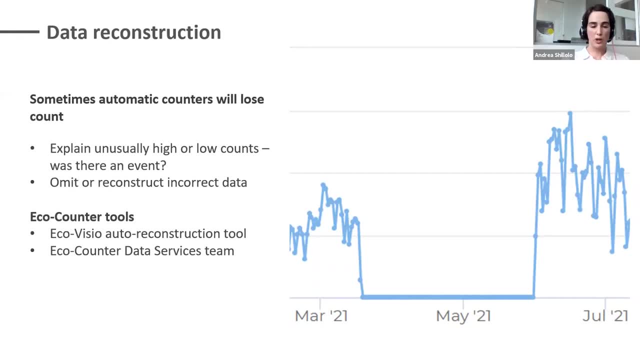 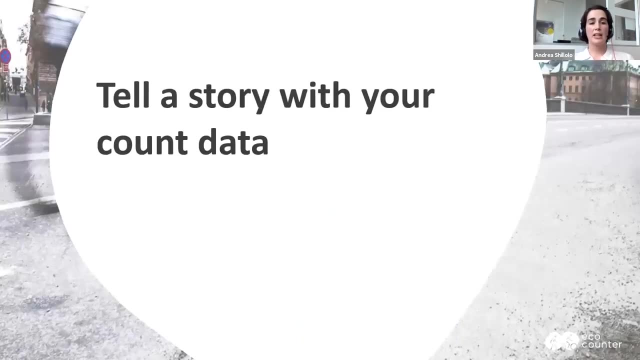 So there are options, but just something to keep in mind. You do want to keep an eye on your data to prevent this from happening where possible And, finally, you want to be able to tell a story with your count data as has been shared already. Data is really more valuable when it's shared with. 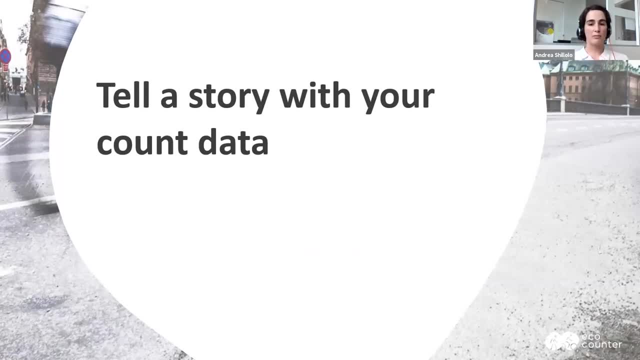 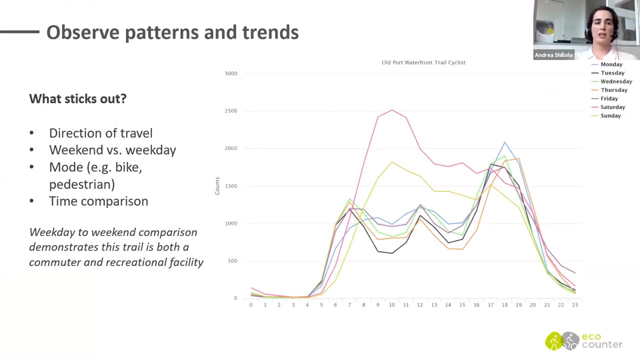 others and giving context to your data can make information more meaningful to audiences. So there are some different ways to do that. Observing patterns and trends is kind of the first step. I really like this graph because I think it says a lot about the nature of a bike path here in. 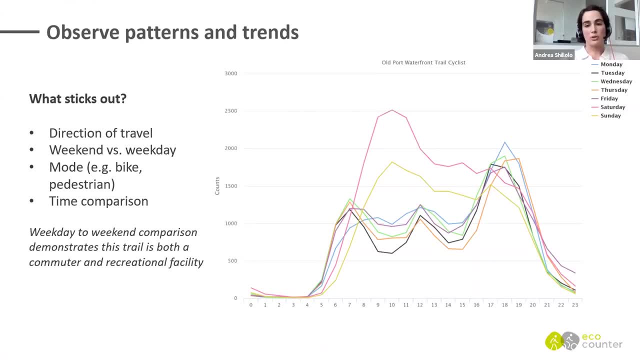 Montreal With, you know, just a very simple line graph. So bike volumes for each day of the week are plotted against hours of the day on the x-axis, And then the top pink and yellow lines represent Saturday and Sunday, And then the rest of the colored lines below are the weekdays. 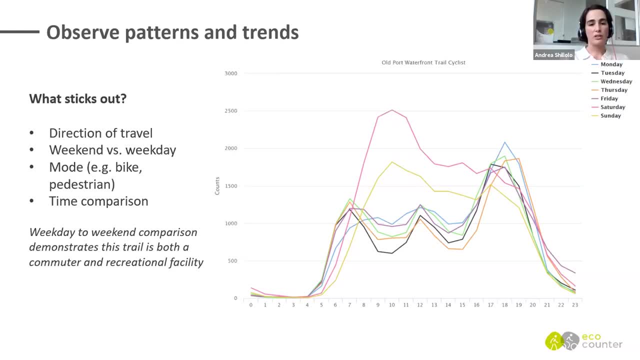 And just by looking at the spikes in this graph you can see that this is a very popular recreational trail on the weekends as well as a commuter trail. You see those spikes during rush hour and lunch during the week and then kind of a midday spike. 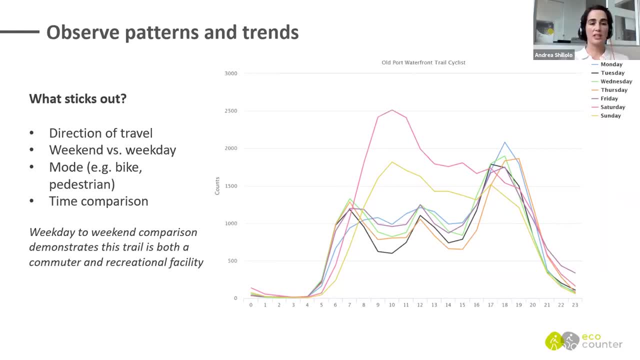 on the weekend. So just look for things that stick out, Things like direction of travel, bikes versus pedestrians- and then doing a time comparison such as this can be a good way to figure out what trends and patterns are emerging, Highlighting key figures Sometimes. 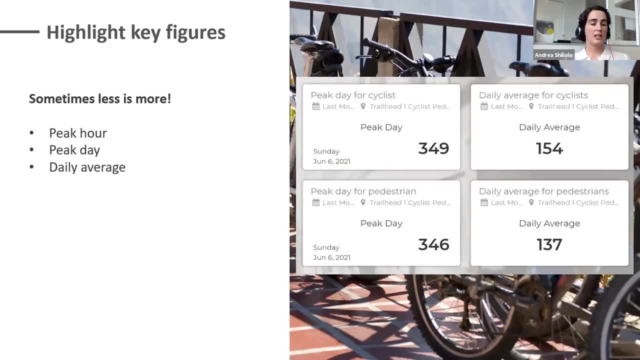 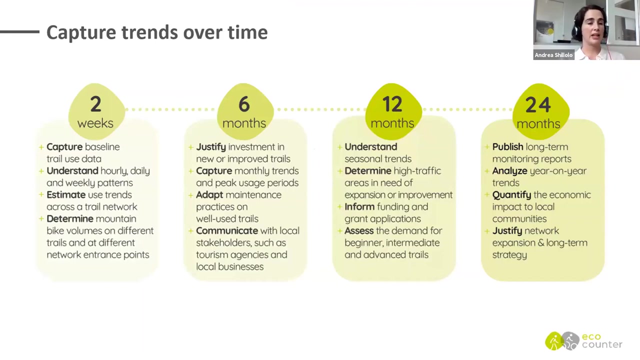 simple figures can be very powerful. This is taken directly from our online software once again, And it's just showing peak days and average for both cyclists and pedestrians. Really simple, but also powerful, Also capturing trends over time. So the longer that you have been collecting, count data. 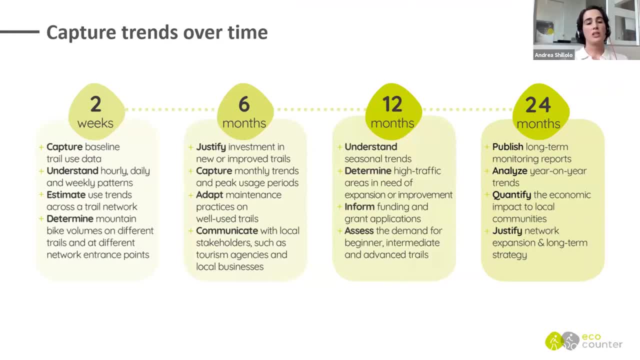 the more that you're able to do with it. So this demonstrates, you know, at two weeks, your ability to get baseline data and understand daily and weekly and hourly data. By the time you get to six months, you can start doing things like justifying investments and improvements. 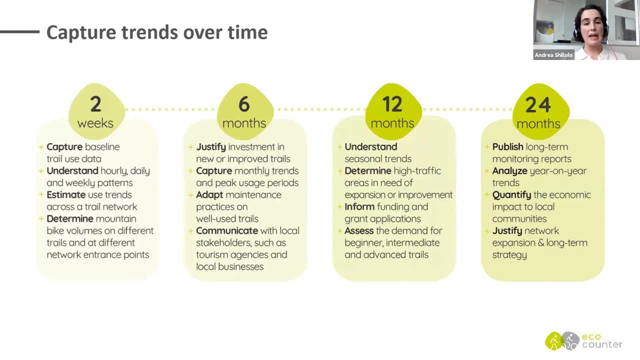 capturing monthly trends, maybe starting to adapt maintenance to your facilities and to the traffic on those facilities. Around one year you start to understand seasonal trends. You might be able to start informing grant and funding applications And then, at two years, you have yearly trends. 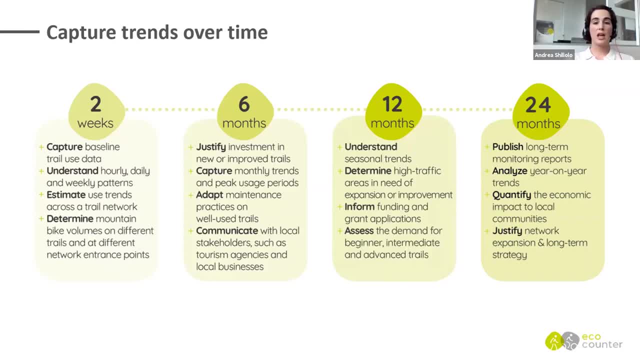 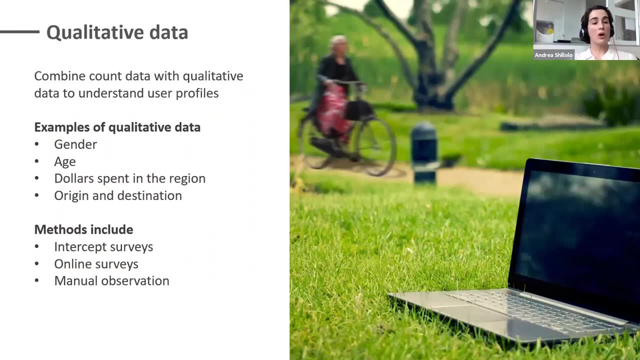 You can publish long-term reports and you can also justify expansion to your networks. Also, qualitative data, And this was brought up earlier. It can be really interesting to combine your automatic or manual count data, raw count data, with data, So your counts can provide a ground truth from which you can extrapolate the proportion of 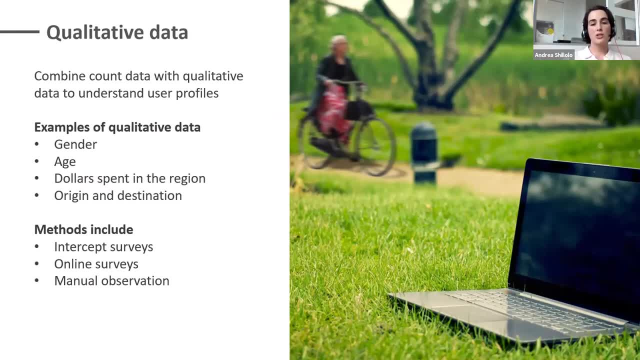 users who fit a certain profile. So you might want to collect data on things such as gender, age, origin, destination, And you can do this through things like intercept surveys, where you'd actually stop people. Maybe while you're doing your manual counts, you can have an online. 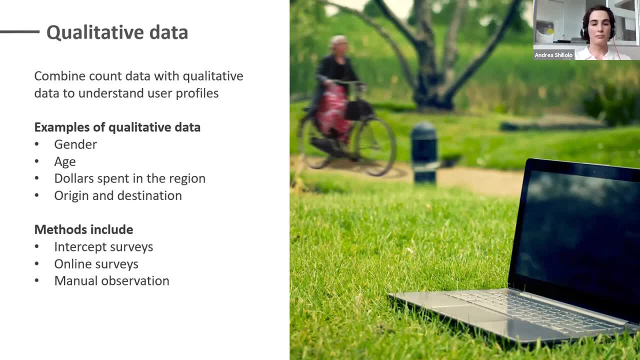 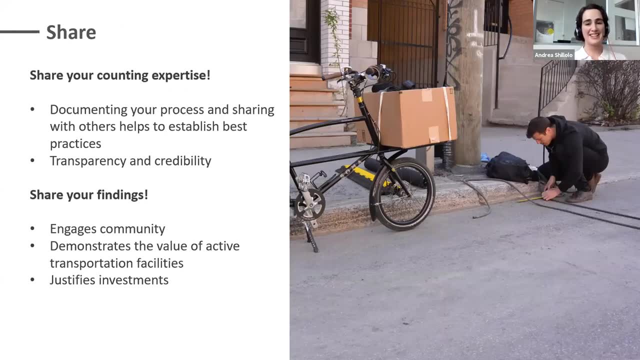 survey and just manual observation, And then, finally, you really need to share that data. So all of the time that you spend on your count program and in the field and analyzing your data is really valuable knowledge and expertise. Think of all that you've learned through your 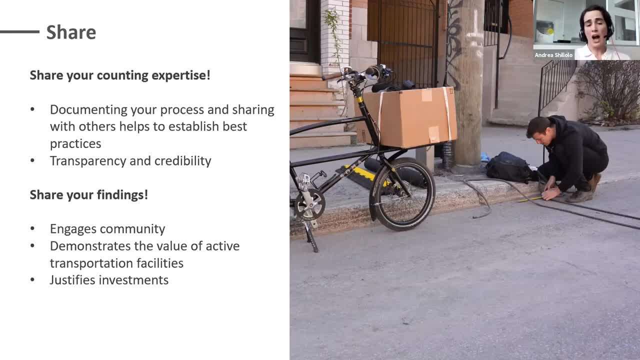 process and how much you could share with others. It also helps to establish best practices if you publish your findings, as well as leads to transparency and credibility. If you share your process, it's just easier for people to understand how you arrived at the counts that you did And then count data can also be used to engage others. 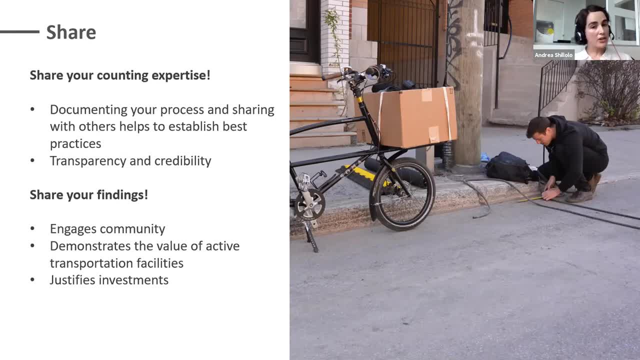 So it can engage the community, It can demonstrate value of your facility And it can also be used as a way of sharing your data. So if you have any questions, feel free to reach out to me And I'll be happy to answer any questions that you may have. 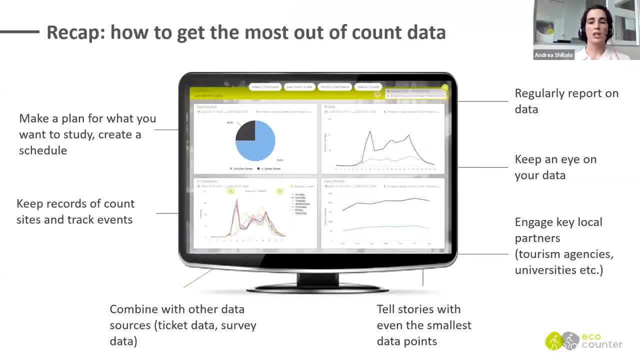 So, just to recap, make a schedule, keep records of your count sites, records of noteworthy events, keep an eye on your counters, keep an eye on your data, observe any patterns and trends that emerge and then try to tell a story with that data that can really engage others. The image here is: 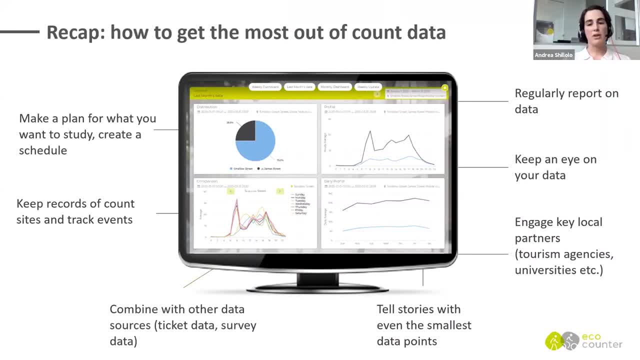 an image of EcoVisio, our online software that makes it really easy to kind of keep track of all of these different steps. But you can definitely come up with a system on your own that's systematic and methodological and will just help things later on. 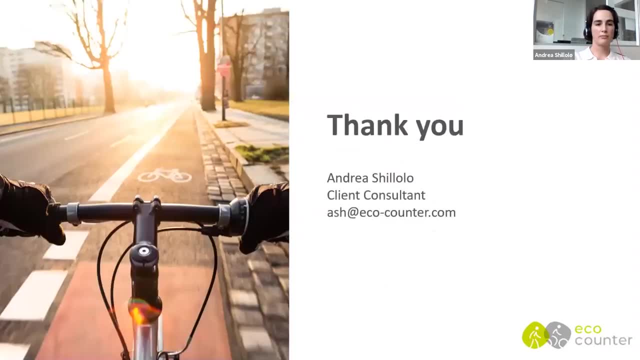 and not let any of your work go to waste. And that's it for me. Thank you so much. Thanks so much, Andrea, And thanks to everyone who's still on. We're actually exactly at time And I don't want to stop the conversation if folks still do have questions. 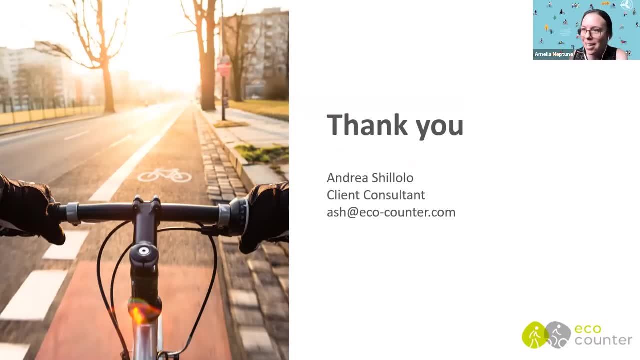 But in respect of everyone's time, feel free to hop off if you- and I know people have been. but if you need to, if you need to leave, feel free. And I want to thank all of our speakers not only for presenting but for typing answers into the chat throughout. 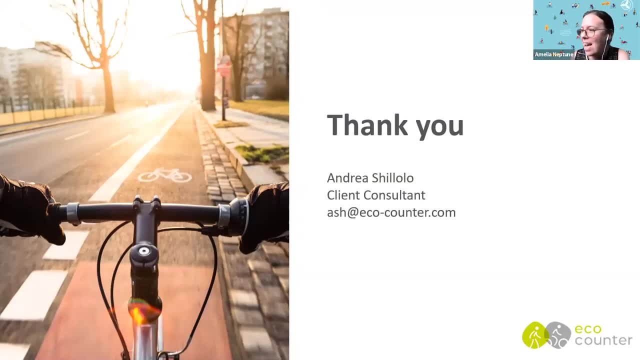 So I feel like we've actually answered most of these questions, So if anybody has any last burning questions, feel free to type them in the chat quickly before We end, And what I'll do is I'll also download all of these questions and make sure that we answer them in the blog post that we'll be doing next month as a follow up. 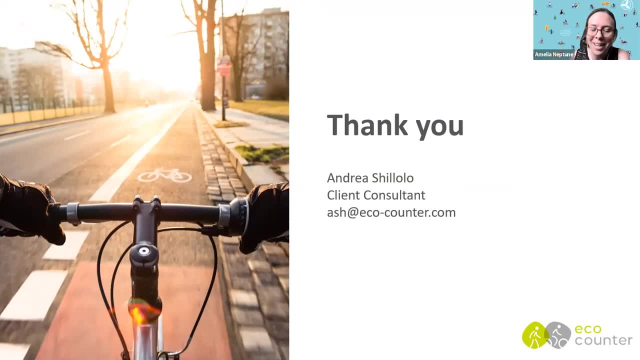 We'll also be sharing out the recording and the slides much sooner, But expect a lot more information about the results of the competition and some really exciting data visualizations that EcoCounter will be producing for our award winners. So thank you again to everyone for joining today. 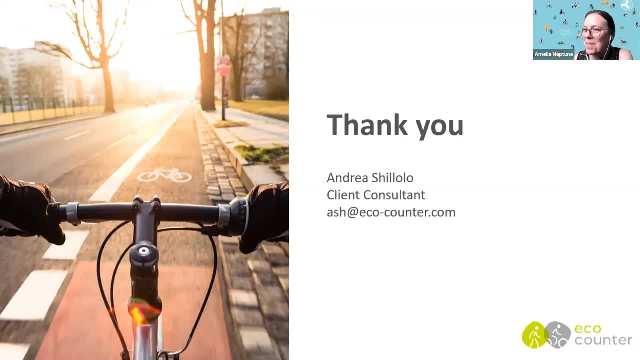 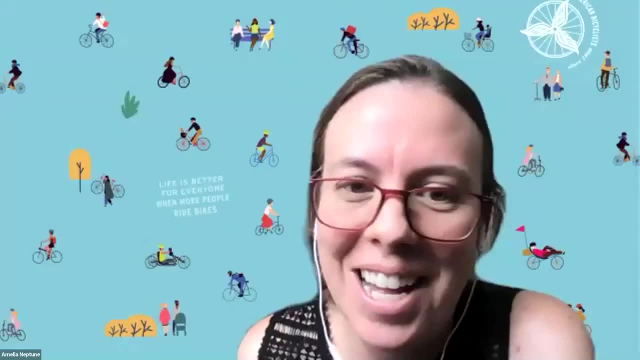 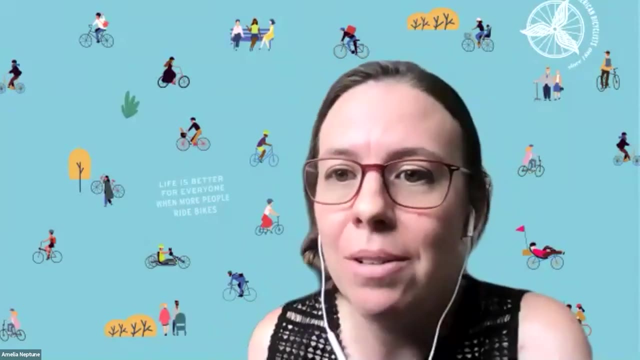 I'm not seeing any new questions So I'll close this out in just a minute, But again really appreciate our presenters and EcoCounter for all your work and support of the League and the Bicycle Friendly America program. And if other folks have questions, please do feel free to reach out to me at the League, Amelia at bikeleagueorg, or to Matt or Andrea at EcoCounter. 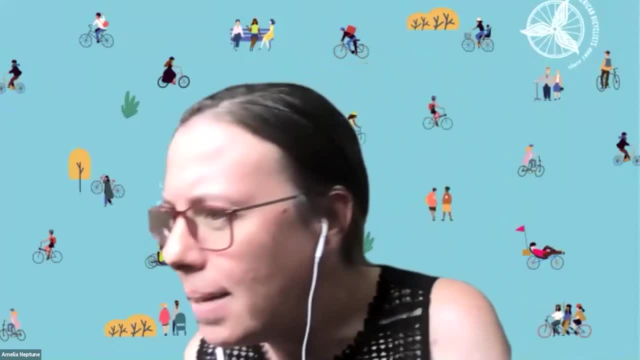 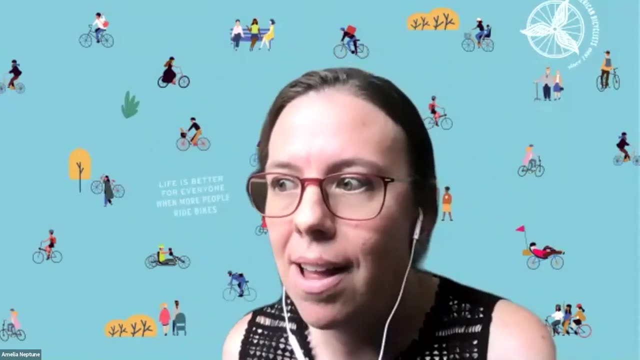 And we look forward to working with all of you. And the last couple of questions that got in. I don't know if any of our speakers want to answer those Quickly or we can handle those offline. if not, We've got one.